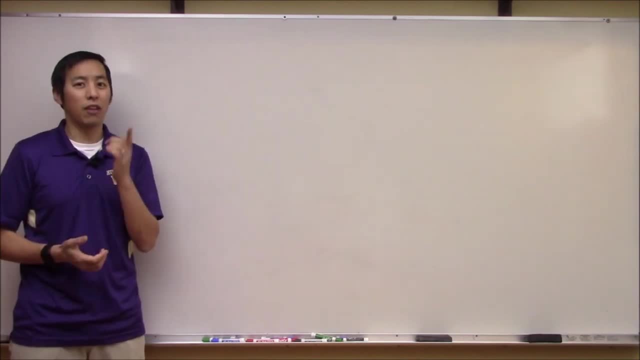 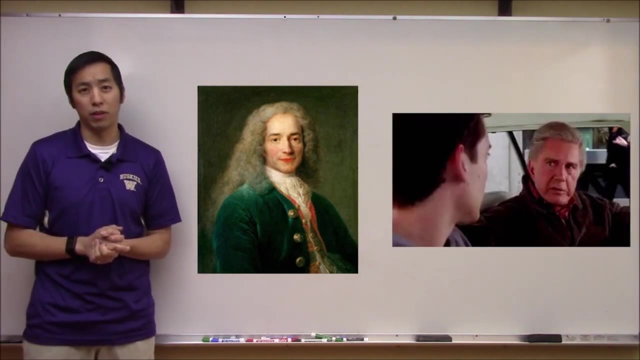 what's the price we pay for this amazing ability? As Voltaire, and perhaps more recently, Spider-Man's uncle Ben Parker, once said, with great power comes great responsibility. Therefore, today I'd like to look to see if there are any practical implementation issues that might arise when you try. 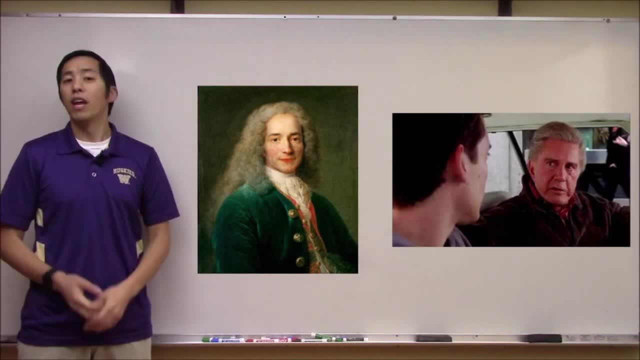 to use a full-state feedback controller on a real system. So if that sounds like fun, why don't we jump over to the whiteboard and take a look at some of the questions that have been asked? So if that sounds like fun, why don't we jump over to the whiteboard and take a look at some of the questions that have been asked? So if that sounds like fun, why don't we jump over to the whiteboard? 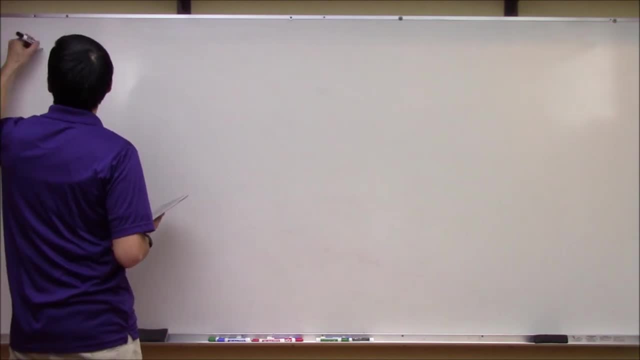 and take a look at some of the questions that have been asked. So if that sounds like fun, why don't we jump over to the whiteboard and get started? Okay, so to refresh your memory, the idea with full-state feedback control. 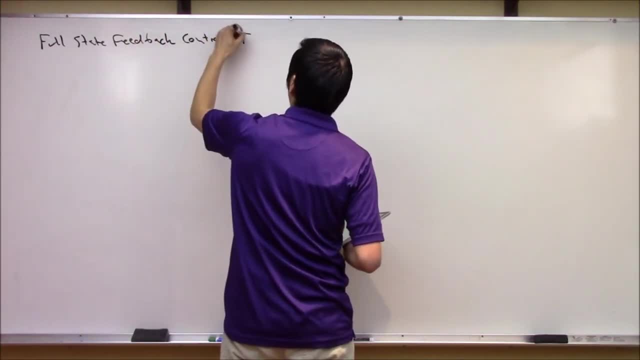 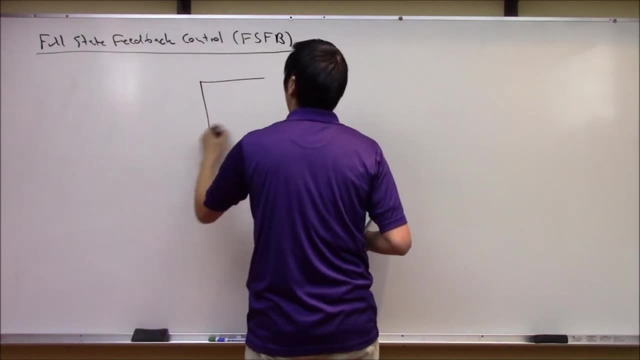 and in fact this is going to get tedious writing this, so let's just abbreviate this as FSFB- full-state feedback control here. So the idea again here was that you had some plant model here which was typically modeled as a linear state space model. x, dot is equal to ax plus bu And y in. 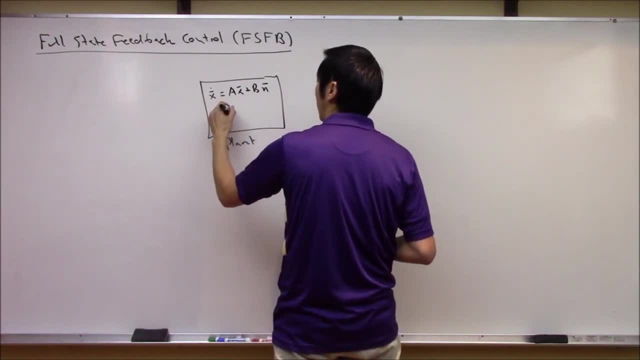 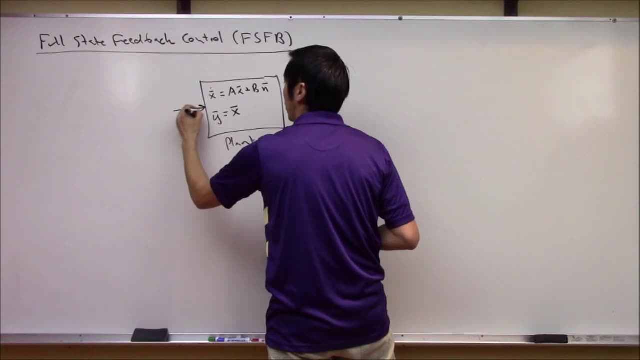 this case is actually equal to the entire state vector here. So in this case, your C matrix with an identity and your D matrix was zero. So in this picture, what goes on here is again, you have a control vector of u coming in and now you have an output which is the entire state here. 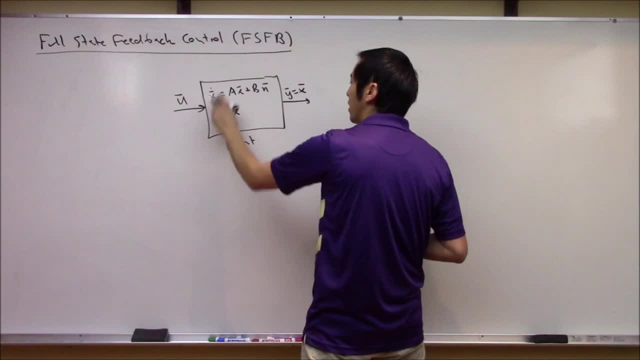 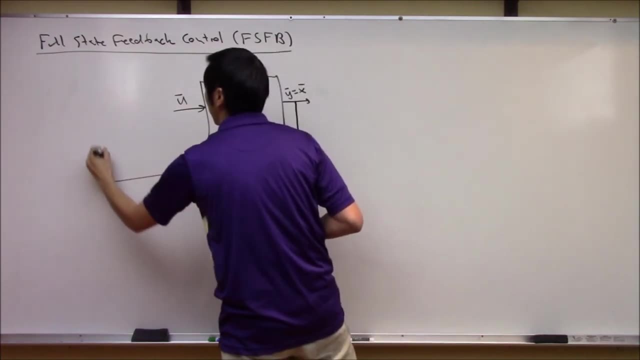 And now what we were going to do here is that we maybe didn't like where the open loop eigenvalues of this plant were, So we were going to change this by feeding back the state vector and running it through a controller here, And in this case we are going to use a full-state feedback controller. 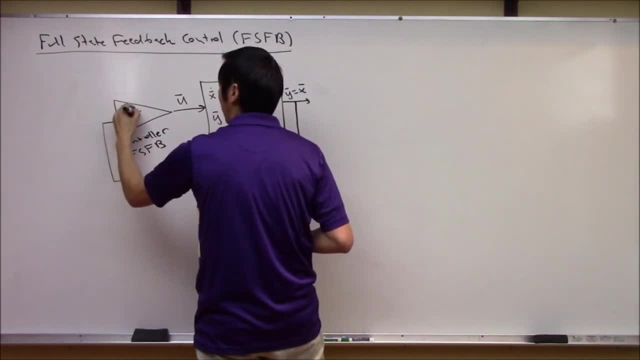 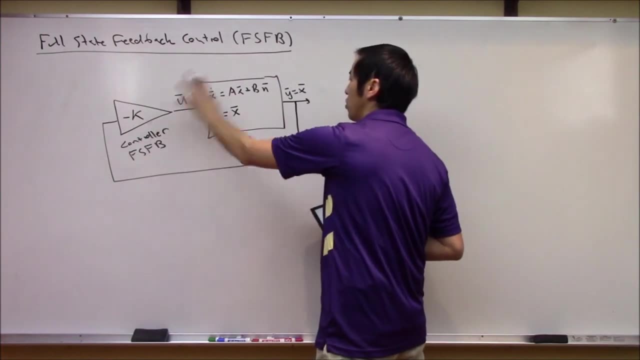 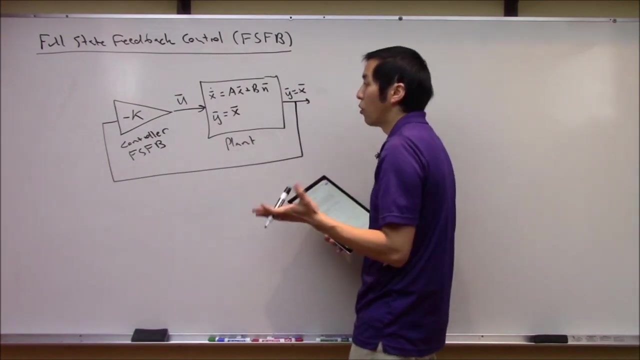 here, And what that looked like here was just a gain of negative k here right Now. within this context, we said that by choosing k intelligently, you can change the eigenvalues of this entire system to any arbitrary location, provided that this plant is controllable. okay, So you know me. 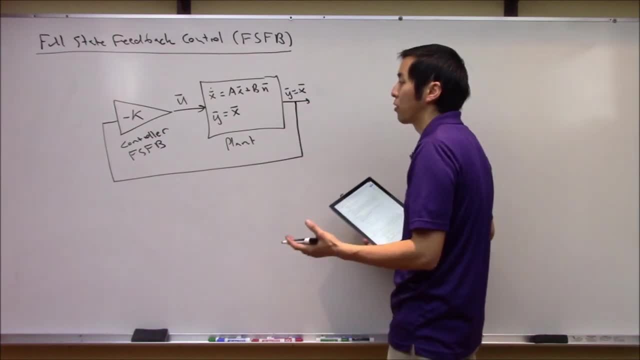 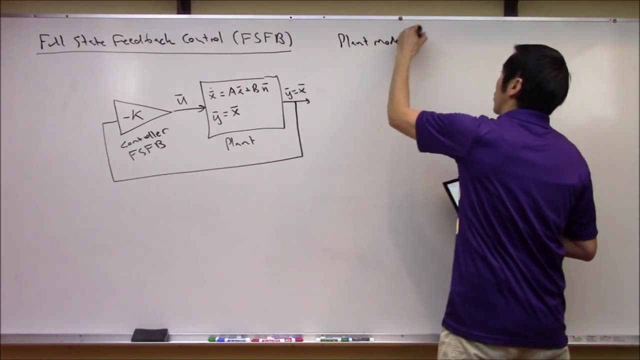 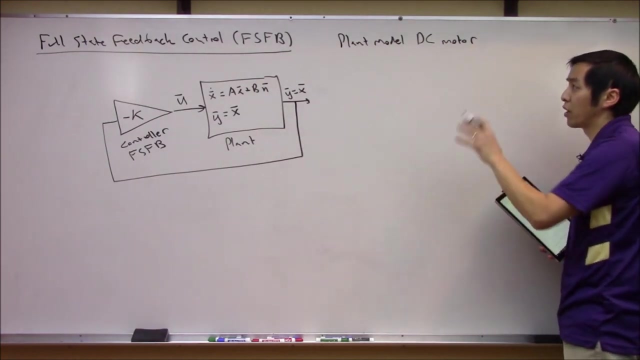 I always like to look at concrete examples because I think that helps with the analysis here. So let's look at a plant model here of a DC or direct current motor. okay, So again another plug for one of our other videos In another discussion we have. 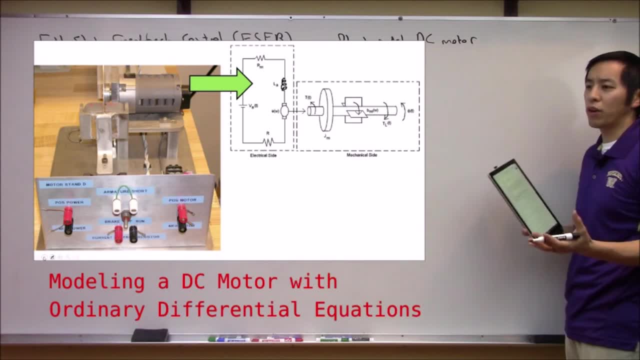 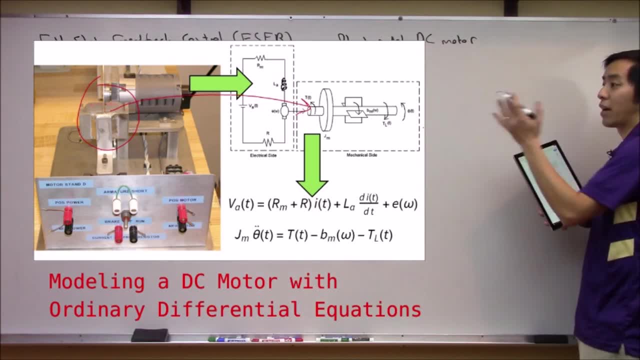 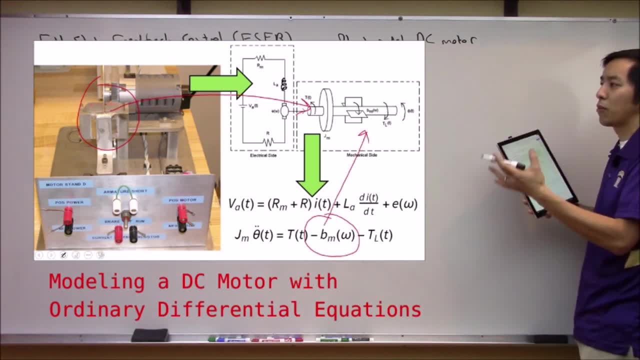 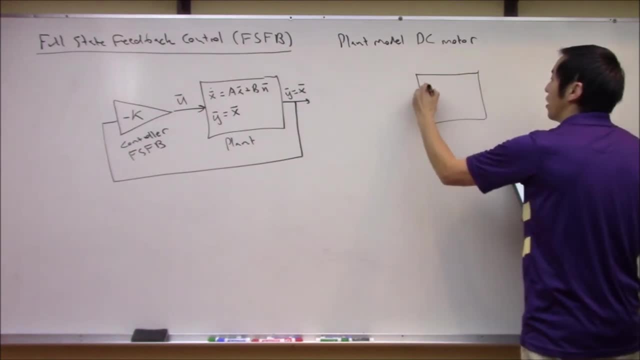 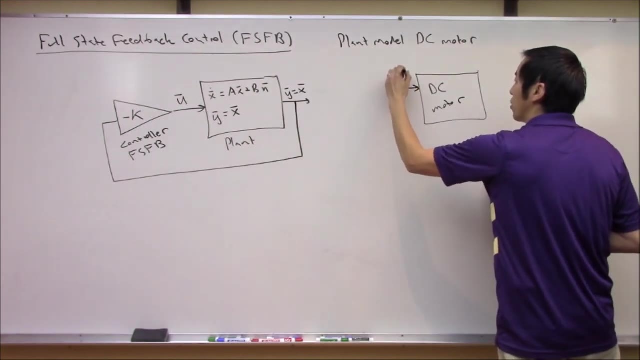 seeing that. If not, though, you can think of this as just a linear plant here that we're going to be using. It just happens to represent a DC motor here. So the system in our case, like I said here, was a DC motor, And the two inputs to this system here were a armature voltage- let's call it VA- of. 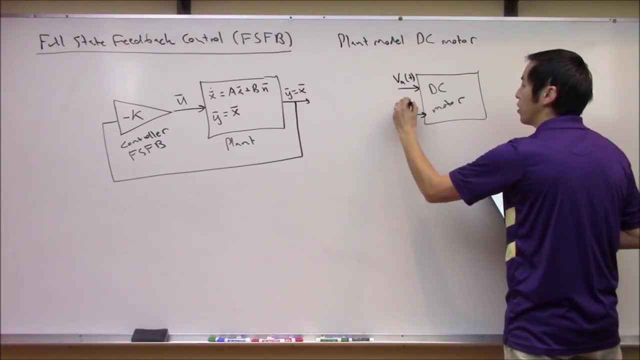 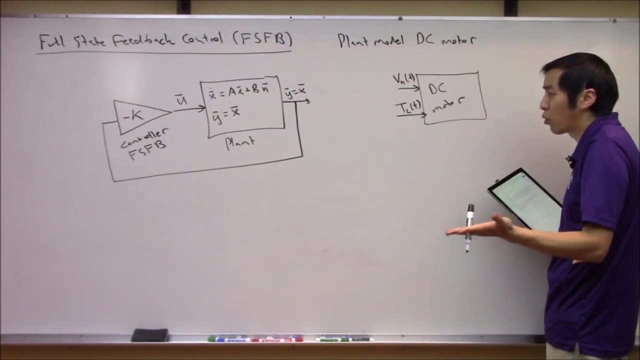 T here And also there was a disturbance torque to this, So that would represent somebody physically moving the wheel or the flywheel of the motor or some other kind of torque to the system right. And then those were the inputs here And the outputs. this system actually had three outputs. 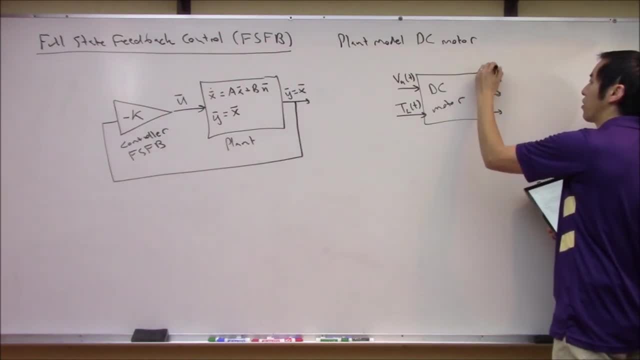 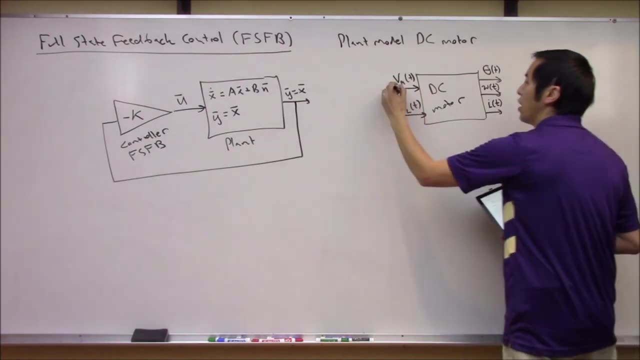 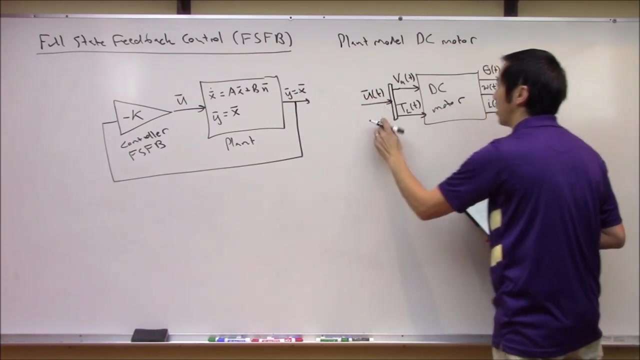 here. So there was the position of the motor, was something we're interested in- the velocity of the motor, let's call it omega of T and finally the current going through the motor here. So if we go ahead and maybe Visualize this here as a DMUX here We can say this is the entire control vector U of T here And then 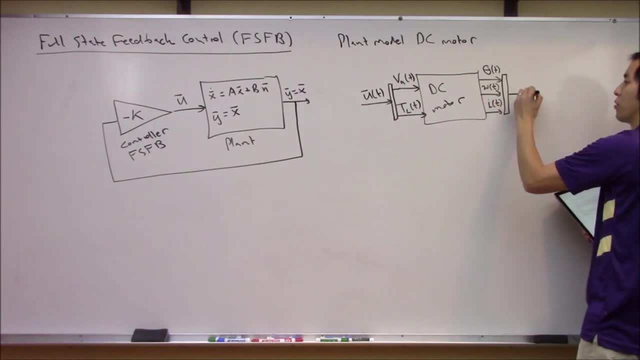 finally, we can MUX up these three inputs, or, sorry, these three outputs, to get the entire output of the system, which in this case was the entire state. Okay, So here's the physical inputs and outputs of the system, And then the state-space representation governing this input-output relationship. Again, 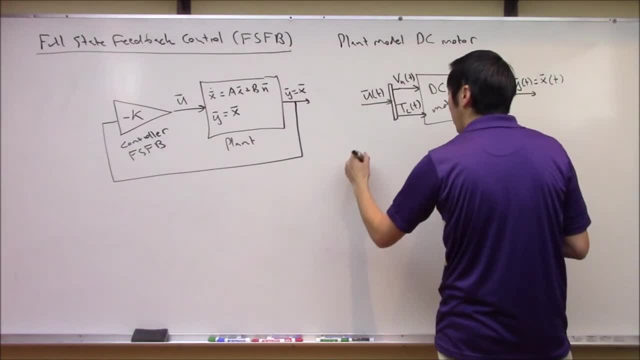 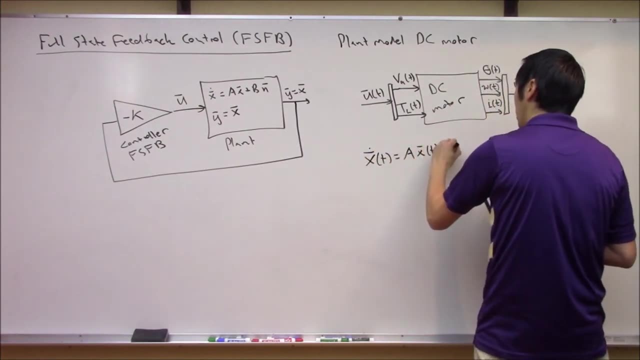 watch that video. I'm just going to go ahead and write it down here. We basically wrote this down as a linear system And normalize that. So, for example, this it looks like, And in this case we got the data, Stratton data on what we used to watch Swarz's system: X dot is equal. 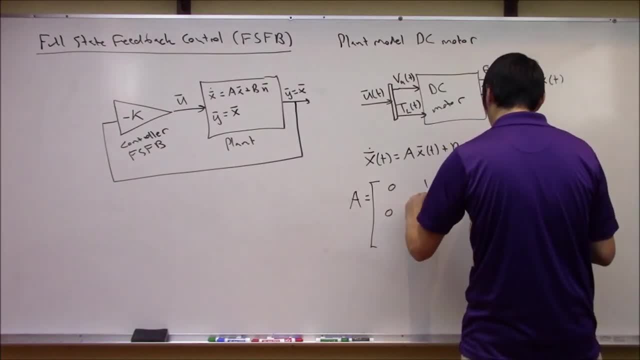 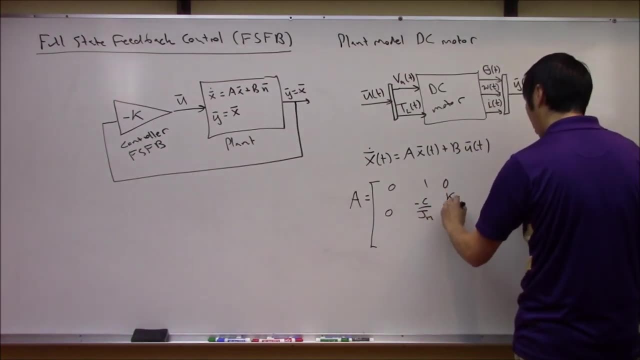 to AX plus BU, right, And in this case your A matrix looked like a 0100 minus C over JM, which is so damping over moment of inertia, And then our mechanical machine constant over the moment of inertia, And then this last row was zero minus KV, or electrical machine constant over the inductance of the motor. 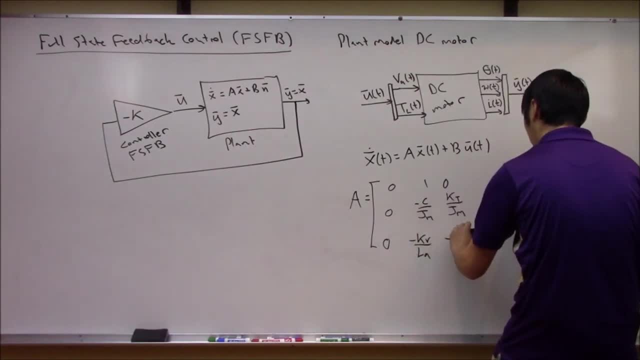 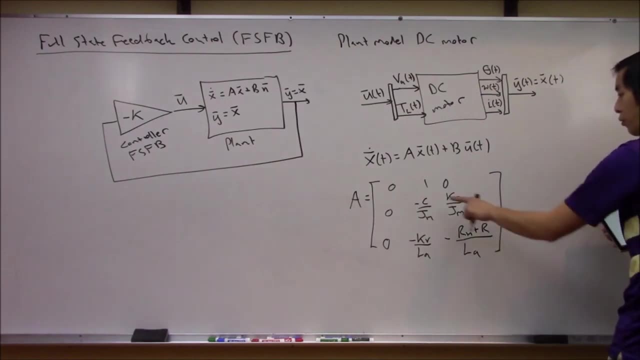 Okay, So the output benefici こう こ. Quantum girls. and they didn't measure each reflectore. Okay, the motor minus the quantity, rm plus r, so that's the total resistance of this motor over the inductance here. so that was our three by three a matrix here and our b matrix. maybe we will write. 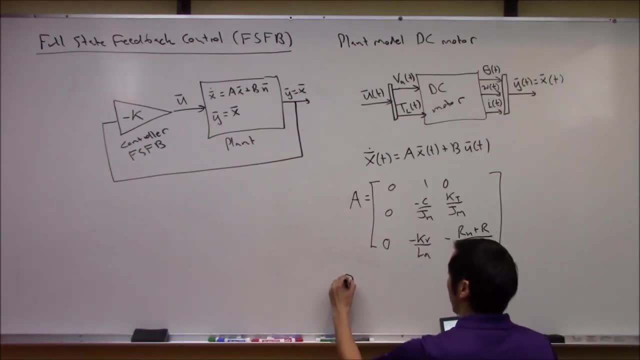 it. uh, let me write it down here a little bit lower, actually it might be easier. and our b matrix here was a three by two, right, because there's two inputs here. so the first column here which dealt with the armature voltage was just zero, zero one over la, and the other input here was zero minus one. 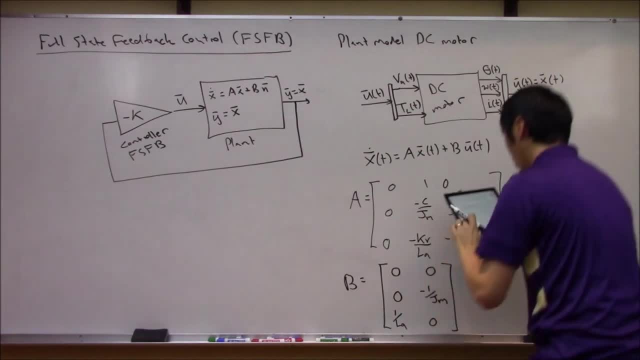 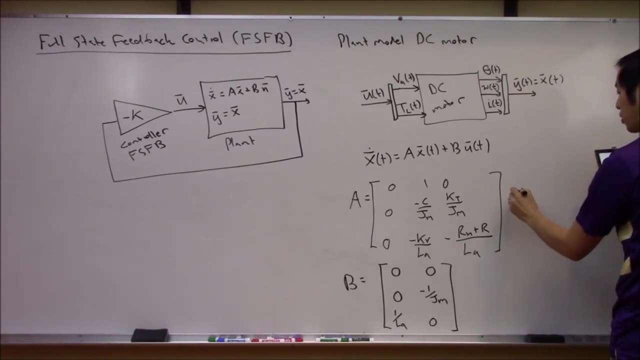 over jm zero, great, okay, so here was our states here and um numerically here. if you were to go plug in actual values for our particular motor here, um, let's just pick some numerical values that we can use for the purpose of this discussion. so some realistic values would look something. 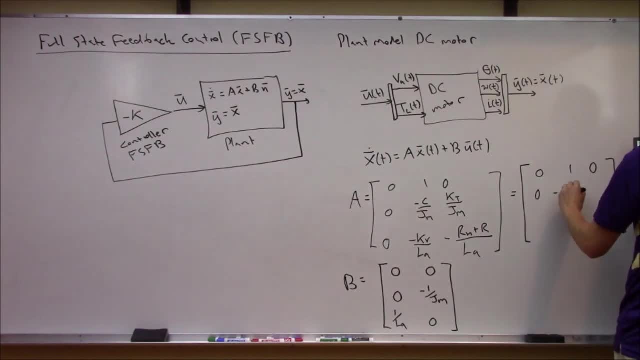 like this, and we're going to use this for the purpose of this discussion, so let's just pick like: uh, zero, one, zero, zero minus zero, point two, nine, seventy one point nine, three, zero minus sixty three point two, four, and then minus one thousand twenty point three, five. that was our a matrix, and 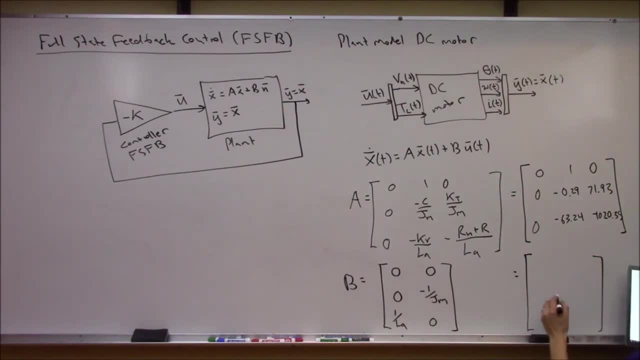 then a numerical value for our b matrix here was going to be: uh, where was it here? um, uh, yeah here, zero, zero, 141.81, and then 0, and then actually I forgot to write down this value, but we actually don't. 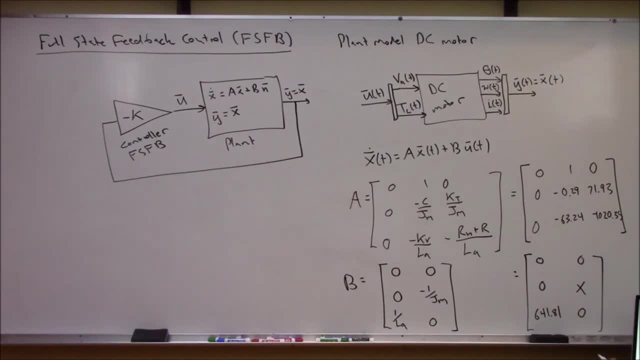 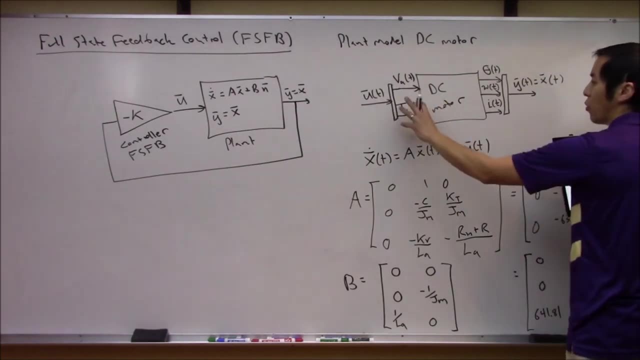 care about this value here. We'll see here in a second why. because really what we're interested in doing is we only want to use the first input for control here, So we're going to ignore this second external disturbance torque. We're only going to try to control the position or the 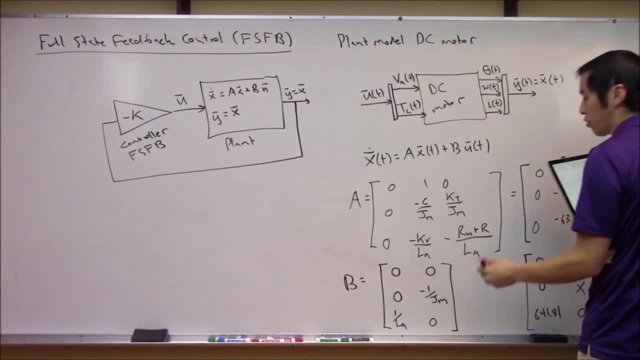 velocity or the current of the motor using the voltage that we're going to send to it. So really we don't care about this column of the B matrix here. So really it doesn't really matter what numerical value is, because we're going to neglect it and only pick this column here for the B matrix. 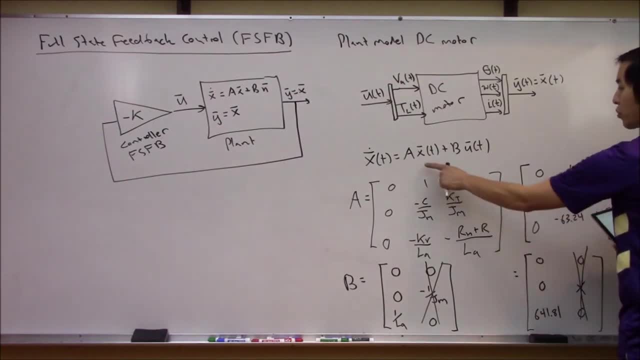 Okay. so again, maybe what also it would be helpful is we should write down what is the state and what is the control vector here in this case. So maybe let's do that. I didn't use the board very well here, but I think we can. maybe we'll just write it. yeah, maybe right over here. 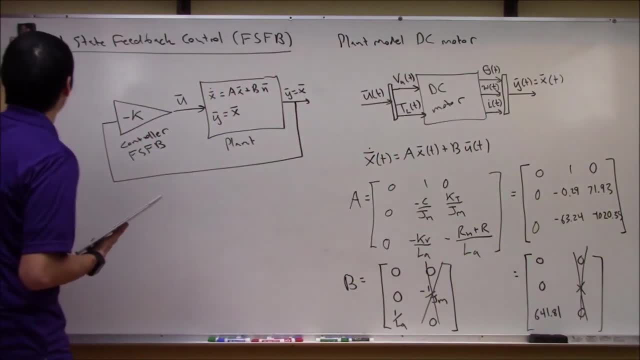 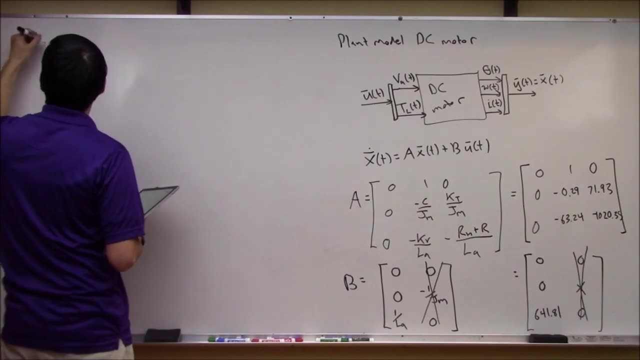 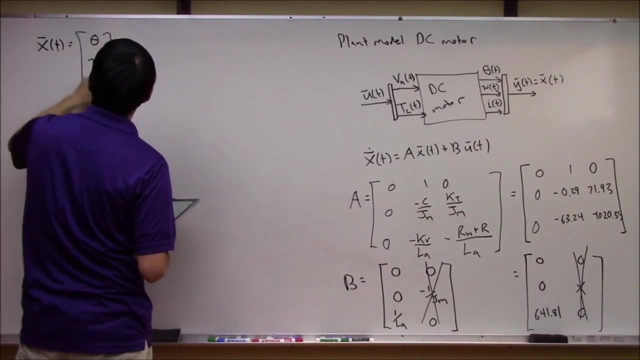 okay, just so we We have it in our memory, So let me erase some of this. Okay, so our state vector in this case was going to be the position of the motor, the velocity of the motor and the current through the motor here, And then our control. 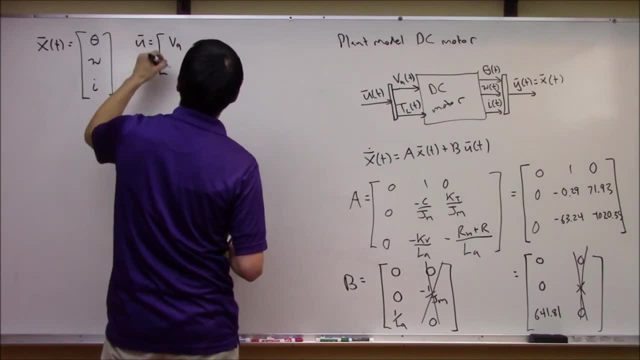 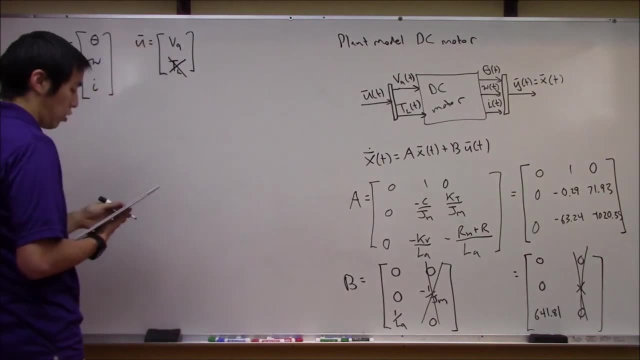 vector here was going to be the armature voltage and the disturbance load, But, like we said, we're not interested in the disturbance torque, We're only going to be using the armature voltage to control the system here. So the picture that goes along with this now is in the context. 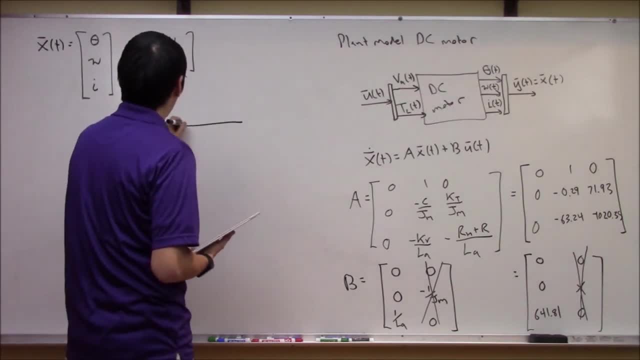 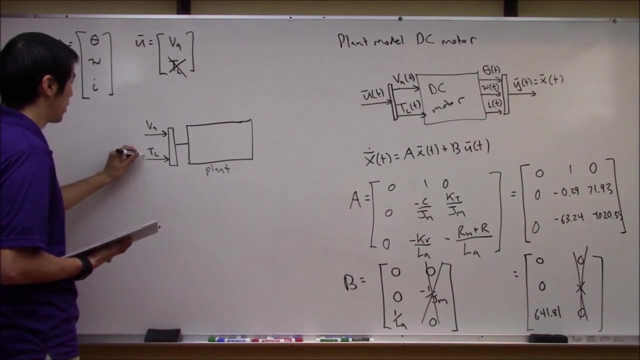 of having our full state feedback system here. right, we are going to have our plant model right, with two inputs here. we said was our armature voltage and then our disturbance torque here, And all we're going to do here is we're going to basically- I don't know- just put. 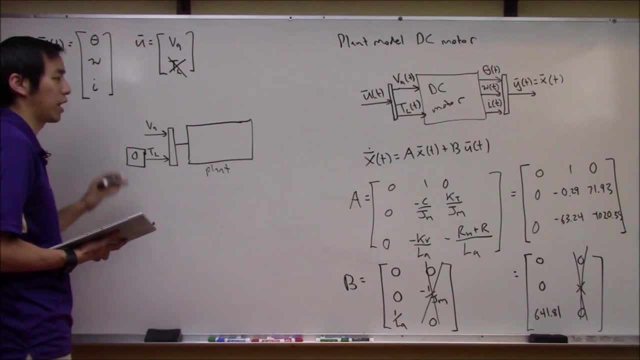 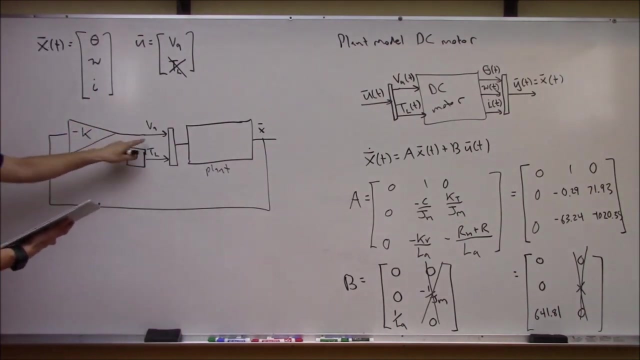 in a constant zero going into the disturbance torque. We're gonna ignore it here. right Then state coming out and we are now going to wrap this back and run it through a negative k and that's how we're going to control our, our armature voltage. going to this plant here, right to the one, 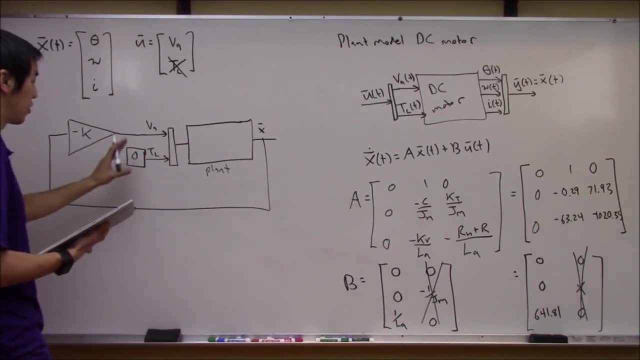 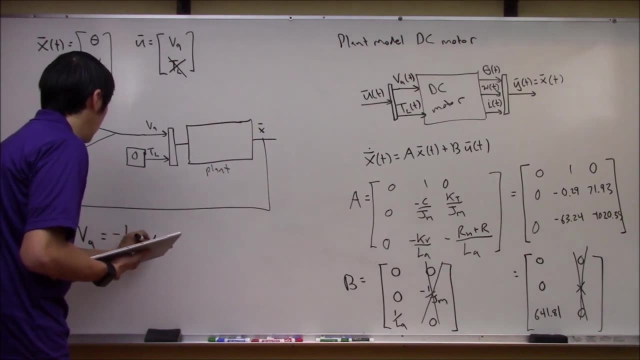 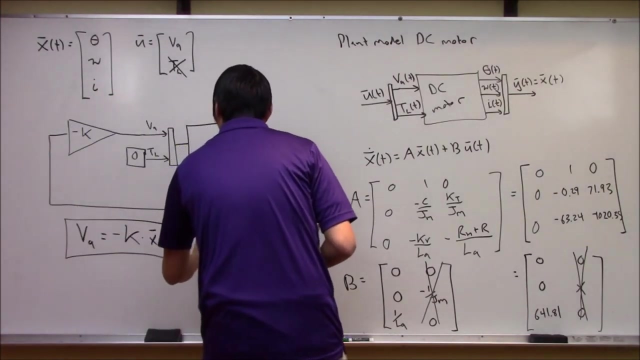 input we're going to use for control, all right. so again under this control law, we see that, all right, that the armature voltage is going to be minus k times the state vector, right. so this was going to be our control law here. this is our full state feedback control law, where we are only using the 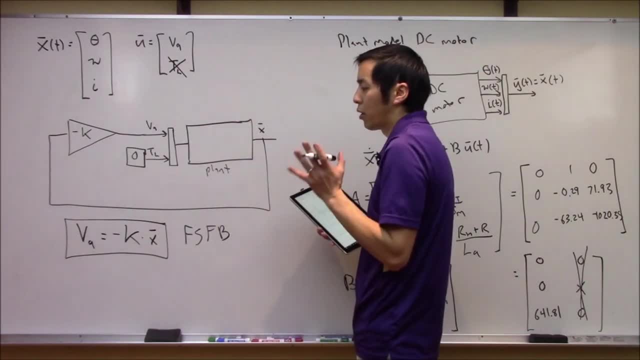 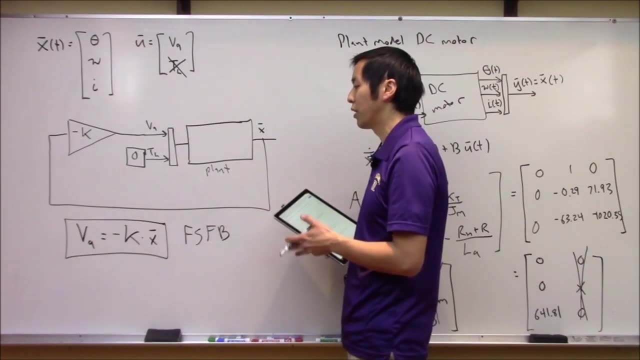 first input here, um, for control here. so i want to make, uh, make that clear here, because although we're just using a single input, one nice thing about full state feedback control here is it really nicely and gracefully handles multiple inputs here. so if you wanted to use both the 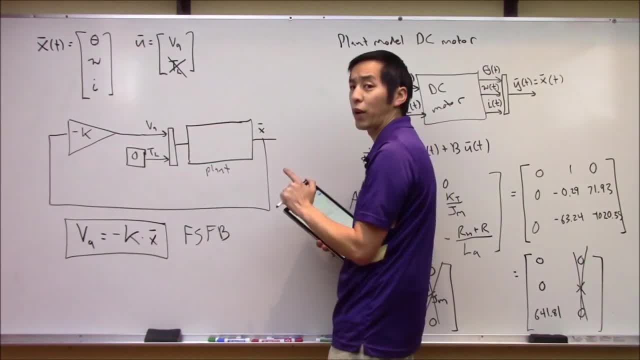 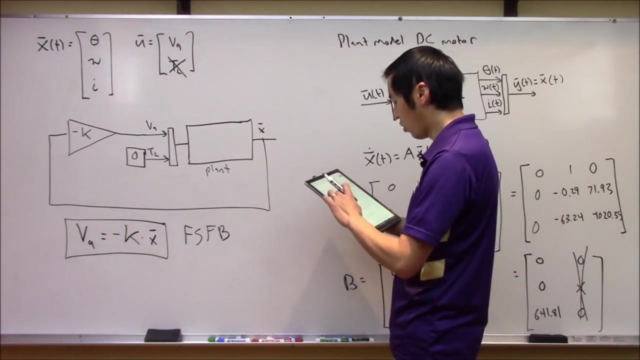 voltage and the disturbance torque to try to control the state or to regulate it to zero. you could just go through all of this discussion here and it would be- uh, it would directly follow here, and we're not making any um specializations that are going to cripple us here in the future. um, okay, so with that, what we should maybe do here: 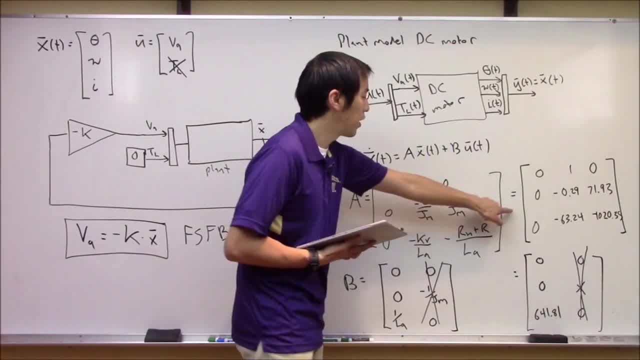 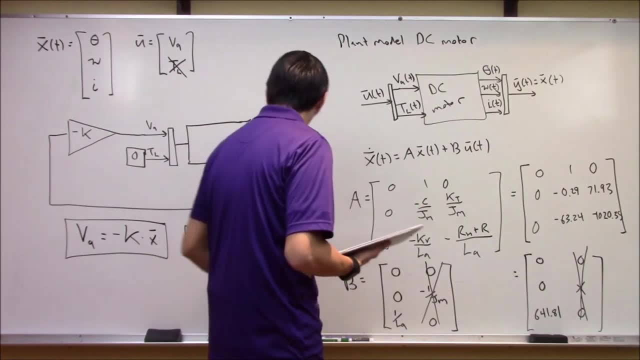 is: let's go ahead. and now that we have a numerical value for our, a matrix, it might be uh handy to go ahead and just look at where are the open loop eigenvalues of this system here? where do the plant, where does it have eigenvalues? uh, naturally, without any control. 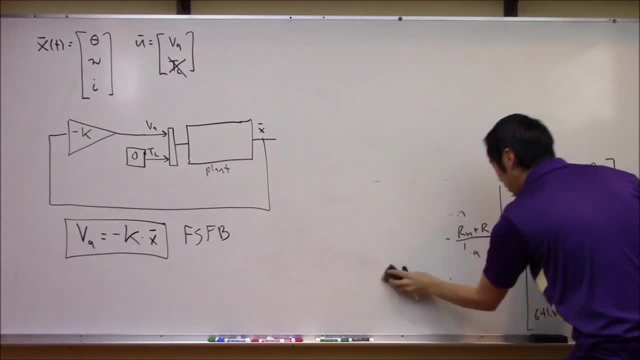 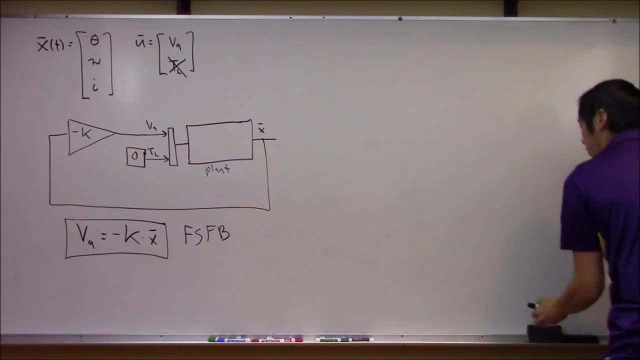 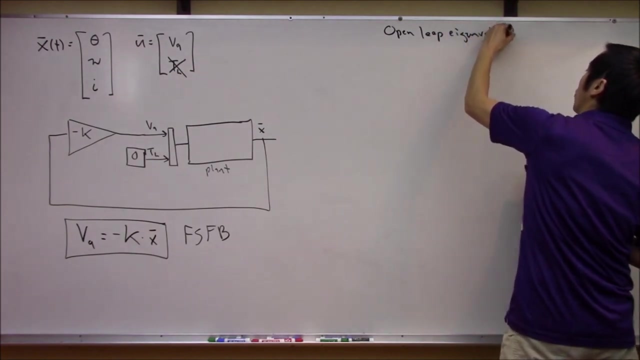 so let's do that right now. okay, let me erase the board here. so to get the open loop eigenvalues of this system. i think it's pretty simple. you guys all know how to do that here- open loop eigenvalues. so we can just run over to matlab and we will basically ask it to say: 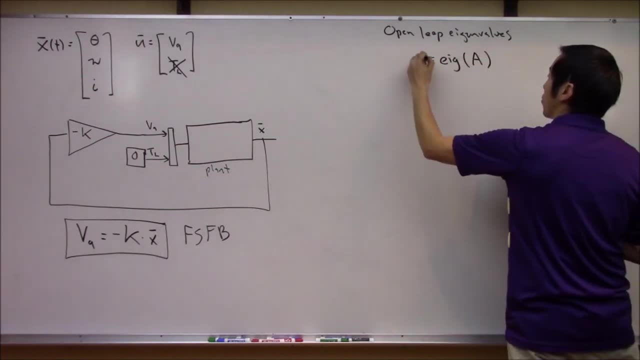 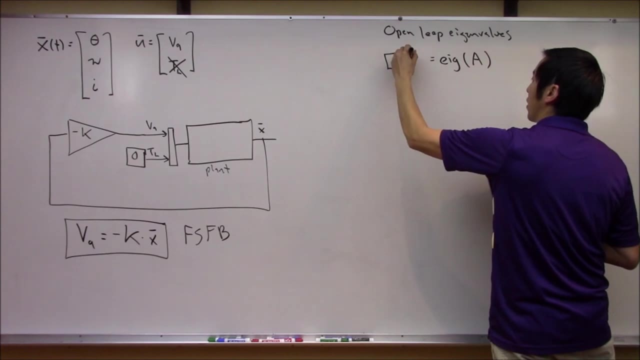 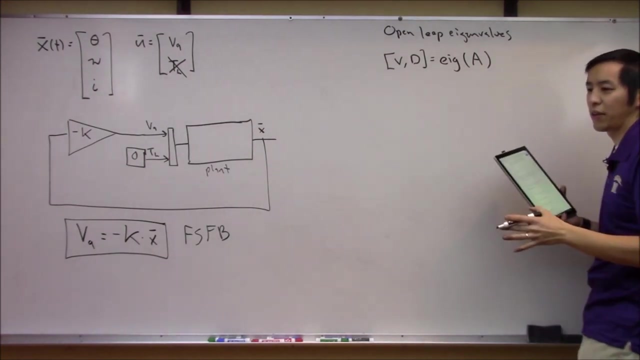 i of a right and this is going to return basically our eigenvalues. i think it actually gives you the eigenvalues. uh, i can't ever remember which order one of these is of eigenvalues. one of them is the eigenvectors. it doesn't really matter. right, you can go here and you can calculate the eigenvalues in matlab. 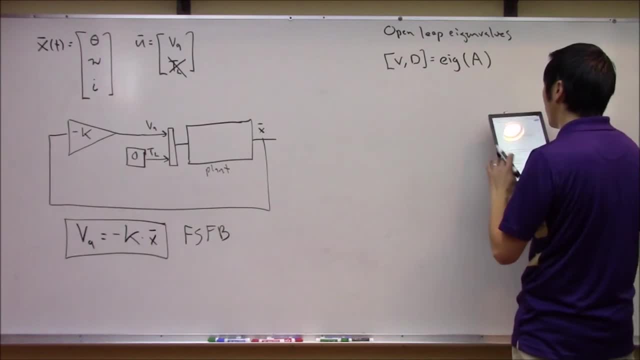 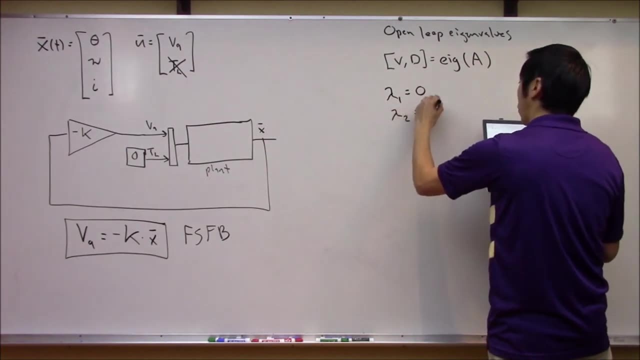 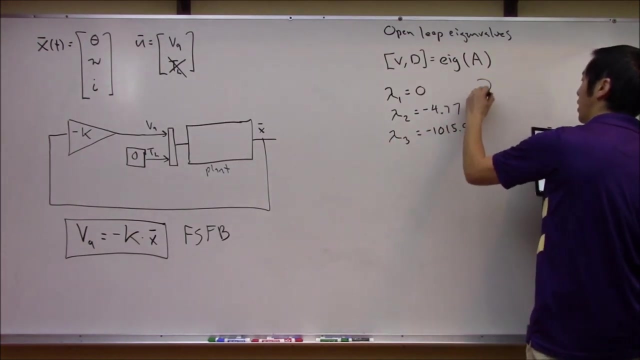 you could do it by hand here, um, but what you would end up with here is we would end up with eigenvalues of lambda one here being at zero. you'd have a lambda two here at minus 4.77, and then a lambda three here of minus 1015.9 here. so again, these are the open loop. 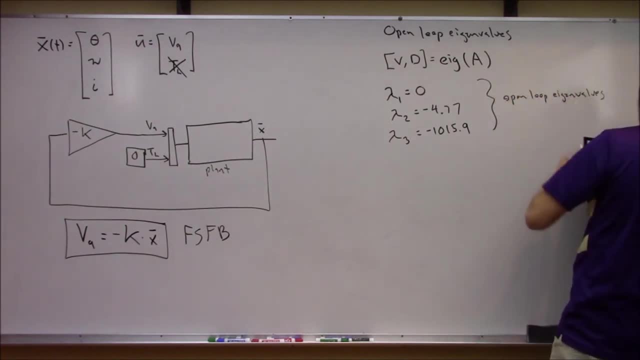 eigenvalues. okay, so, uh, what we can do here is let's just sketch these on the real imaginary axis here. so let me just go ahead and draw. here's our real, here's our imaginary axis, and this is not not going to be to scale here, maybe. 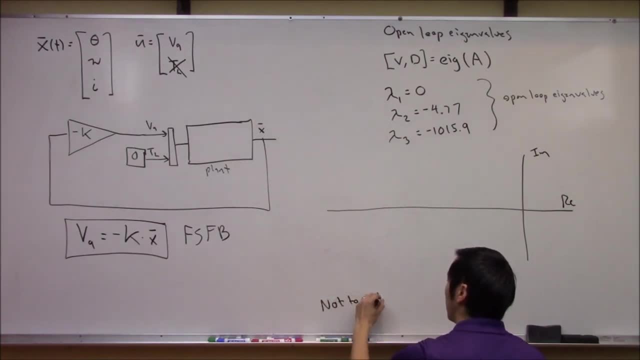 we should make. make a note here not to scale right, because you can kind of see there are some here that are. you know, there's an eigenvalue right here, then there's something way over here at um 1015.. so tell you what, actually, to help visualize that i've got these little uh, blue x's here that we 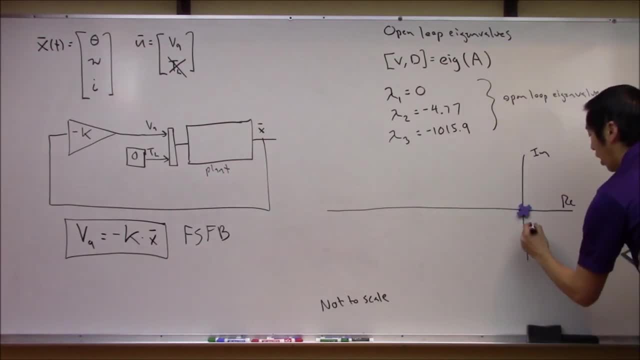 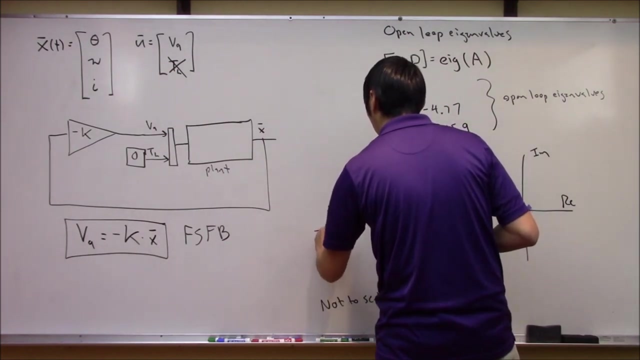 can put here. so here's one. here is an eigenvalue, here at zero, right. then we have another one here at minus uh, 4.77, right. so let me put another blue x here. that's another open loop eigenvalue. and then finally we have one way over here at minus 1015.9. 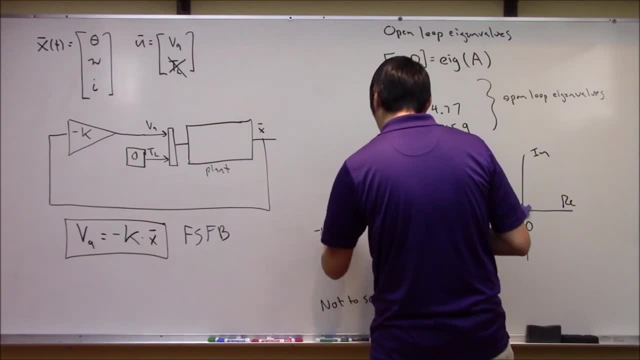 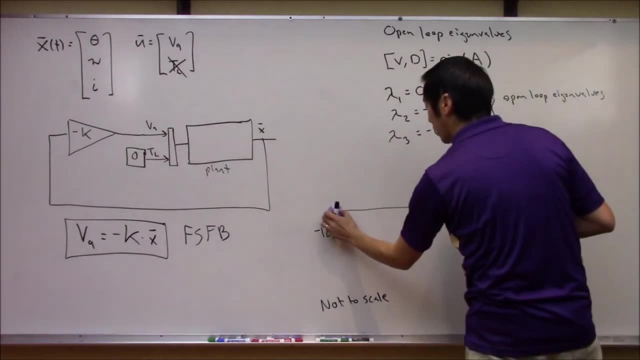 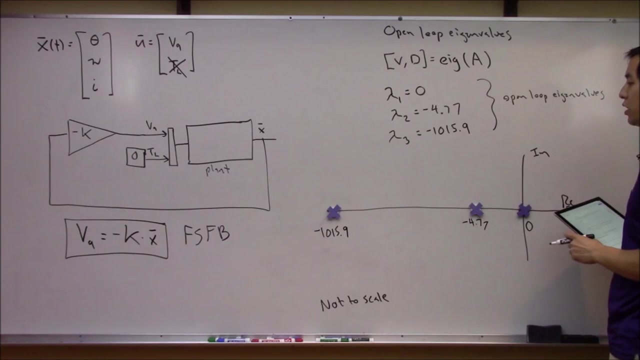 uh, what was that point? 0.9, right, oops, sorry, let me get rid of this black x. i forgot. we're using our little blue magnets here to represent all of these here, right, okay, so we've got our open loop eigen values here. uh, we can now start thinking about designing a controller k to move these eigenvalues. 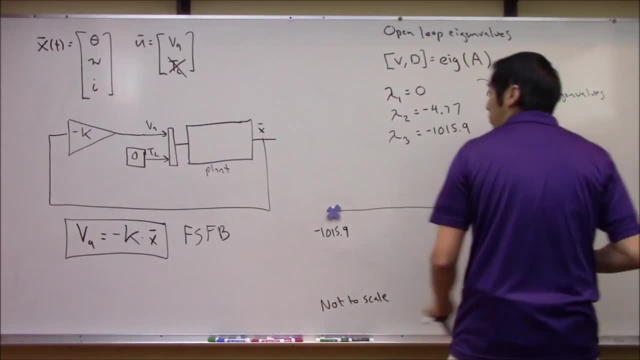 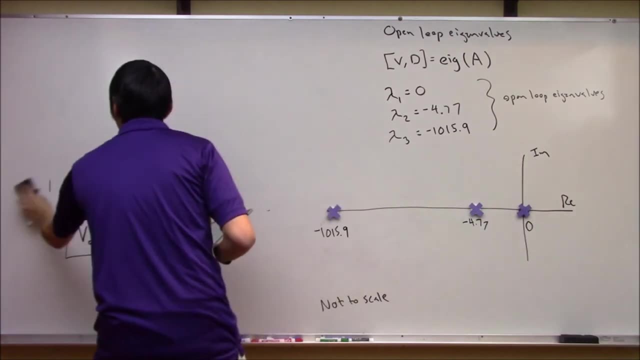 to some location that we desire here. so the first thing we got to do here, right, is we need to go ahead and make our controllability matrix to ensure that this is controllable and that our full state feedback controller has a chance of working the way we want it to right. so let's just. 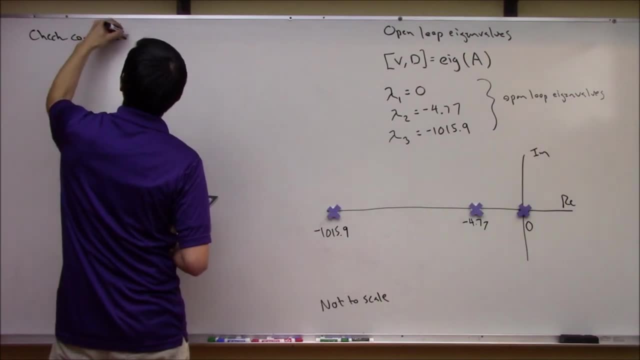 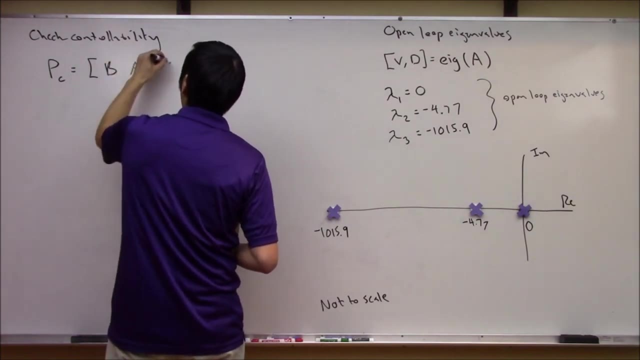 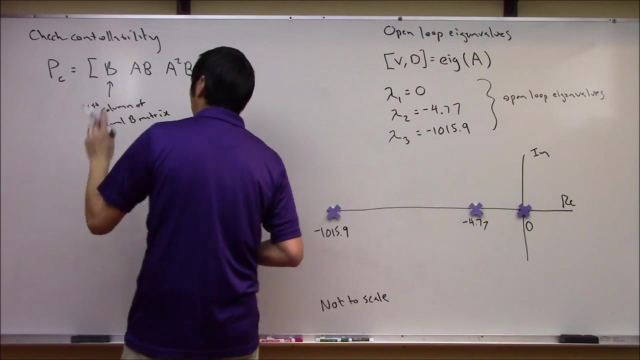 quickly check controllability, right? so we're going to make our controllability matrix pc, which is going to be b, a, b, a, squared b, right. and again, we're going to make a note here that this b here is only the first column of the original b matrix, right, because that's all we're using. it's just the. 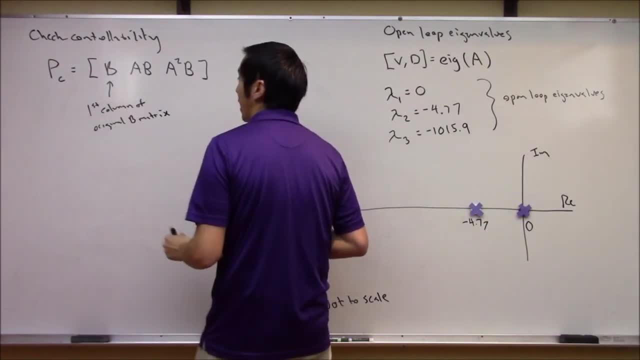 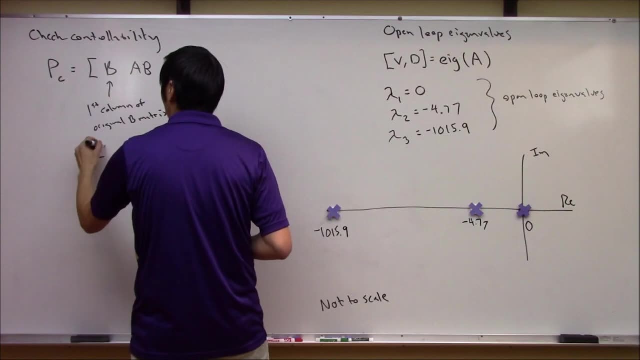 first input here, right, so we can run over here to matlab and we could go and basically give it. uh, we could. we could build this matrix ourself if we want. or, like we talked about last time, there's this function called ctrb for the controllability matrix. you just give it the a matrix, then you give. 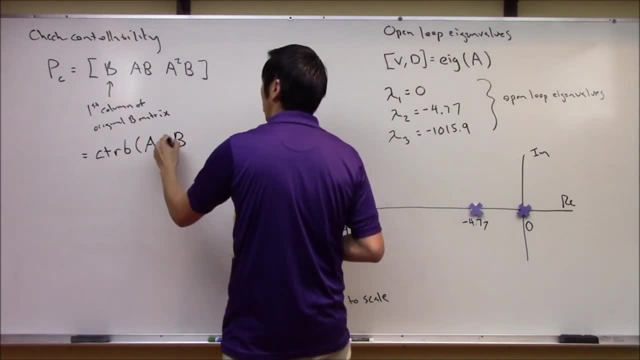 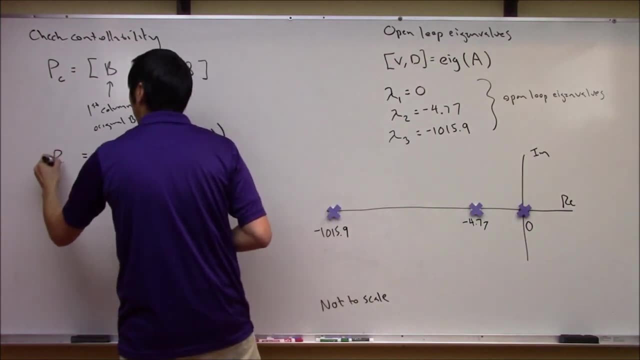 it, the b matrix. and again, since we only want the first column, maybe what we should denote here is, maybe we should do something like: all rows, column one here, right, and this would give us the controllability matrix pc here. and then what we're going to do is we're going to check the rank of. 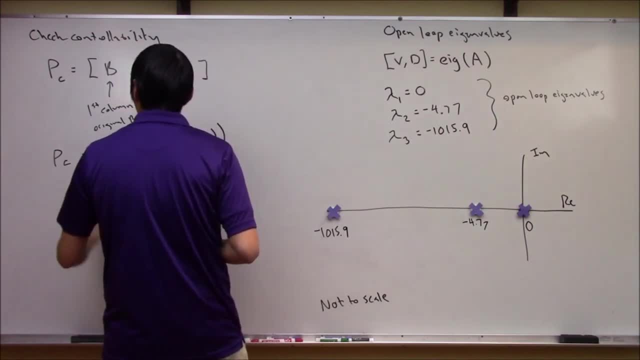 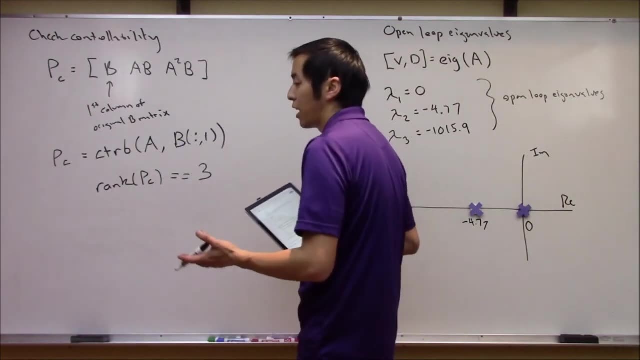 this thing. right, we're going to check the rank of pc and we're going to make sure that this is equal to the number of states, which is three in this case. right and again, um, and to save ourselves going back and forth and breaking our flow here, i'll just- i'll- make the claim that this actually 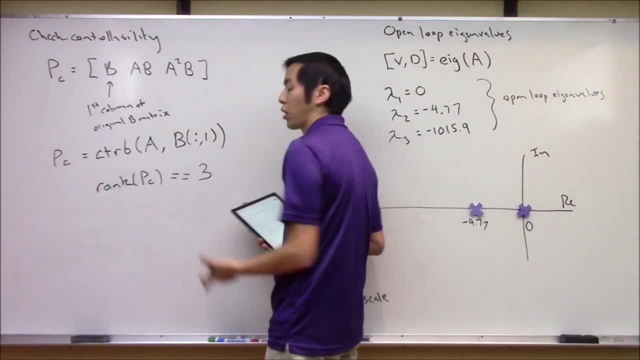 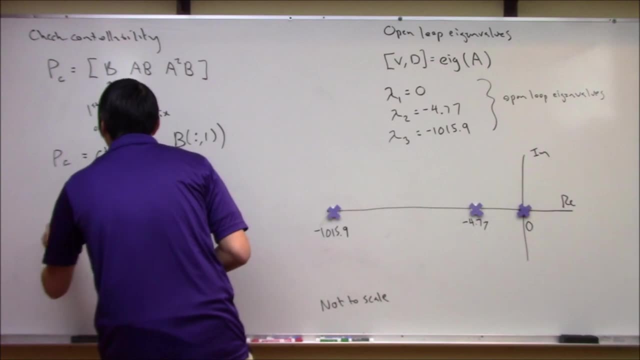 is true. if you run this in matlab, um yeah you'll, this will come out to be a logical truth. so it's great this system is controllable, so we can say that the system- or actually slash plant maybe is- is more, uh, accurate plant is controllable. 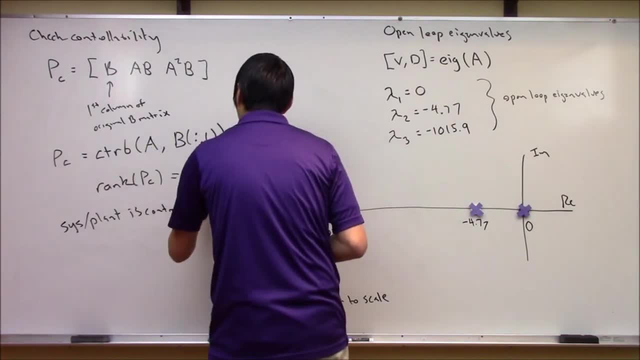 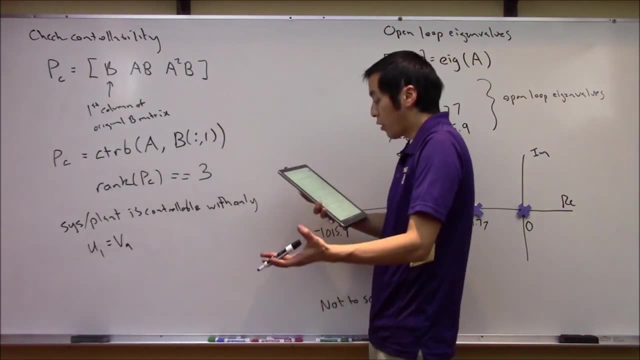 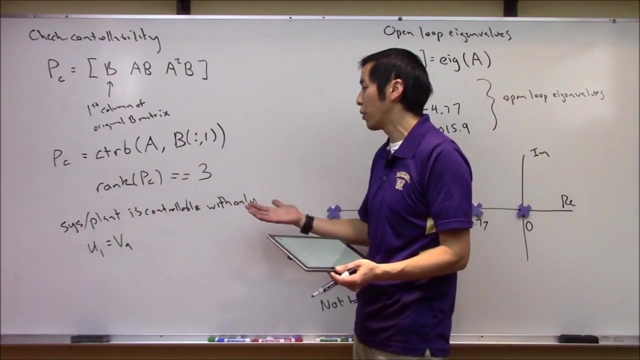 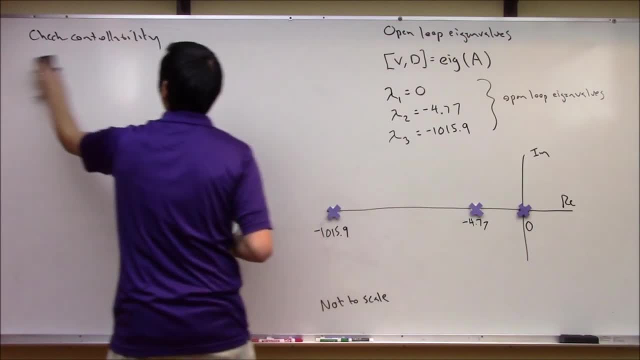 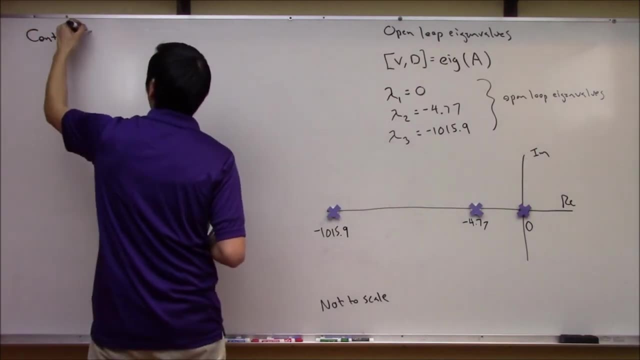 issue here. this is where we're going to start running into some of these practical implementation issues that we were talking about here, right? so the first issue that i want to look at here is- let's just call it maybe under this big heading of how let's call control saturation. 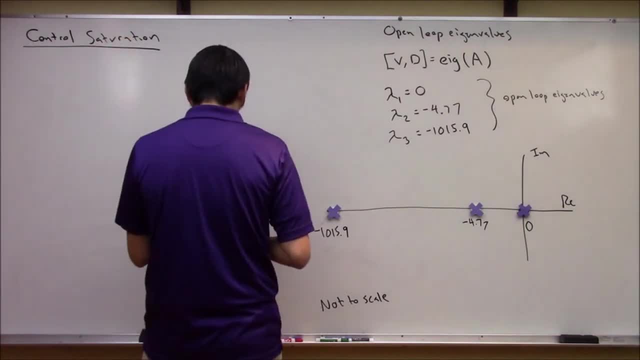 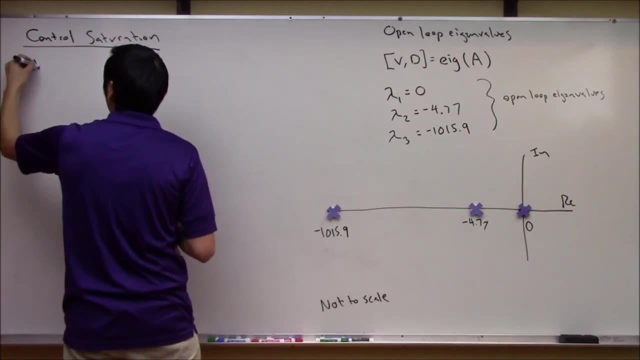 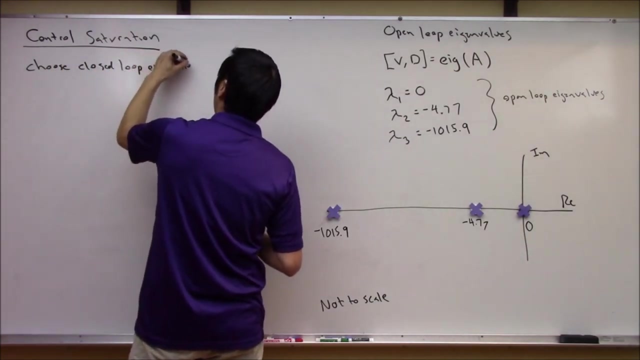 problems here, right? okay, so to set the stage for this here: um again, we've got our open loop eigenvalues. let's just go ahead and choose some open- uh, choose closed loop locations, right. so choose closed loop eigen values. slash poles, right, and maybe for the remainder of this, 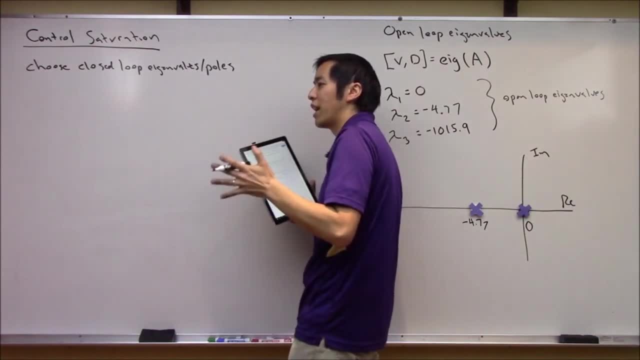 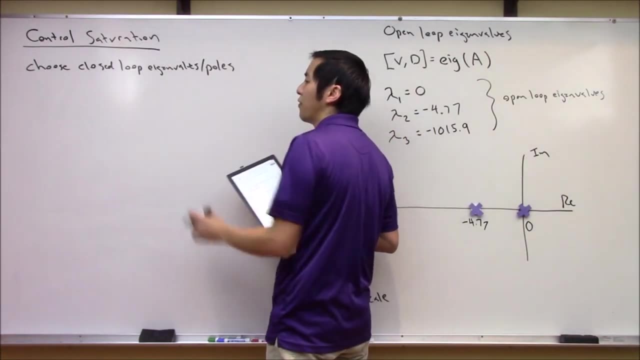 discussion here. i i think everyone realizes right that eigenvalues are not exactly the same thing as poles. right, you might have pole zero, cancellation or something like that. but, um, in general, right, the eigenvalues are a larger set than the poles of a given transfer function. but to keep our discussion, 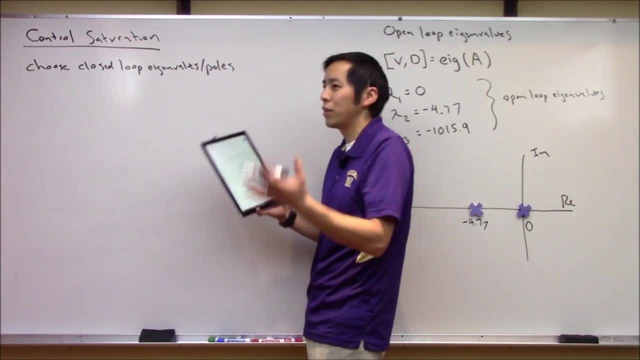 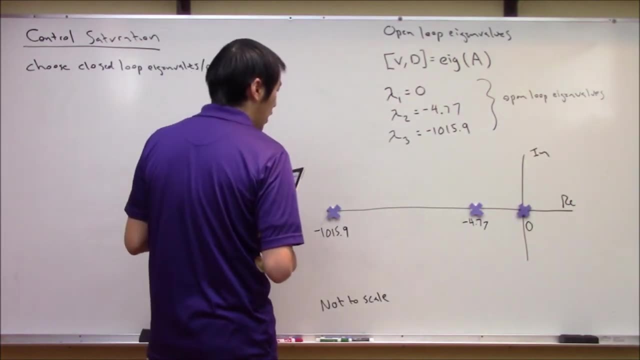 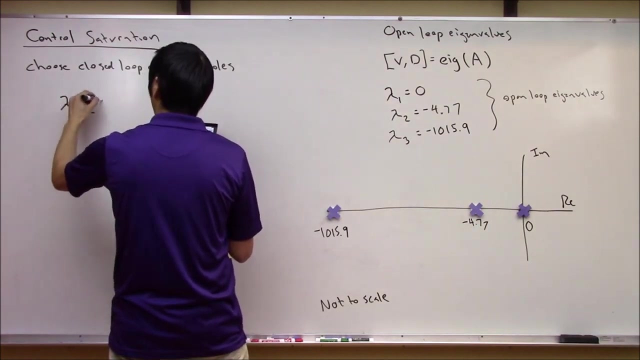 simple. let's interchangeably use the word pole and eigenvalue- they really mean the same thing for this case. so let's try to move them to some arbitrary location. so i don't know. let's pick something like um, i don't know, uh, how about? how about a lambda, uh, one closed loop, what i'd like. 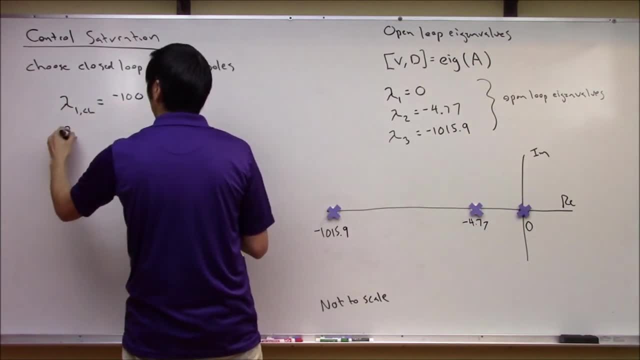 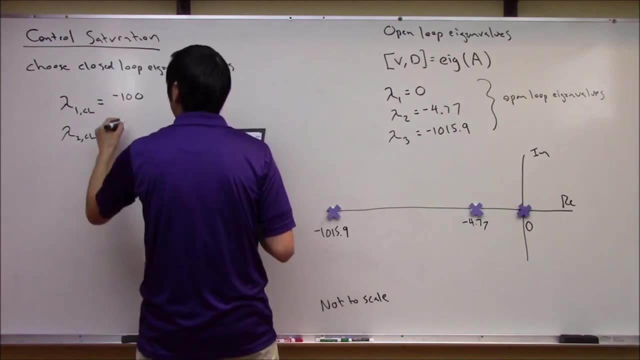 here is i don't know how about minus 100? how about lambda 2 closed loop of minus 200 or no, sorry, minus 110 is what i've got here on in my example here, and a lambda 3 closed loop of minus 120 here, right, 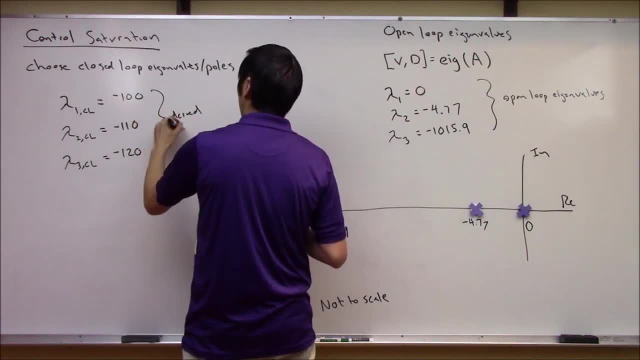 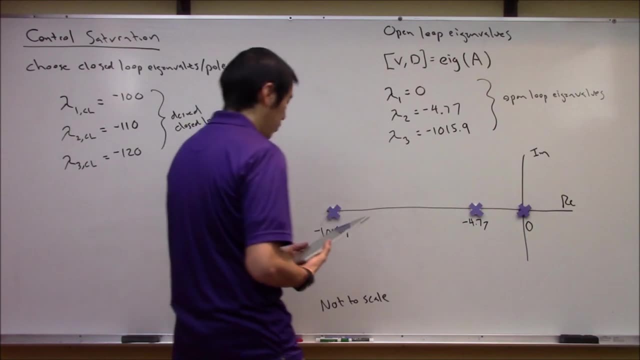 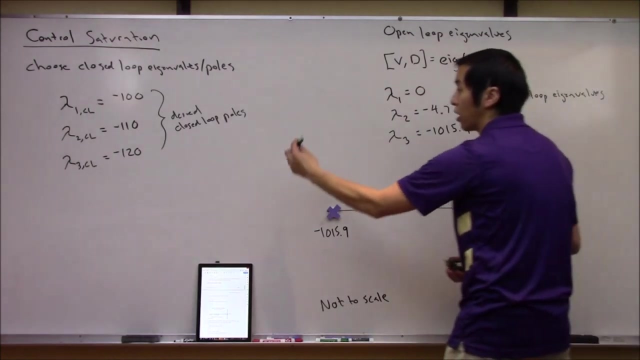 these are my desired closed loop poles, right? so to visualize that over here we can. we can go ahead and let's grab a couple of these other dots here, all right? so i've got some green dots to represent our desired closed loop poles, so we see that normally. here you know, our open loop poles are. 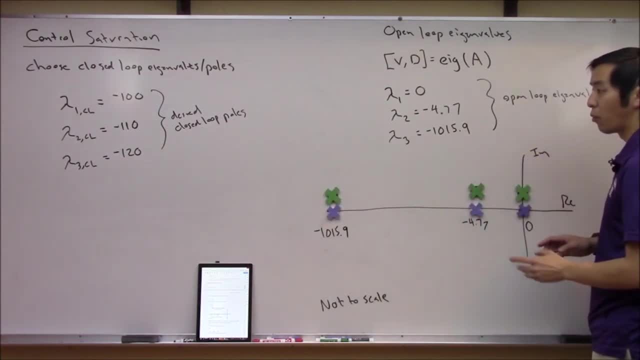 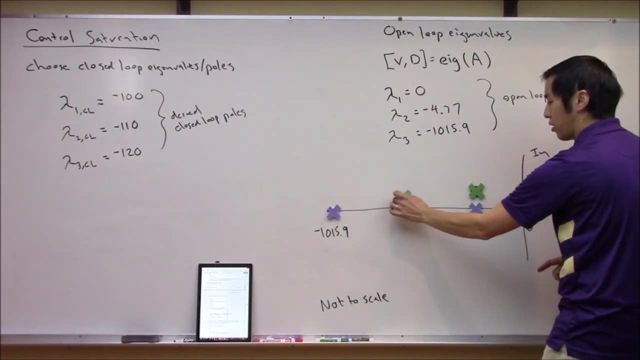 sitting here at the blue locations, right, but what i want is i want them at this minus 100, minus 110. what i'm talking about is, you know, taking one of these and moving them here, taking this other one, maybe, moving it here, and then taking this one and moving it all the way over here, right? so maybe? 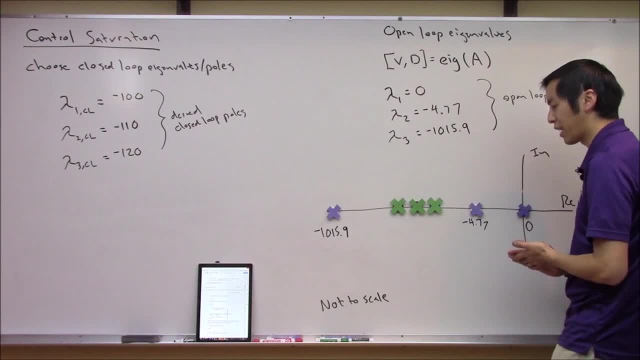 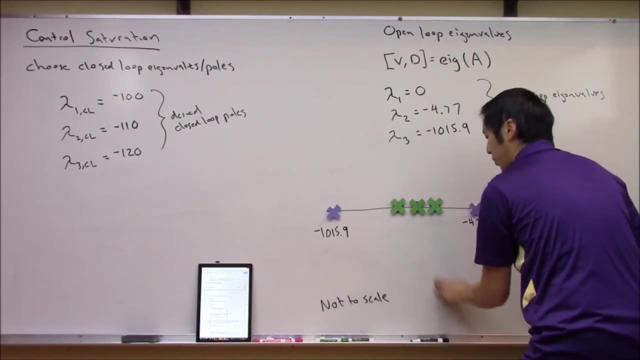 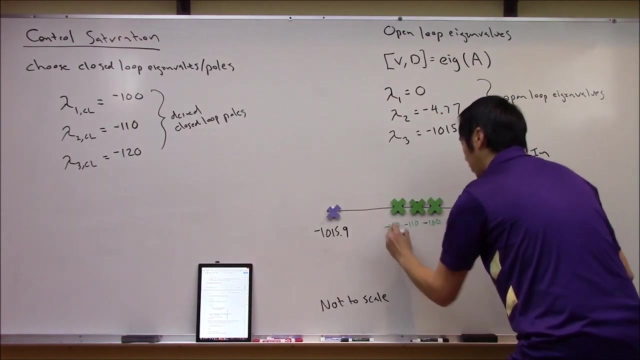 let's put them here on the line, right, something like that. okay, so i've got this thing here at minus 100. well, actually tell you, let's do this in a different color so we can keep them straight. maybe we'll do them in green here, right? so here's minus 100, minus 110, minus 120.. right, 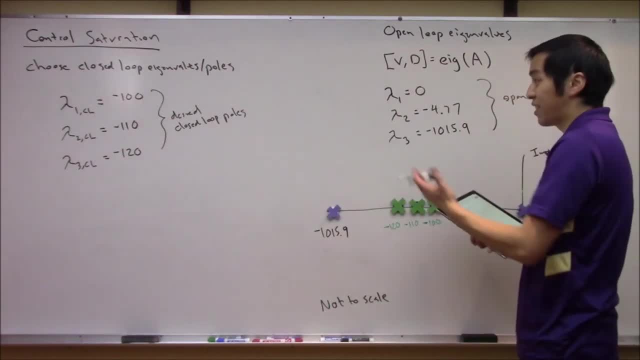 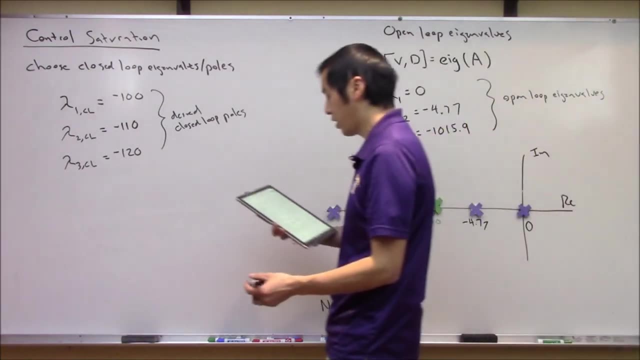 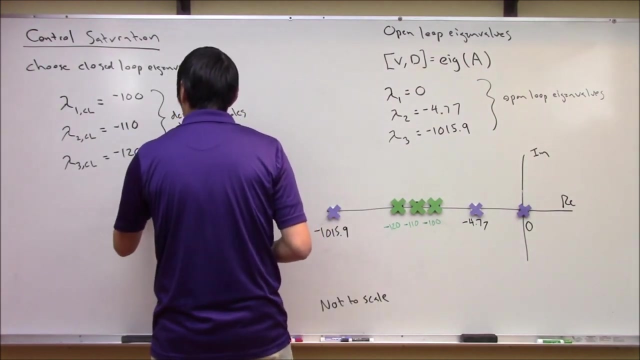 okay. so, um, since the system is controllable, we show that mathematically, there's this is totally feasible. in fact, the way i'm going to calculate my k matrix to get this done here right, is i'm just going to go over to matlab and we're just going to say: okay, matlab, do pole placement like? 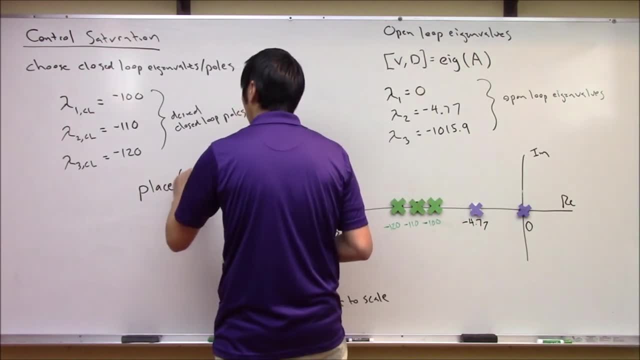 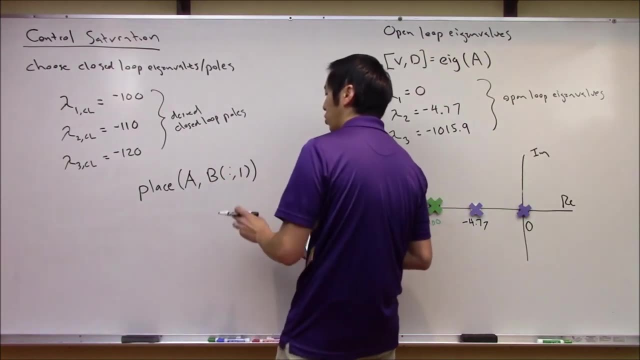 we talked about last time. so i'm just going to say place, give it the a matrix, give it the b matrix and again give it the all rows, column one here, right, because i only want the first um control here, right? oh sorry, yep, place. and then give it all the desired locations here of your poles, here, right. so i? 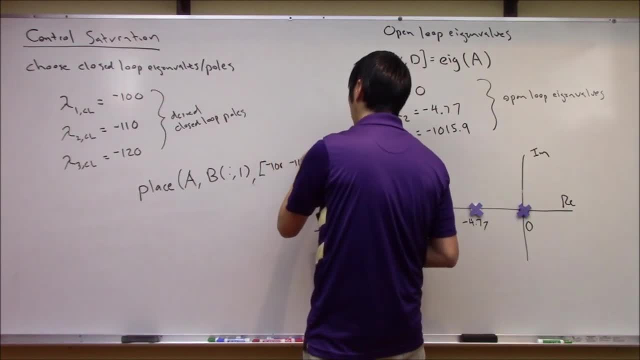 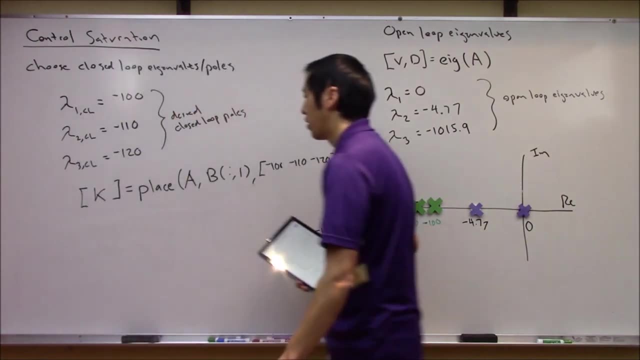 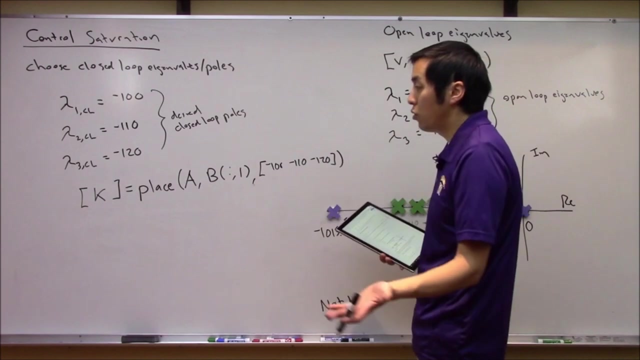 want it at minus 100, minus 110, minus 120, right, and just go ahead and this will basically return for you the the uh full state feedback, matrix k that you need in order to make this thing happen. so if you do that in uh, in matlab again, we'll go over to matlab in a second, just to see what. 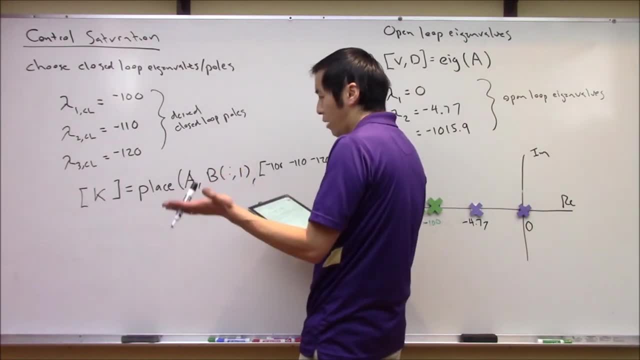 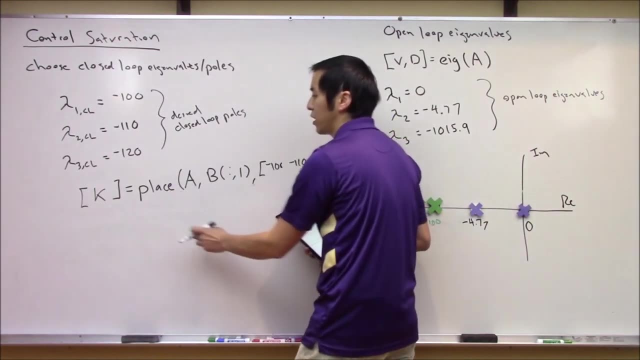 happens here? um, actually, you know what? maybe now is an excellent time just to plug this in, and then maybe we will go ahead and simulate this here. so what we'll do is: let's run over to matlab. let's go ahead and do this calculation. figure out what. 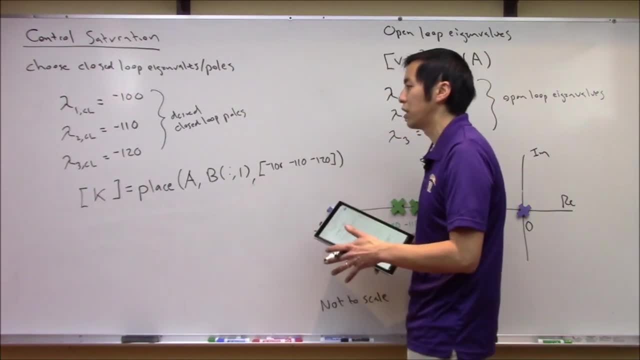 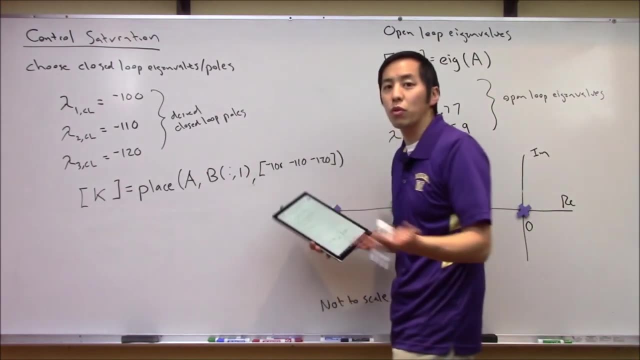 our k matrix is, and then let's build a simulink model here to run it and check to see: did the eigenvalues actually go where they were, where they were supposed to, and we'll see if anything else popped up while we were trying to do this. okay, all right, so let's- uh, let's- pause the filming. 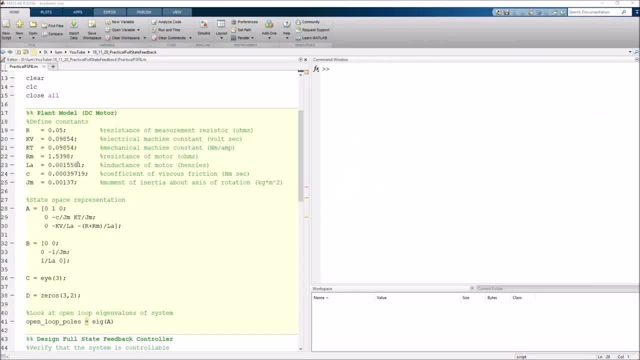 here and we'll head over to matlab. all right, so here we are in matlab and i've already actually picked up this script. just to avoid, uh, me and my fat fingers punching it in and making tons of mistakes and forcing you to watch all that, i thought i would enter it in ahead of time. 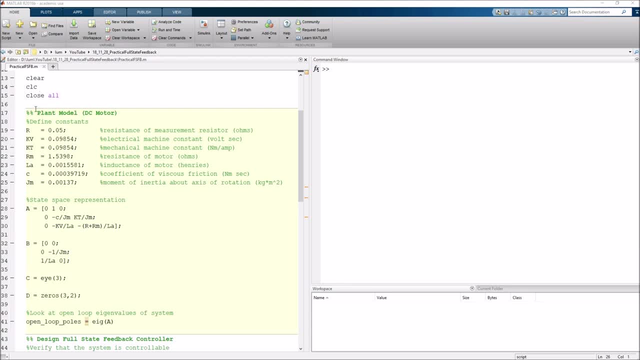 as you can see, it's pretty darn standard right. we got our normal clear clc, close all, and then the first thing i'm going to do here is just define that state space representation of the dc motor here. so here are just all of these constants here again. if you don't care about, 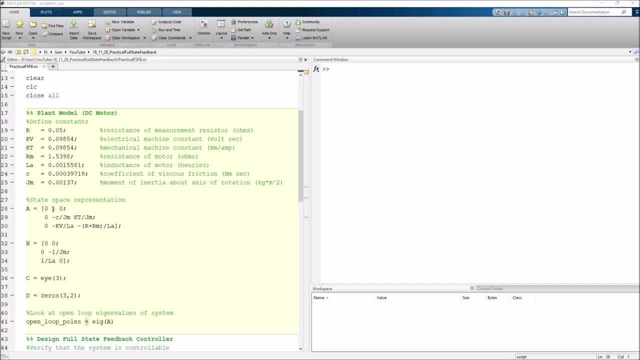 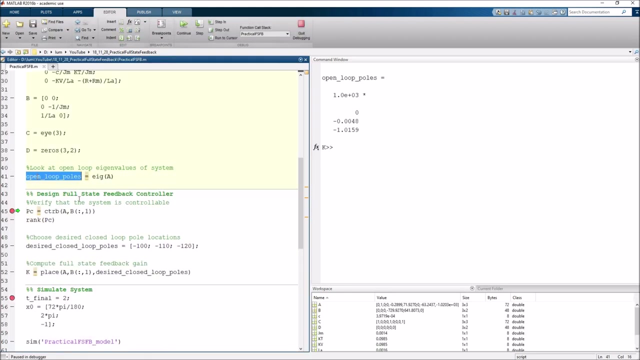 the actual physical meaning of the plant. you can just remember that it is a three state system here. so let's just go ahead and run this first chunk here up to calculating the open loop poles. and, as you can see right here, like we said earlier, you've got those poles here at zero minus 4.7 and minus. 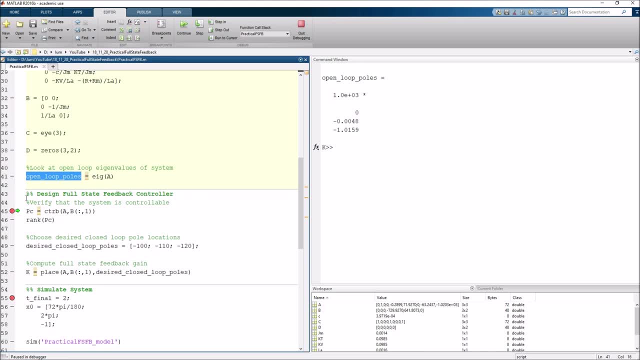 1015.9 here. okay, all right. so, coming back to the matlab script, we're going to run this first chunk. we see that the next thing we want to do, like we chatted about earlier, is just check to make sure that the system is controllable using only the first control input. so i only pass in the first. 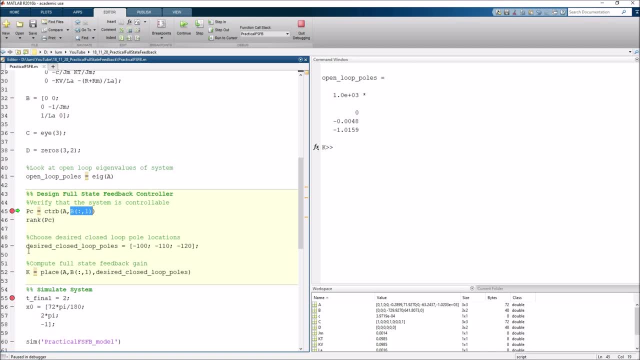 column of the b matrix here. then i'm going to check the rank here. so let's just go ahead and maybe just f10 that step and then we'll step and yep, look at that, the rank of this system is three. so the system is fully controllable. so i can now move the poles to any location that i want. so 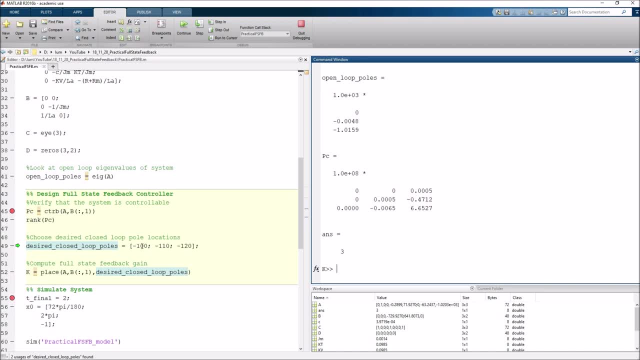 i'm just going to go ahead and list out the locations that i care about. so i want to move the closed loop eigenvalues to minus 110, oh sorry, minus 100, minus 110, minus 120. then i should be able to call place again. i'm going to pass it a. 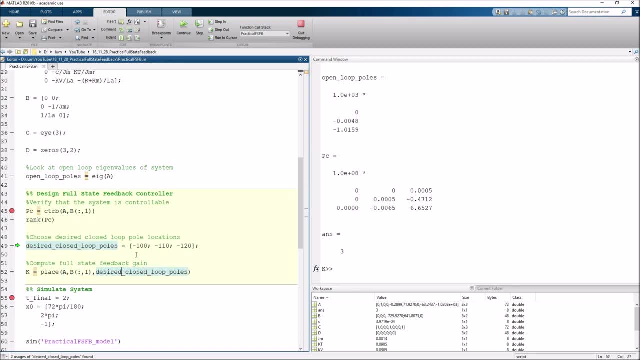 and then the first column of the b matrix here, and then my list of desired pole locations here. so go ahead and step, step and here's the uh full state feedback matrix that's going to make this happen for me. it's uh, yeah k of 28.6, 0.68 and minus 1.07. 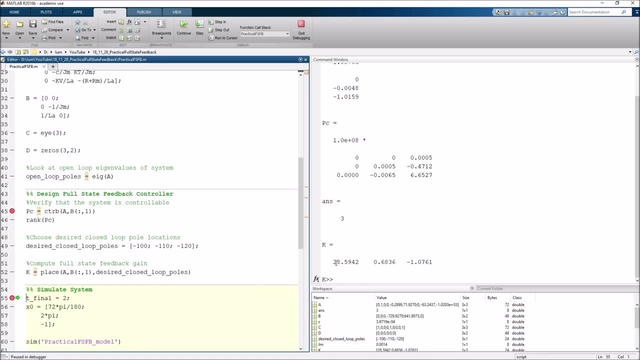 uh, eight ish, something like that- great. so now that i've got this, this um controller computed here, why don't we go ahead and simulate the system to make sure that that works? so what i'm doing right here is i'm just setting up some simulation parameters, like how long i want to simulate for. 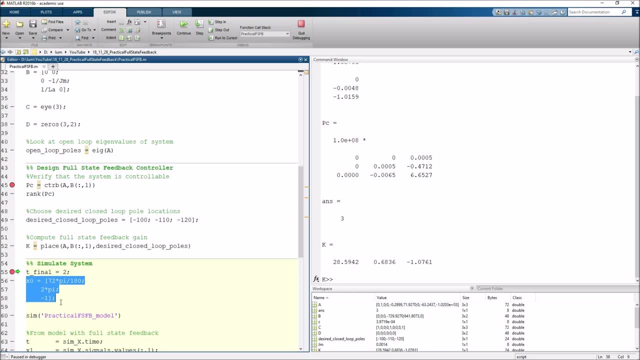 and then i'm going to use some non-zero initial condition and i want to make sure that the full state feedback controller will regulate this system back to the origin here, so the initial deflection of the wheel here in terms of angular position. so it's, it's cocked up and then i'm going. 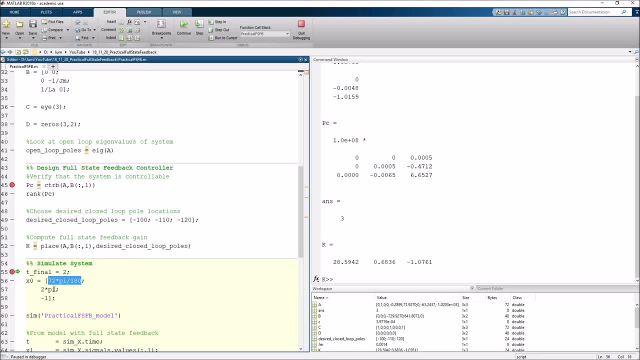 over at 72 degrees, it has two pi radians per second and it has minus one amps flowing through it at time zero. so here's my initial condition, and then i'm just going to simulate a simulink model here called practical full state feedback model. let's just go ahead and open this so we can. 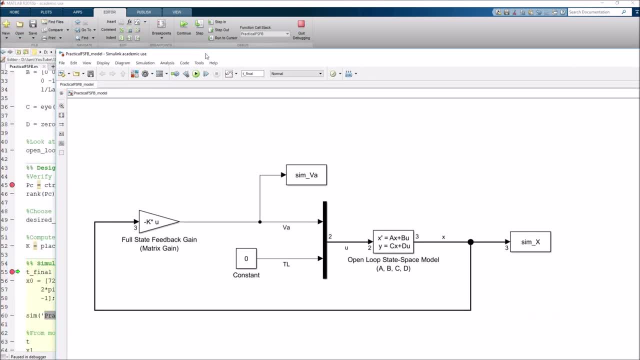 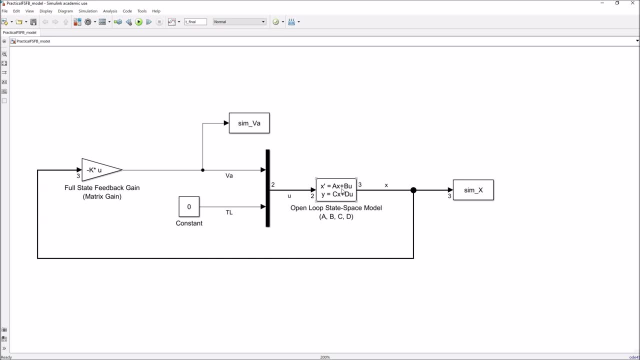 get a look at what that uh looks like. and again, just so you don't have to watch me cobbling blocks together: i've built this already ahead of time. again, here's my plant model. as you can kind of see nothing special here, you know, you've got your. 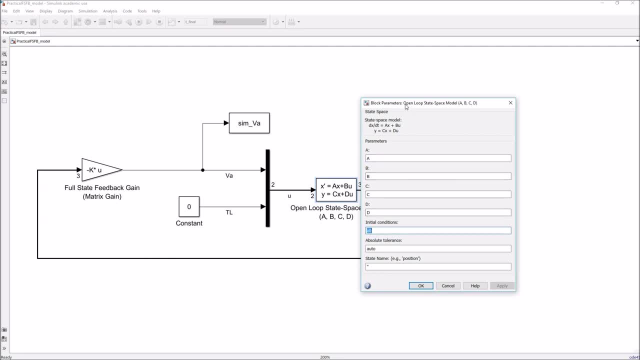 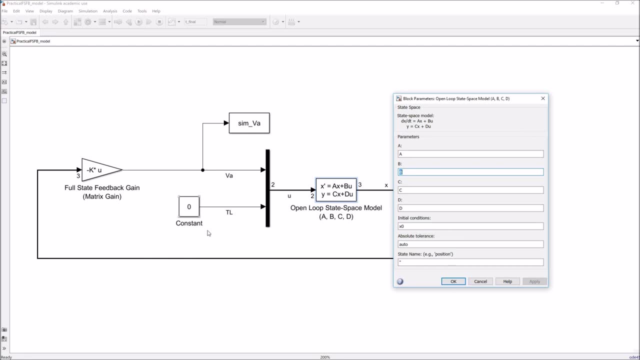 a, b, c, d and my initial conditions here. the only thing to note here is maybe i'm passing in the full b matrix. so again, this system has two inputs, but as you can see, here we're just putting the external torque load, or that second input, to zero, because all i want to do here is control the. 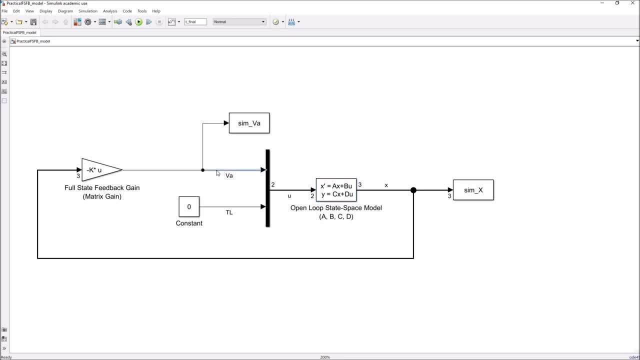 system using just the armature voltage here or the first input, right. so that's what my full state feedback gain or my controller is doing here. the only thing that maybe called your attention here- that might be a little bit hidden here- is the amount of torque that i'm going to be getting. 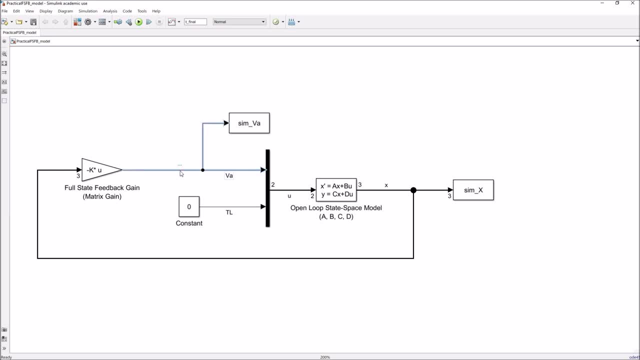 as you know here the control law here is va should be equal to minus k times x. but this is a matrix multiplication or a matrix gain here. so what i actually had to do here is in this matrix here or in this gain block here is i actually had to come here to multiplication. normally it's set to. 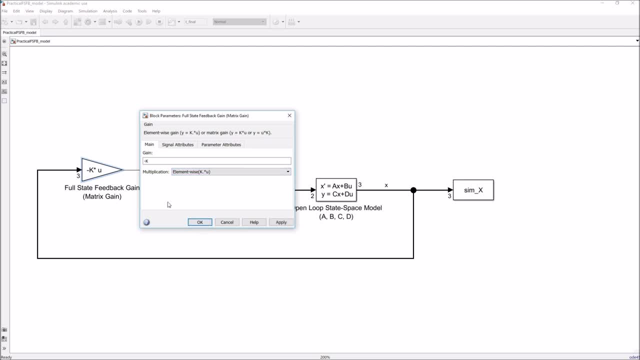 element wise by default. most simulink versions are going to have it: element wise multiplication when you drop this in. that is not what you want to do in this case, right? we don't want element wise multiplication, so i need to change this to matrix multiply and, furthermore, i need to 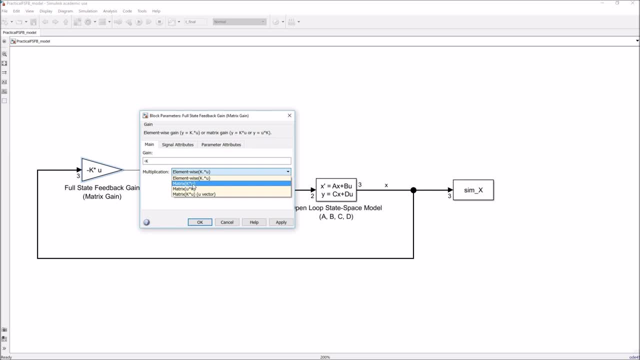 matrix multiply k, with the vector being, uh, multiplied on the right. you can see you can do it opposite here. right, you could actually have the vector multiplied on the left here. so this is the appropriate operation that i want. so i need to make sure that i select it, hit apply and okay. 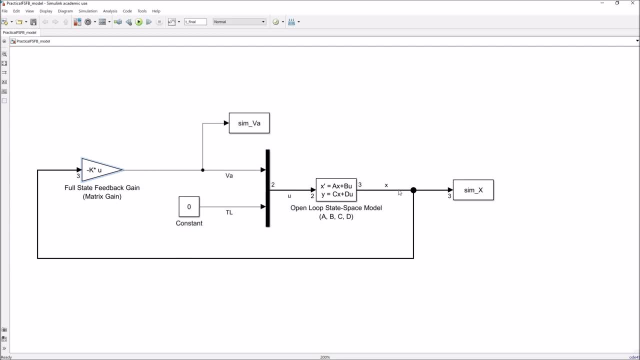 great, and then the only other things that maybe called your attention here is: then let's send the state of the system back to the matlab. uh, workspace using a to workspace block. i've got this variable called sim x and i just changed the save format to structure with time. i like this better than time series. it's just something i'm. 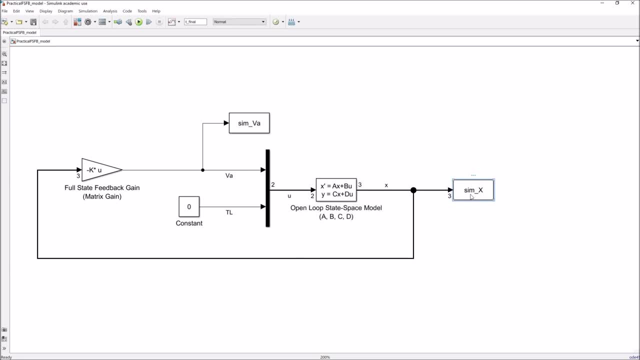 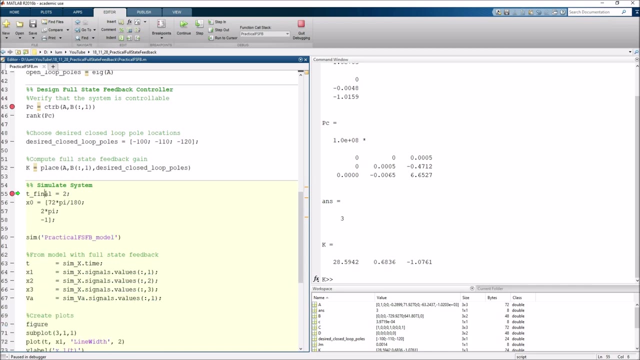 more familiar with here. so let's save both the state and we will save the control signal um and see what we end up with here. so this is what the simulate model looks like. so i think we can go ahead and close that. and now let's just go ahead and step through this a little bit more here. so i 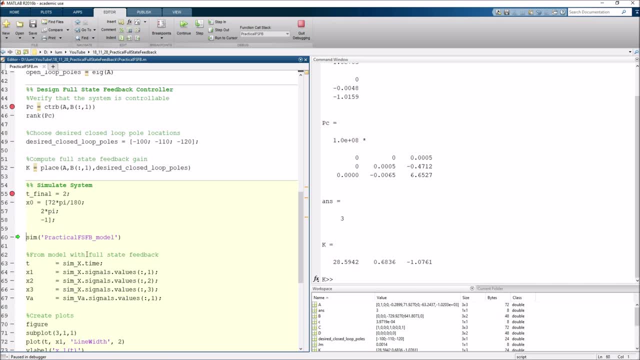 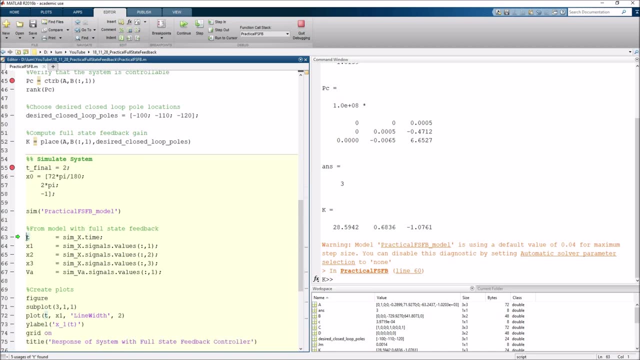 will set up my parameters here now, on line 60. let's just go ahead and run the simulation and whabam, it's, it's done. um, and now what i'm going to do is let's just extract the time, the three states and the control signal, and 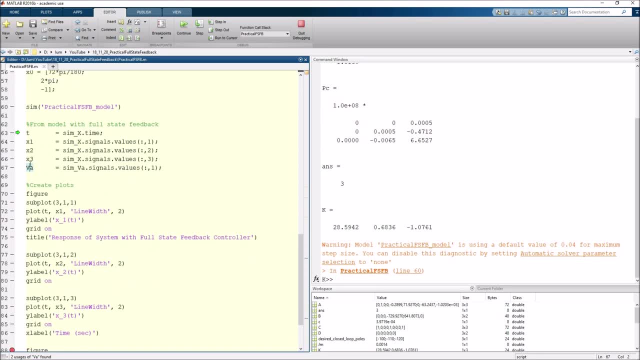 see what we end up with here. so i've just got a bunch of plotting right here. so maybe let's just f5 here and, uh, what i'll do is i'll plot the three states um, and we'll see how this controller performed in this scenario. so let me hit f5 to just jump down there, and here's the plot that we. 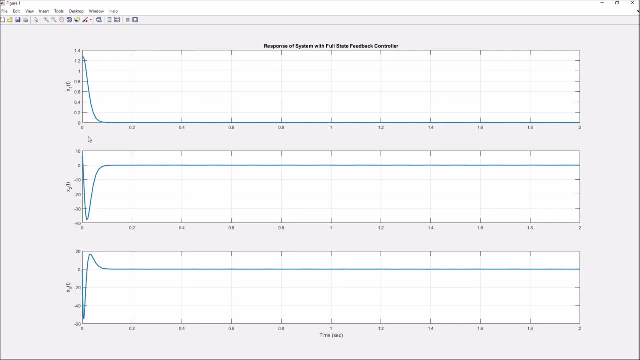 and look at this. this is beautiful, right? if you look at this upon, uh, a cursory inspection, you see, yeah, we've got non-zero initial conditions here. but look at this: whabam the controller slammed this system back to the origin in less than a tenth of a second here, right, look at this. 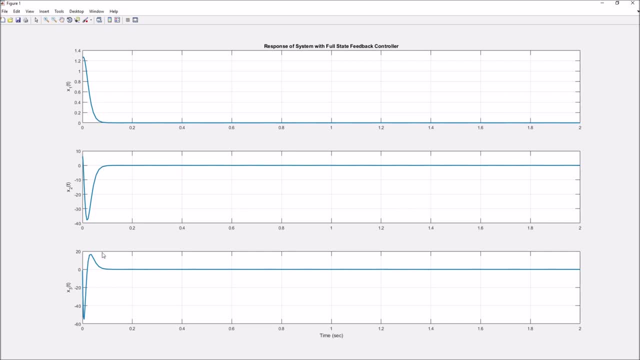 the thing went from 72 degrees and just snapped back here to the origin in you know a tenth of a second. so performance is awesome. and i would say, yes, i'm going to go ahead and run this simulation in less than a tenth of a second. and i would say, yes, i'm going to go ahead and run this simulation. 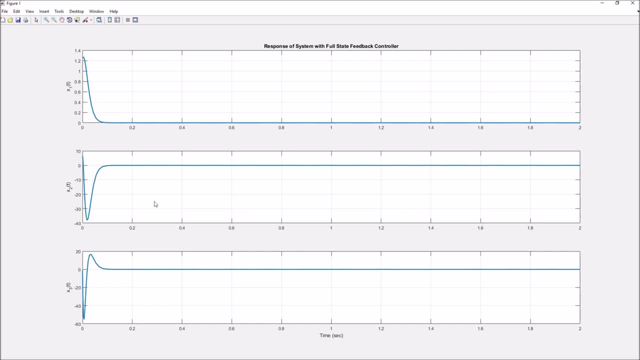 Yes, the system definitely is behaving like it has closed loopholes at minus 100,, minus 110, and minus 120,. right, It's snappy. There's no oscillation, And this you know. if you showed this to your boss, I think they would be really really happy here, right. 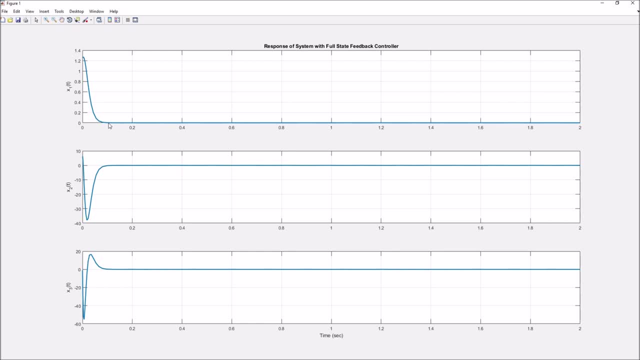 Now, you know, I had a professor who his favorite saying was there's no free lunch, right? We should ask ourselves what's the price we paid to get this phenomenal performance right, And the thing that we can do to answer that question is we should look at the other half of the story, right? 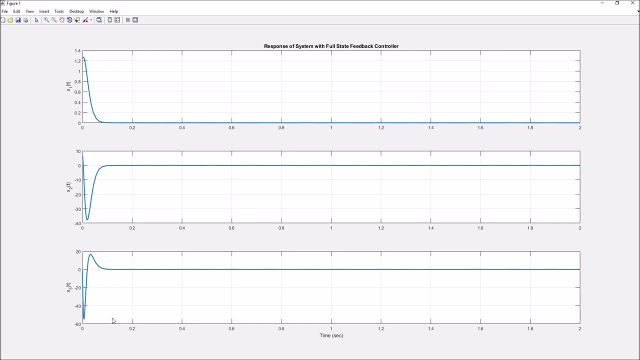 Just looking at the trajectory of the states is not enough. We really should look at the trajectory of the control signal. What did the controller do to the system in order to get this result? So, coming back to MATLAB, that's what this second plot I'm going to make here. 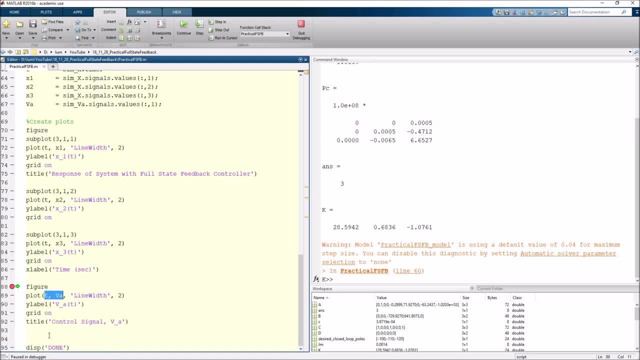 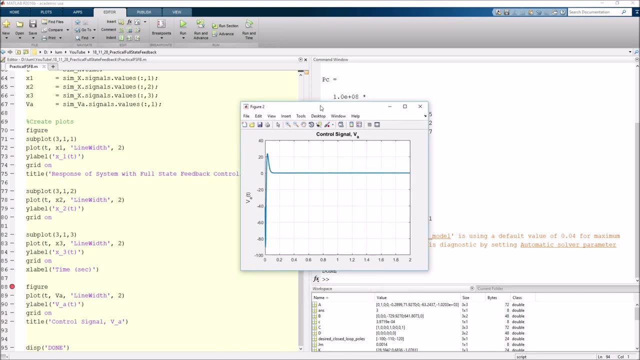 If you notice, here now I'm just going to plot the control signal and we'll see what it looks like. So again, let me hit F5 here and I'll pull this over. And here's what happened. So we should stop and think about: what does this plot mean here, right? 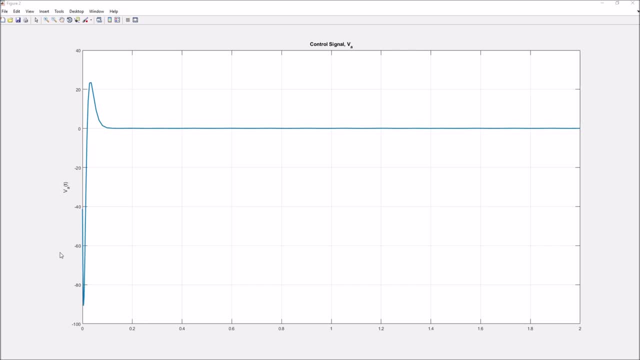 This is the control signal. It's the voltage that we are applying to the motor here in units of volts. So you can see that what happened was, yeah, we got awesome performance, but the controller was asking for and applying something like negative 90 volts to the motor here. right, 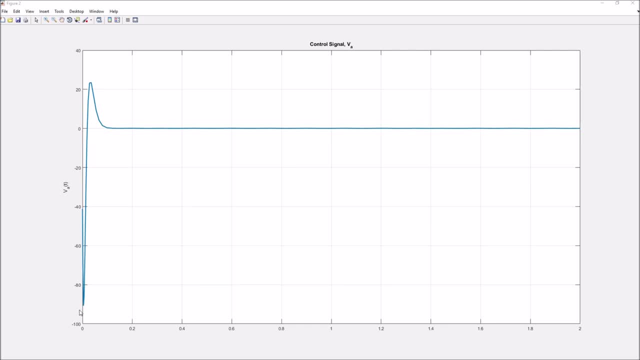 Which in many real-life scenarios with these small little motors, maybe we can't get that, Maybe this is infeasible, Maybe your benchtop power supply can only supply, you know, plus or minus 20 volts. So you see, in this case, mathematically we were able to get that kind of performance. 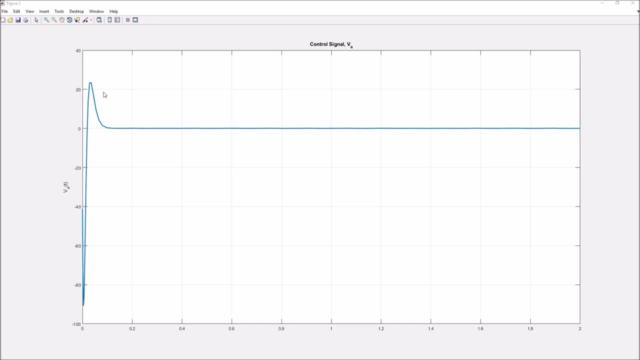 but it requires an enormous control signal to do that here. So in a lot of real-world scenarios you might saturate your controller and your actuator is just not going to have the control authority to enforce this type of drastic change to get you that awesome performance we saw earlier. 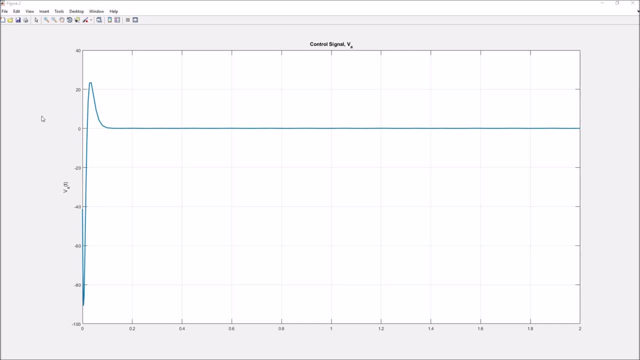 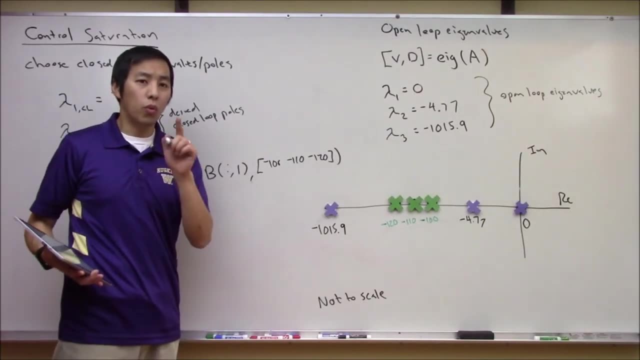 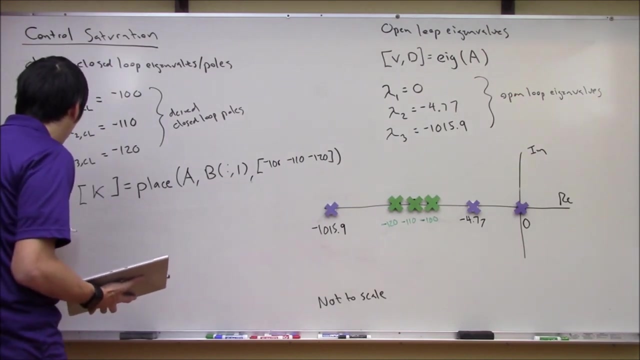 So we should maybe go back to the whiteboard and think about: is there a way we can ameliorate this situation? Okay, so we saw that what ended up happening is we had this control saturation issue. So maybe what we should do is let's start a little table here of maybe my desired poles. 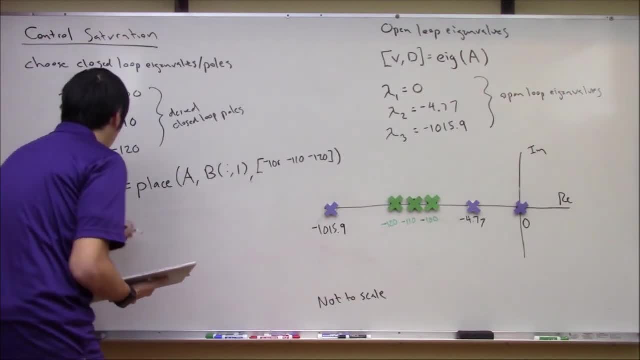 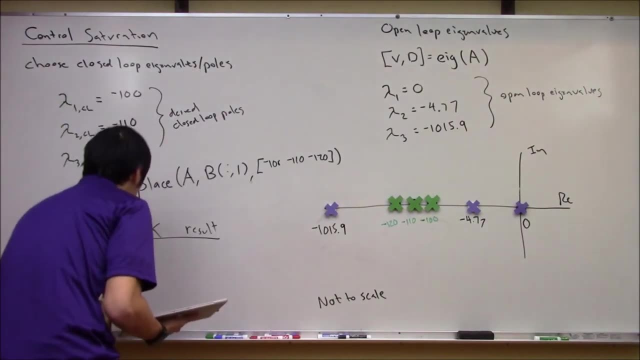 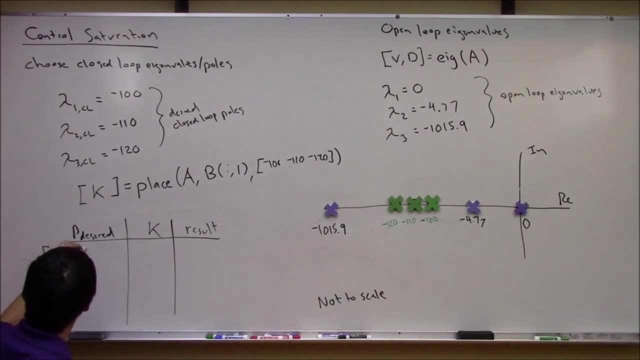 like. so P desired right, And let's talk about what the resulting K was and what was the result, okay? Okay, so let's make a little table here to start. And we saw here that if we used desired poles of what was it minus 100,, minus 110, and then minus 120, right? 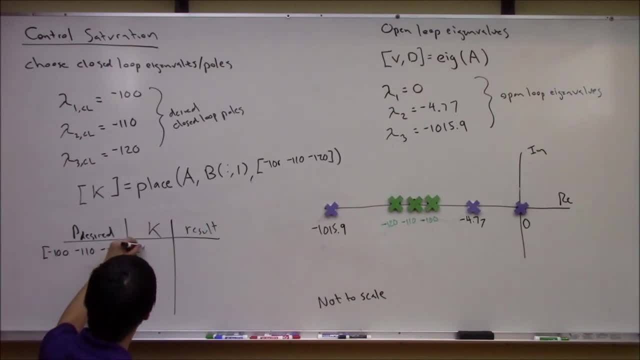 We ended up with a gain K here of it was about something like 28.. Maybe I should have made this a little bit bigger here. Let's make this a little bigger so we have some space. Okay, something like 28,, 0.7, and minus 1.1.. 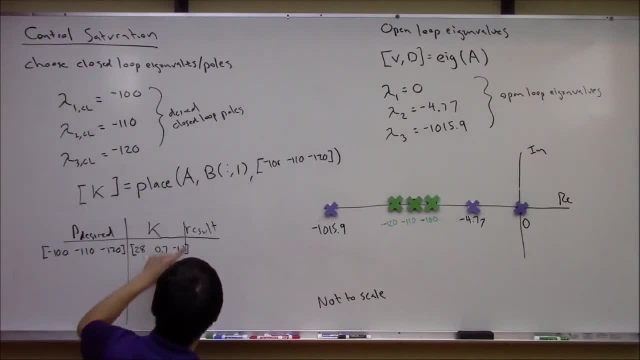 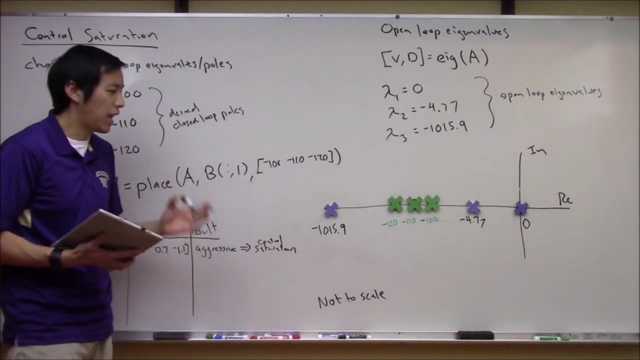 That was our, Our gain K here, And we saw that what this ended up being here was. this was a little bit aggressive right, Which led to control saturation Right, And again I think you can sort of see where this came from. 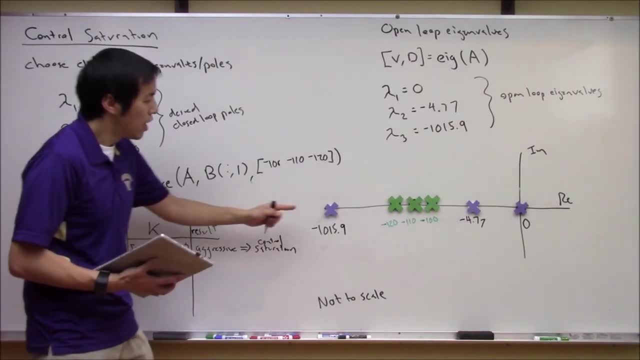 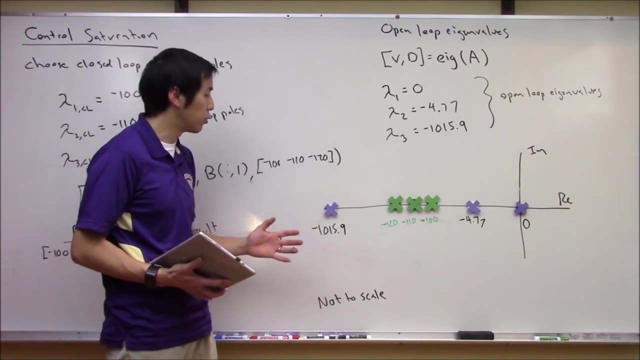 The reason this thing was so aggressive here is because, effectively, what we were asking, What we were asking here is we wanted to drastically change the plant here with our closed-loop controller here. right, If you think about this, right, the blue Xs, right. 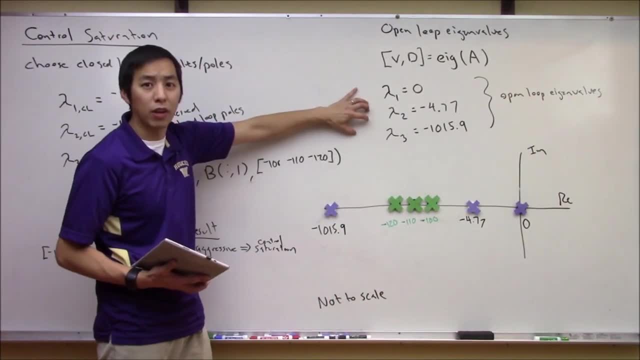 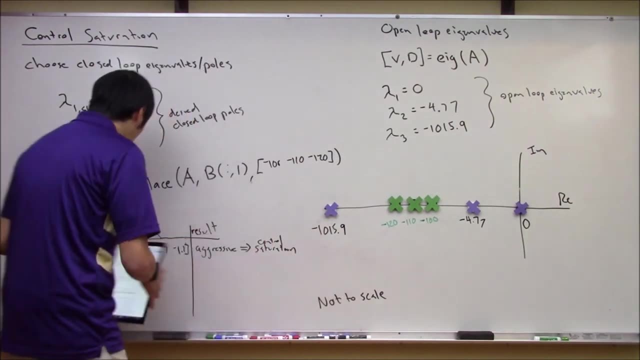 We talked about the blue Xs earlier. Those were our open-loop eigenvalues or our open-loop poles. That's sort of how the system wants to behave in its natural state here, And what we ended up doing here is we said: No, I really don't like the way you behave, or I don't like how you naturally are. 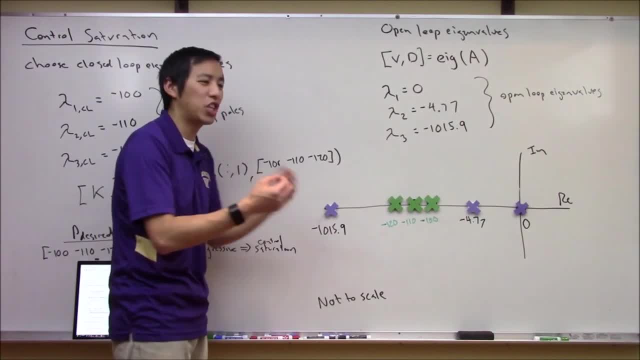 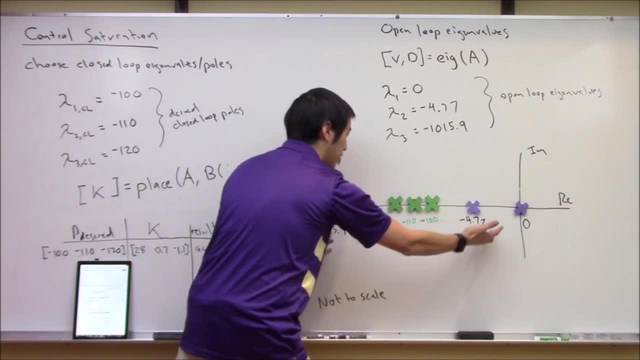 I don't like you as a person here. right, I want to change you. So this is like drastically trying to change the system to instead of behave like the blue Xs, I want you to behave and be a better version of yourself. 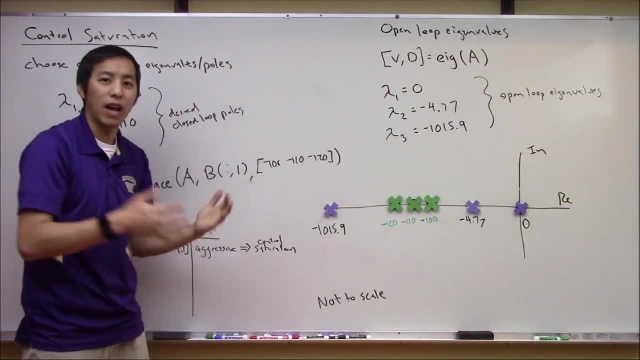 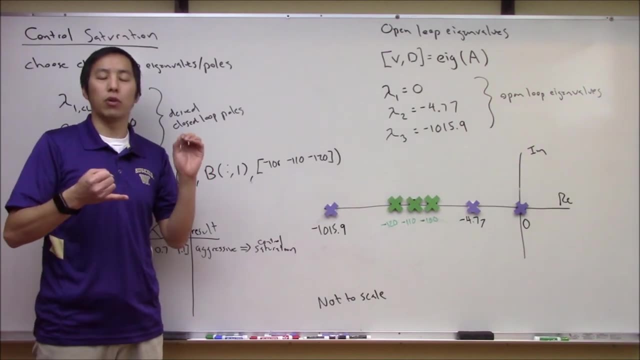 I want you to be these green Xs right at these different locations, And that was a drastic change. That's like you know, if I went up to my dog and I said You know what? I don't want you. I want you to stop eating off of the table. 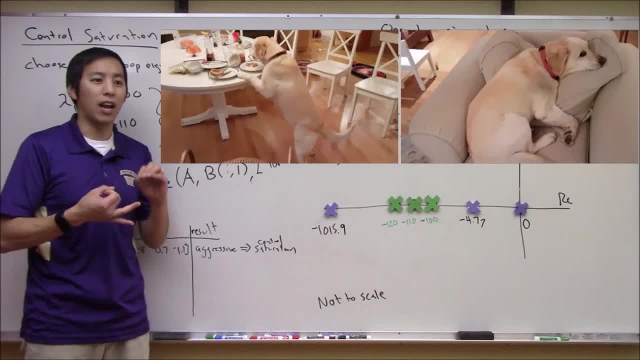 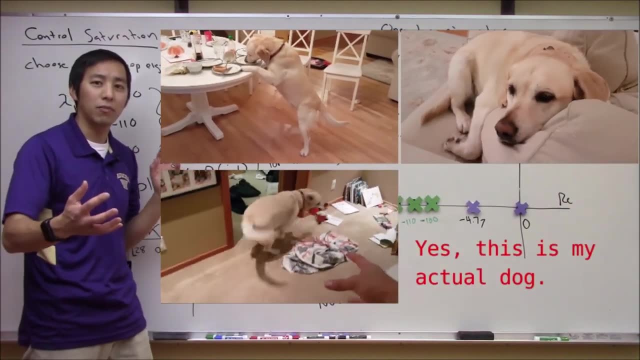 I want you to stop sleeping on the furniture and I wish you would really stop stealing all of the kids' toys here. right, But that's what he likes to do. That's his natural state. If I wanted him to change all of that behavior simultaneously, it would take a lot of control authority here, right. 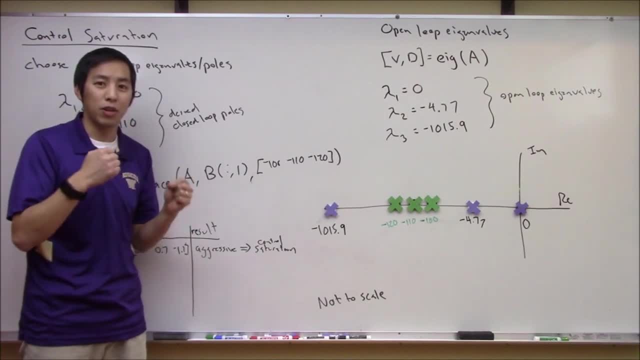 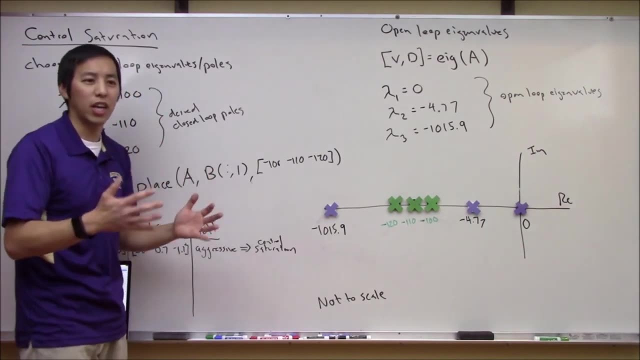 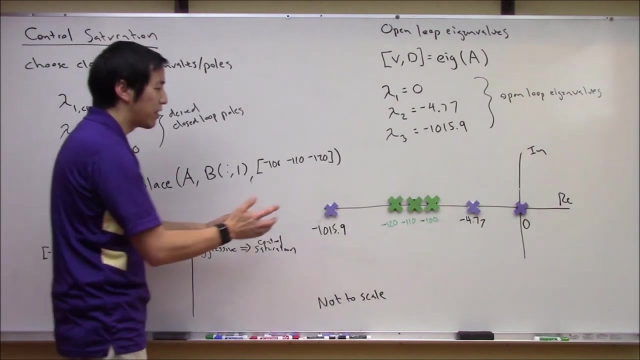 I would have to beg bribe cajole, you know, yell at him. I would have to exert a ton of control authority in order to change his behavior right Or to change how he behaves right. So, following that line of reasoning, maybe one approach here is: let's not ask the plant to change so drastically. 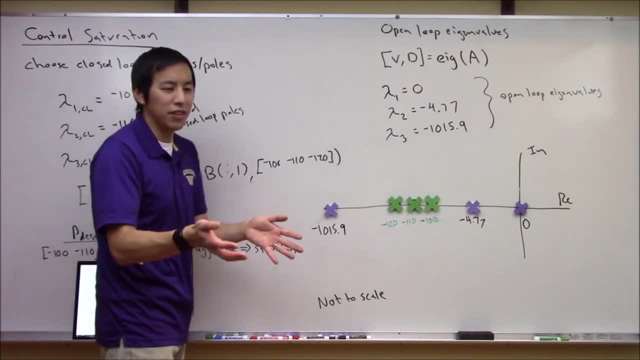 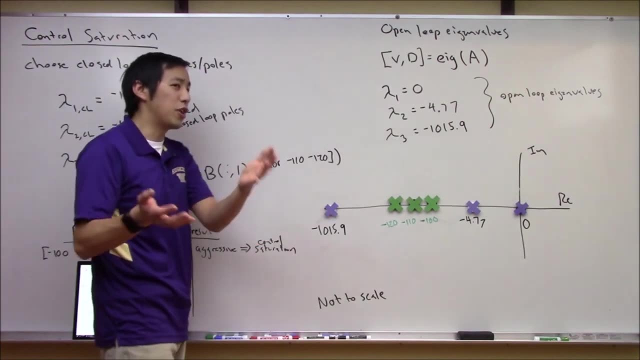 Maybe we'll say, yeah, it's all right if you still eat off the table, just don't do it so often, right? And you can still sleep on the nice living room furniture, but don't do it when you're wet here, right. 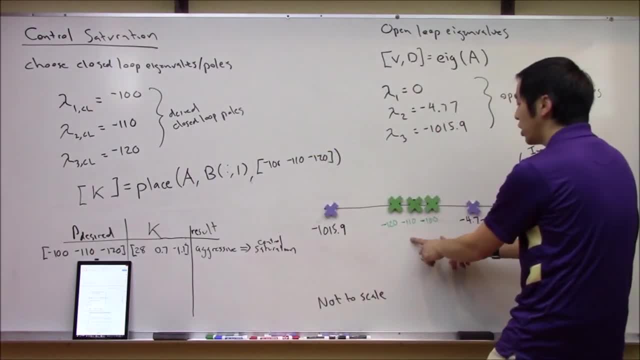 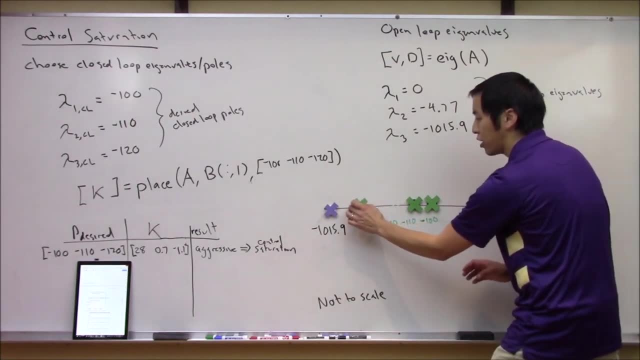 So what we're basically getting at is, another approach here would be to maybe don't make such a drastic change. So let's take this and move it a little bit back closer to the original location, right, And let's do that for all of these poles here. 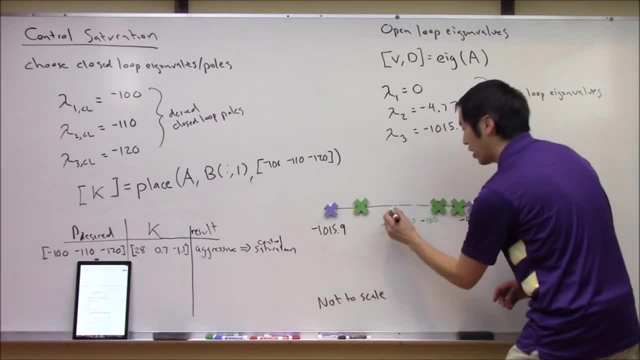 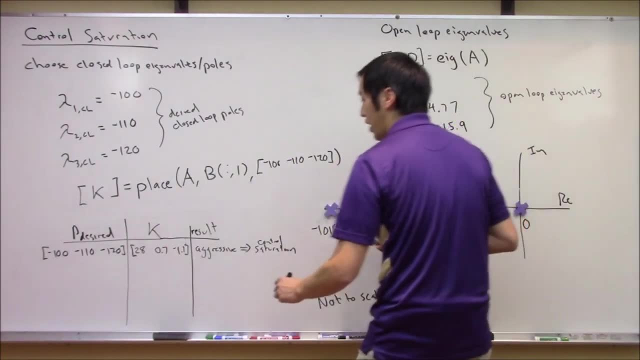 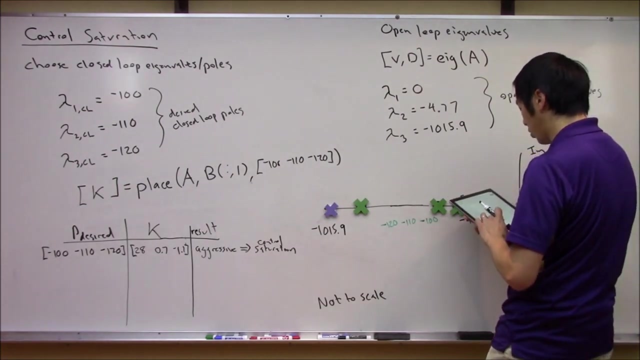 So these ones as well, Let's move them a little bit, something like that, okay, So what I'm suggesting is let's go with approach number two here. So the second way here is to basically choose slightly less aggressive changes here. So in this example- I don't know- let's choose something else. 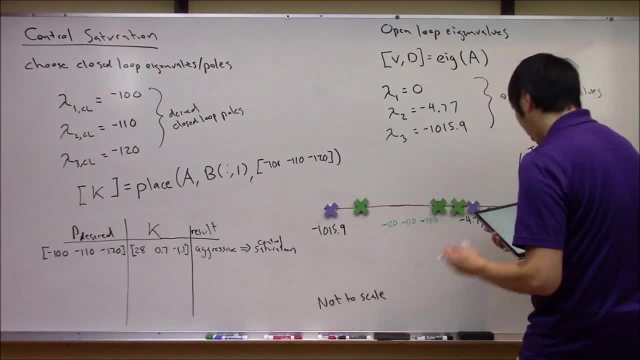 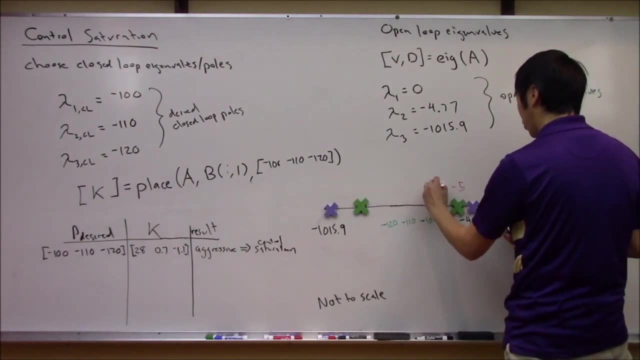 Maybe I'll do it in a different color here so we can keep them apart here. So this approach here is: maybe let's make this here at I don't know how- about minus 5,, minus 30, and minus 400 here, right? 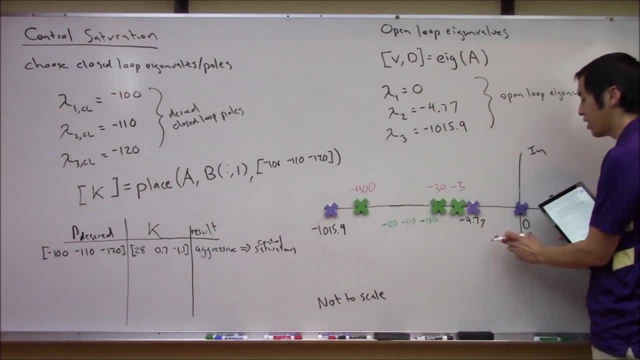 Okay, So this is a less aggressive change. I'm not asking the plant right- the blue Xs- to move that far from where they were originally right. So this is like asking for a small change. So the process is virtually identical, right? 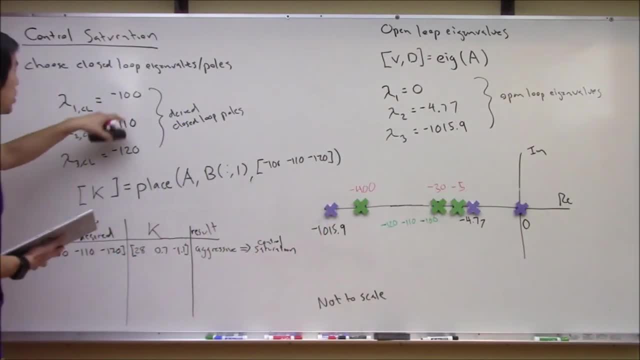 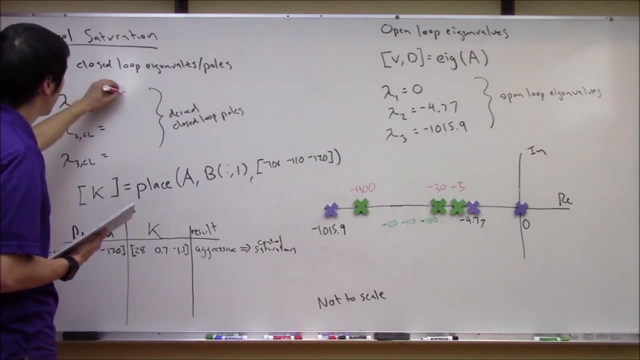 Only thing that changes here is that I just need to change these right. So instead of making this drastic change, let's make it a little bit less violent here, So like minus 5,, minus 30, and then minus 400,, right? 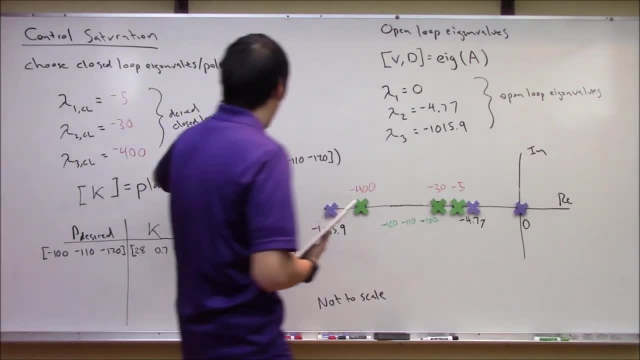 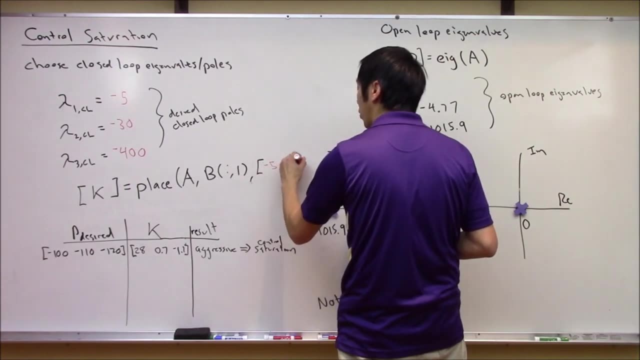 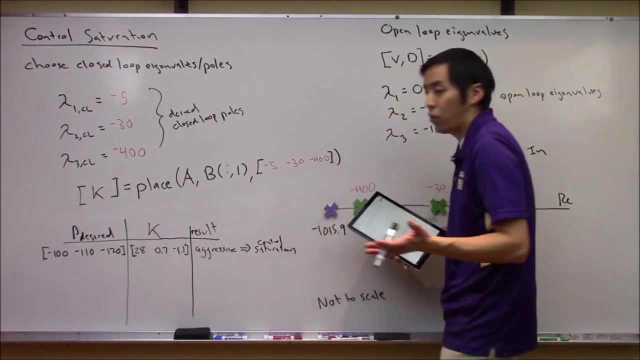 And then I just Let's run this exact same thing again, right, I run the exact code again, but just with different closed loop desired pulls, right? So minus 5,, minus 30, and minus 400,, okay, And if you run that again here, what we end up with is well, you know what. 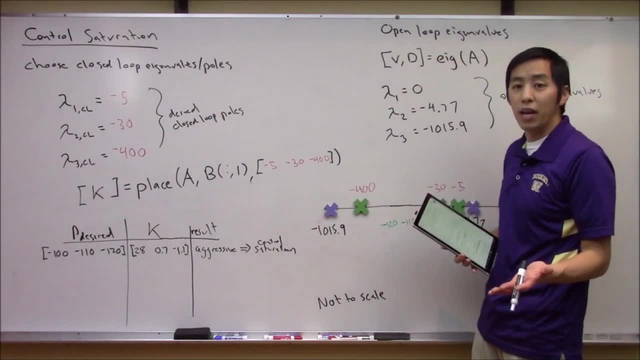 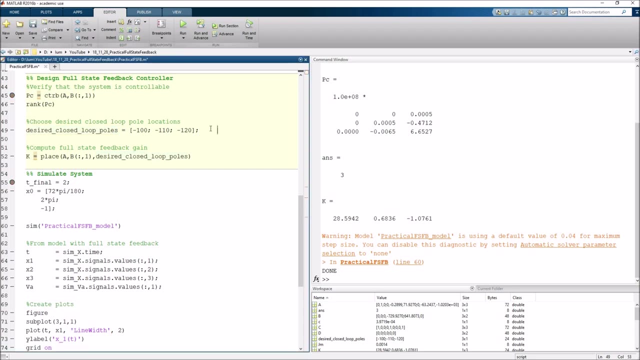 Tell you what. Why don't we run over to MATLAB and see what ends up happening and what the resultant behavior of the controller is? All right, We're back to that same MATLAB script. So we saw earlier that, like we said earlier, this choice. 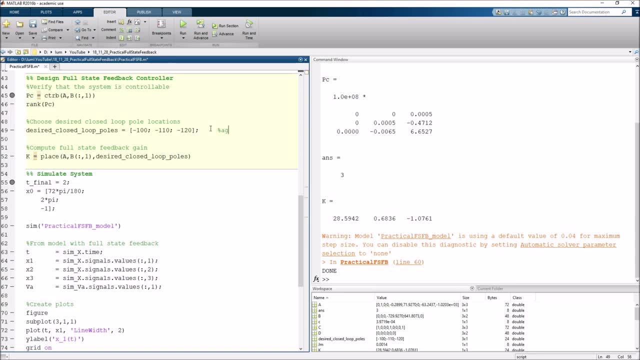 Choice of selection of desired closed loop pulls. This led to an aggressive controller, right? So what I want to do now is: let's actually comment this out and choose slightly less aggressive locations here, right? So what did we suggest here? I think it was minus 5,, minus 30, and minus 400 here, right? 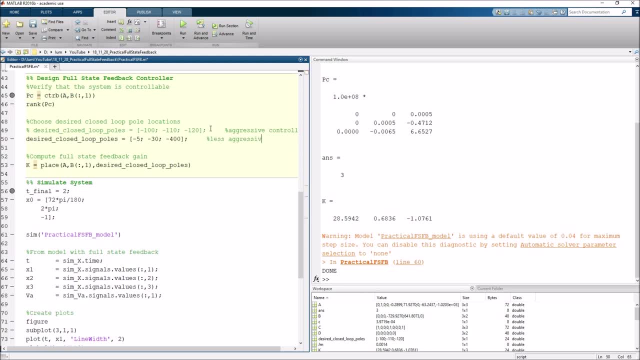 So this is hopefully a less aggressive controller. right And now. what we can do is we can rerun this entire script here And all it's going to do is just give us a new full state feedback controller, And then we can simulate it for the exact same initial conditions and see what happens here. 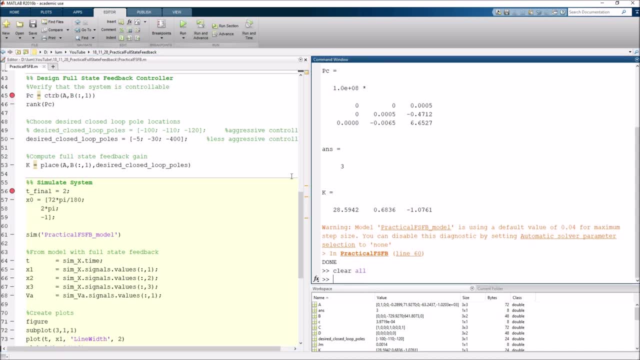 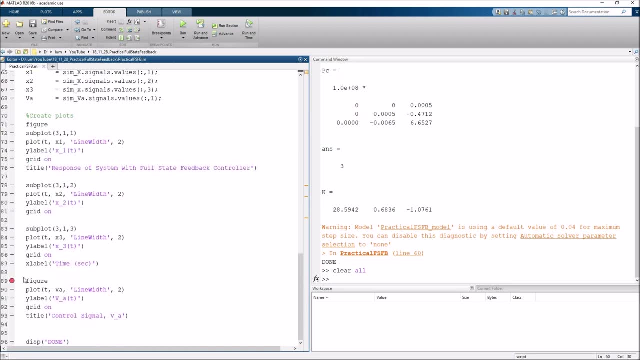 So tell you what? Let's clear all the breakpoints here from the script. Let me just take them off here. Let me see, Take off all those breakpoints. Great, Okay, I think we got the breakpoints out of here And let's just go ahead and run this thing again. 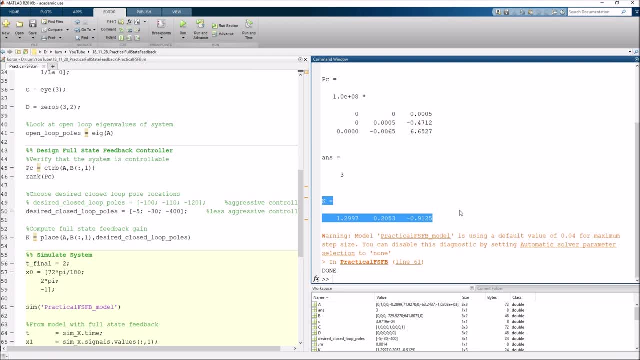 Okay, So here's our new controller K here. You'll notice here that the magnitude of the numbers are a little bit small, or actually quite a bit smaller than we had before, So this should be a less aggressive controller. So let's take a look at the result here. 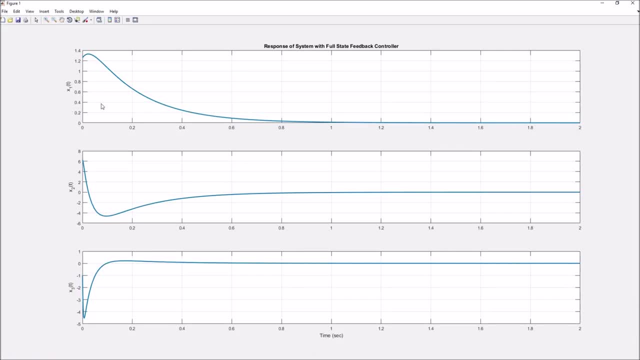 So here's the result of the state trajectory And you see, yes, it's definitely less aggressive. Instead of taking 0.1 seconds to come back to the origin here, you can see it's almost an order of magnitude more, So it almost takes like a full second to come back to the origin. 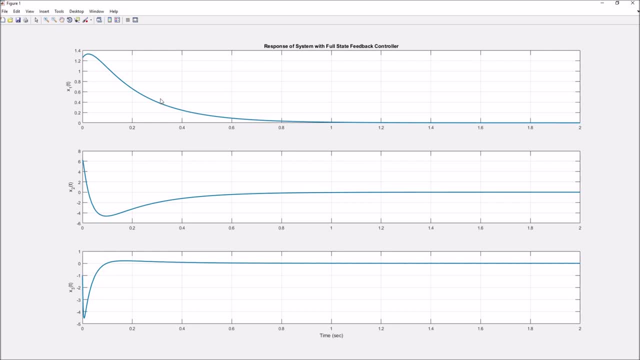 It still does it in a nice fashion, right? There's no overshoot. Everything comes back smoothly here And now. if we look at the control signal, this is where we're going to make some wins here, right? So if I now look at the control signal here, ah, this is much nicer here, right. 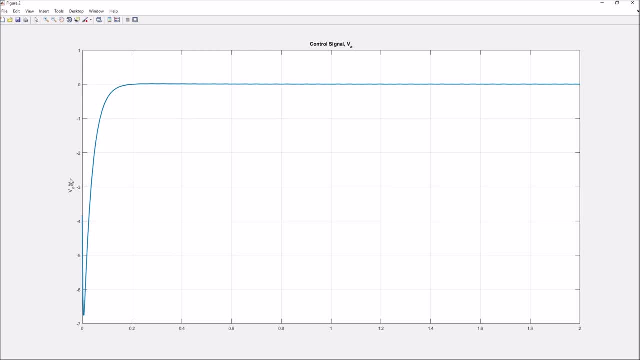 Instead of 90 volts here of control authority to get that behavior. we're now only here at, you know, less than 7, less than a magnitude of 7 volts, Which I'm pretty sure you're not going to saturate your controller at this stage. 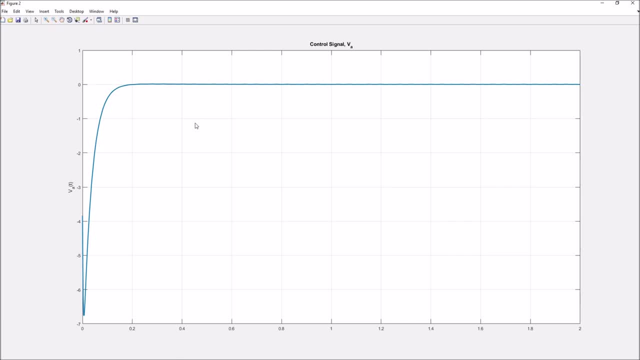 So you can see here that this is one way that we can go about uh uh, dealing with this control saturation issue here, right? However, even though we solve the control saturation issue, there's other, uh, practical implementation problems that we might want to think about. 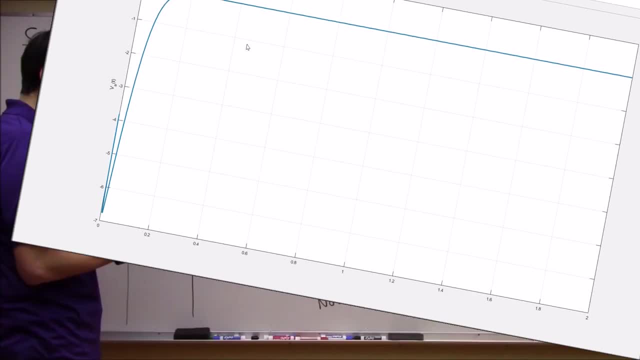 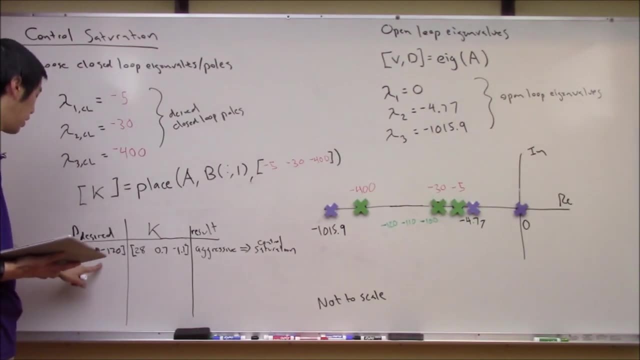 So let's go back to the whiteboard and examine what those are and how we can fix them. Okay, So before we're actually we taught we we leave the control saturation issue. Maybe what we should do is: let's finish up our table right here. 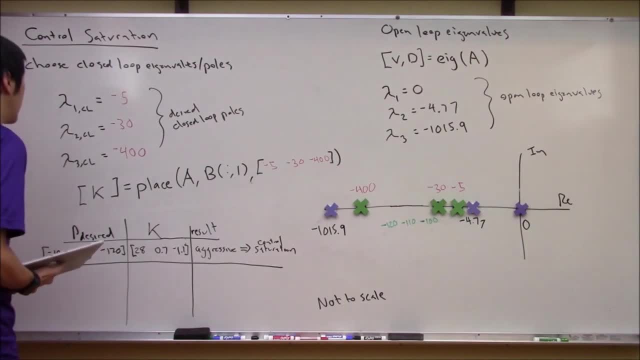 So we saw that We just had a different set of um of desired locations here, right, So, at minus 5, minus 30 and minus 400, right. What we ended up here was with a K that was something like on the order of 1.3, 0.2 and minus 0.9 here, right. 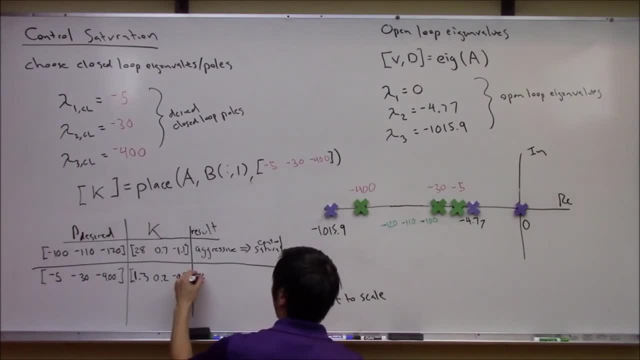 And we saw that, just looking at the numbers, you can see that this is a less aggressive controller, right, And this basically solved the issue. A control saturation. So I think we could say there was no control saturation here, right, Okay? 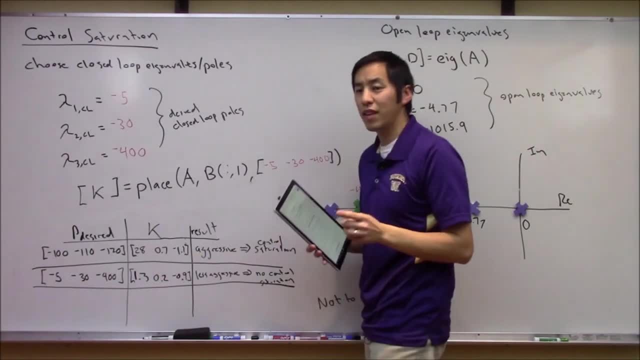 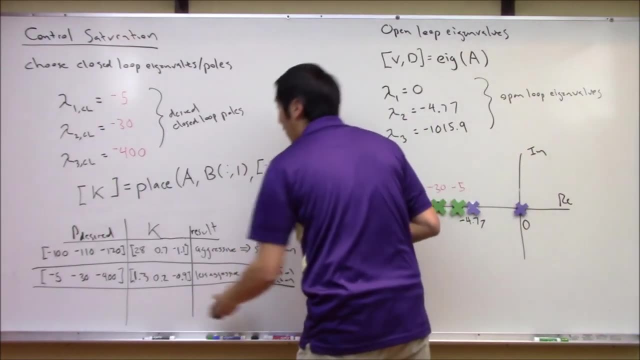 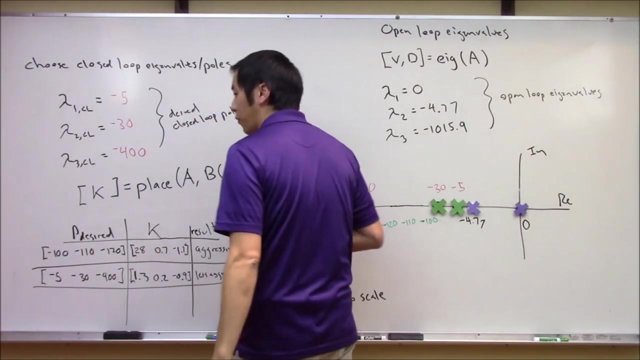 So that's great. Let's leave our table here, And I want to now investigate one of the other issues here that we might uh end up with when we're trying to implement a full state feedback controller, And in fact, this is one of probably the major issues or uh drawbacks that make a full state feedback controller impractical in a lot of real world scenarios here. 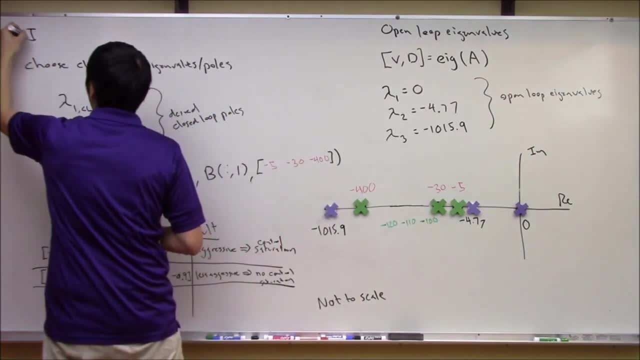 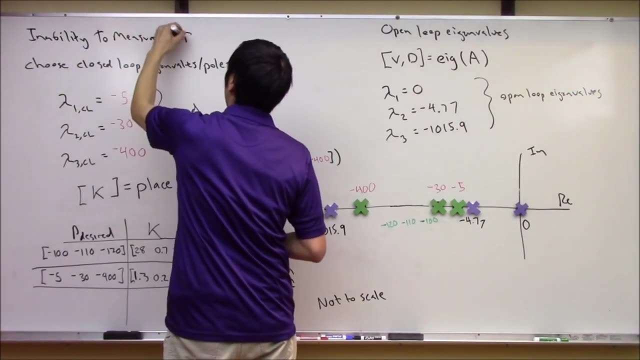 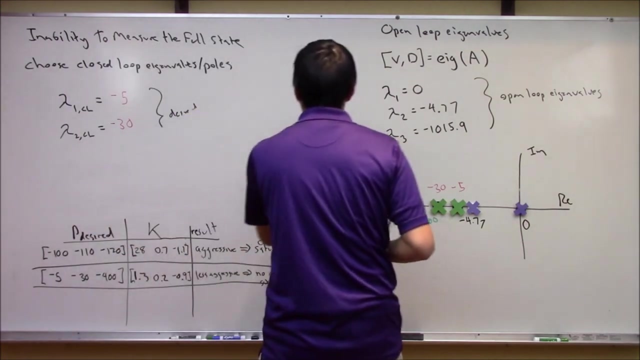 So the problem here is is basically the inability to measure the full state right. So, in other words, let's erase some of this. We can get a little bit of space here. The problem here is, um, the control law right. 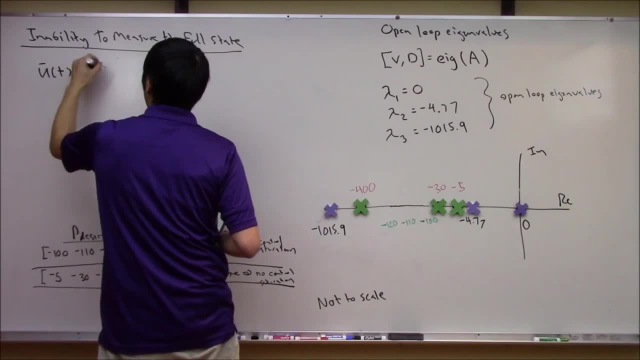 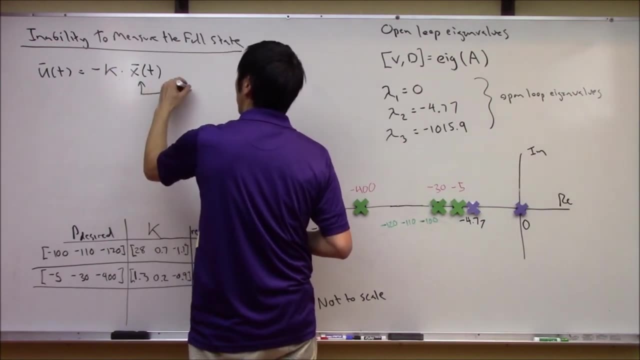 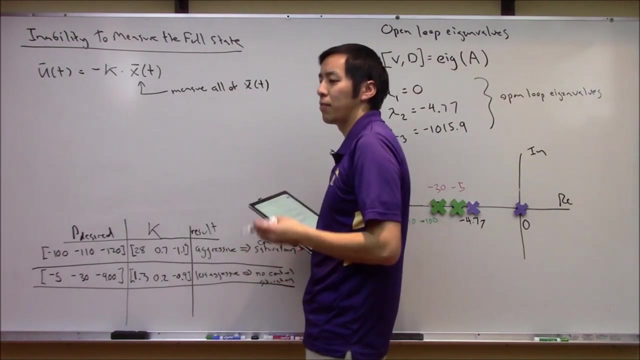 If you remember, is U is minus K times X, Right? So in order to implement, this requires here that you measure all of X. So you need to buy a sensor to measure every single control or every single state in your system. here This can get complicated if, if your system has, uh, you know, a reasonable number of controls. 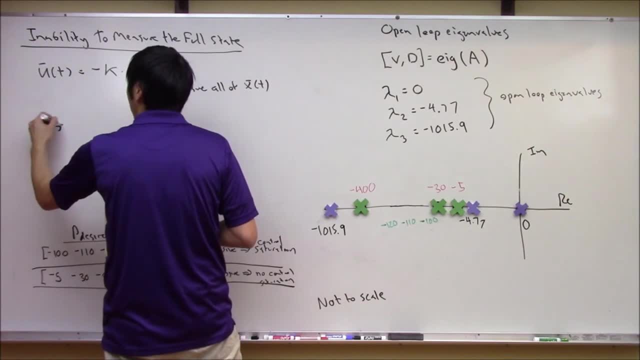 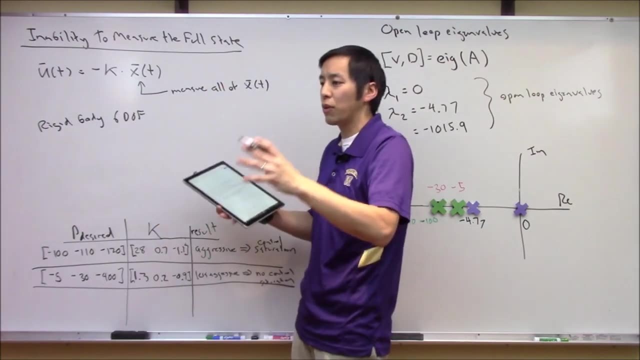 So, for example, if you consider just a, you know, a rigid body um six degree of freedom model for just you know it could be an aircraft Right, Or a brick, or just some rigid body translating in space. here let's use an aircraft example. 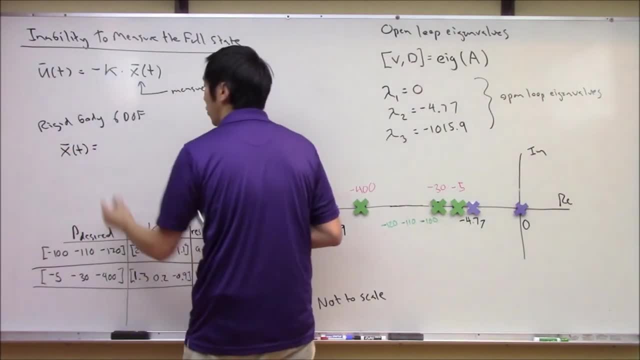 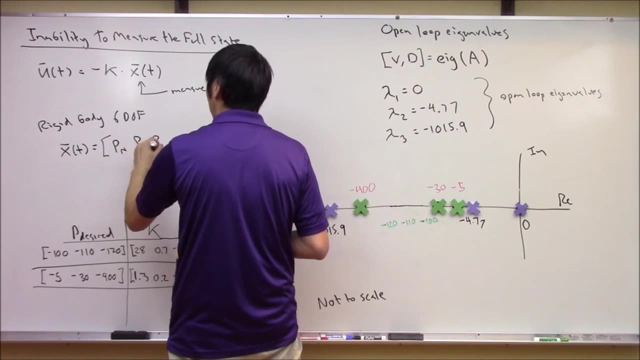 I think that's easiest to deal with here. Right The state vector, you can show that this thing is um. you need to know the position here in space. So like a position north, a position east, a position down, you need to know the velocity in space. 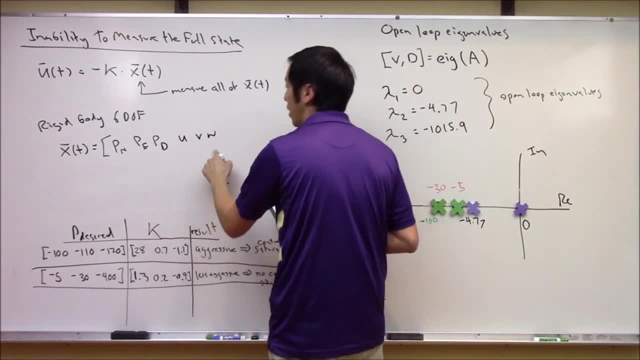 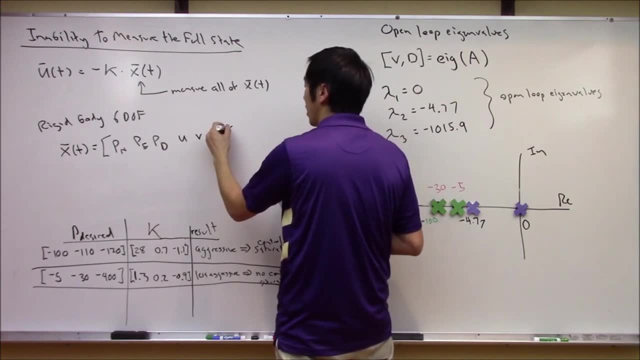 So, like a UVW, these are. these are velocities in the body frame. You also need to know the angles here, since this thing can can translate as well as rotate. So I need to know three angular positions, like like um. 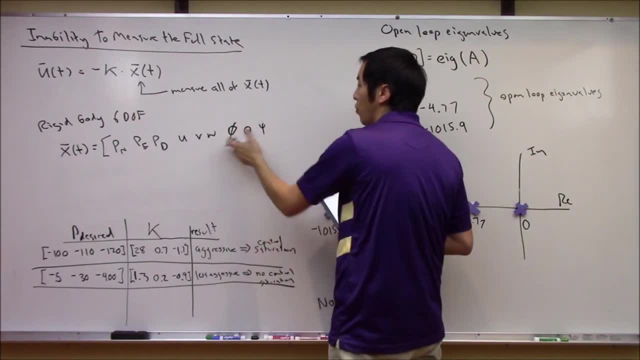 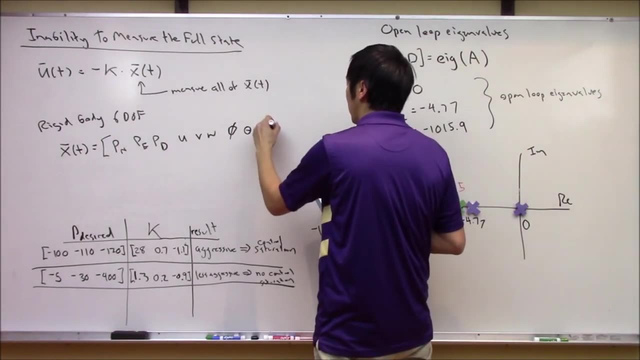 Phi, Theta and Psi, maybe three Euler angles, And then I need to know their rate of change, or some, uh, some idea of how this body's rotational velocity is is evolving, So maybe let's call this P, Q and R here. 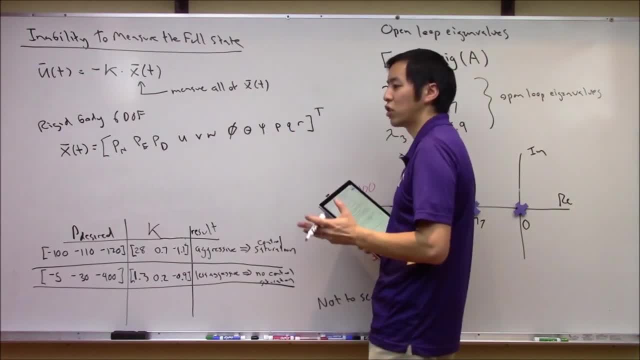 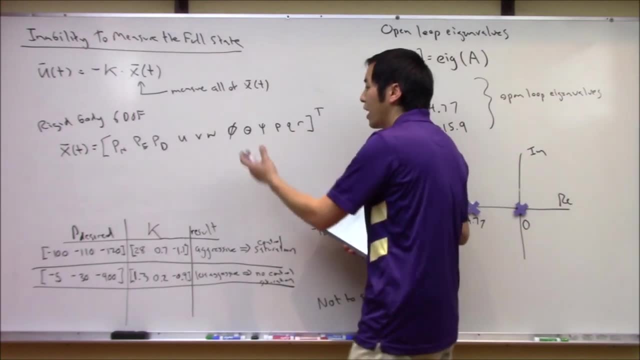 So this might be a state vector here for just just a very pretty much the simplest model of an aircraft that you can make. It's just a rigid brick flying through the air, And already this now has 12 states here, Right. 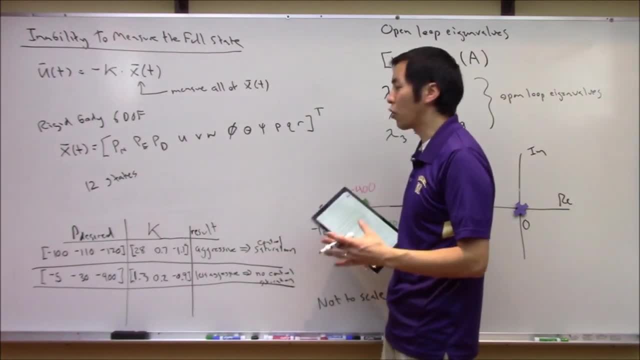 So if you wanted to implement a full state vector, you could do that Right. But if you wanted to implement a full state feedback controller on your aircraft, you need to measure all of these things here, Right? So I need like GPS, you know, to get the position. 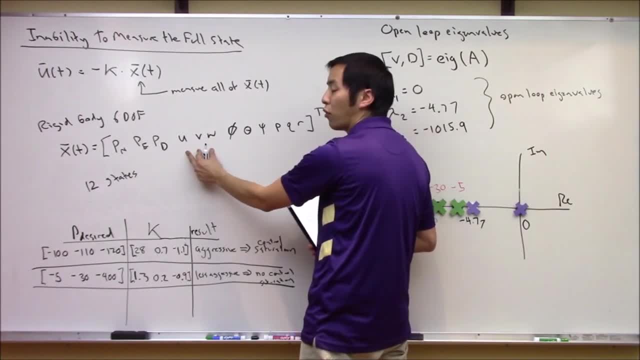 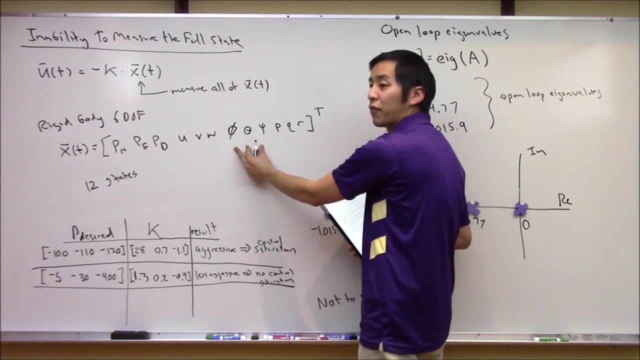 I need um airspeed sensors and, uh, five hole probes and angle of attack veins and something like that to measure the velocity here. Right, I need um, uh, you know, some kind of inertial measurement unit here to measure all of the Euler angles. 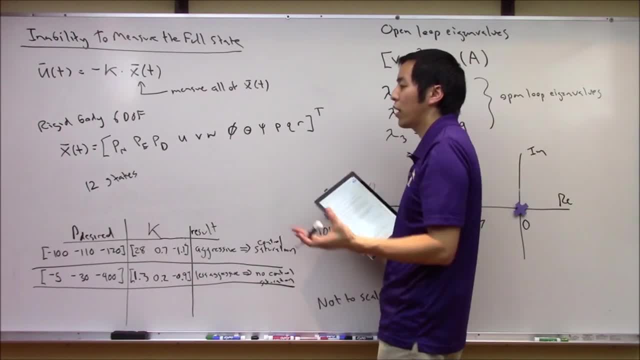 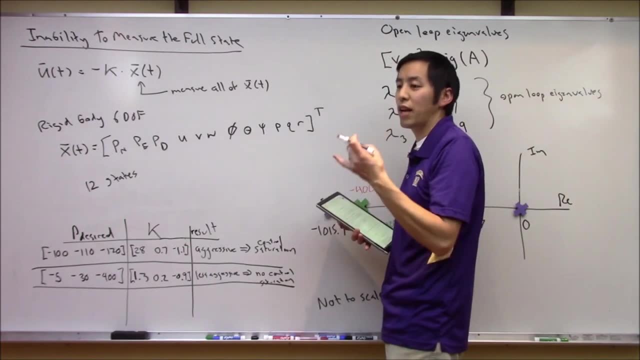 I need rate gyros to get all these. So you can see here that quickly, if your system is somewhat complicated, uh, this can get expensive here. Right, Because you need to implement, or you need to purchase and directly measure accurately every single state in your system in order to implement this. 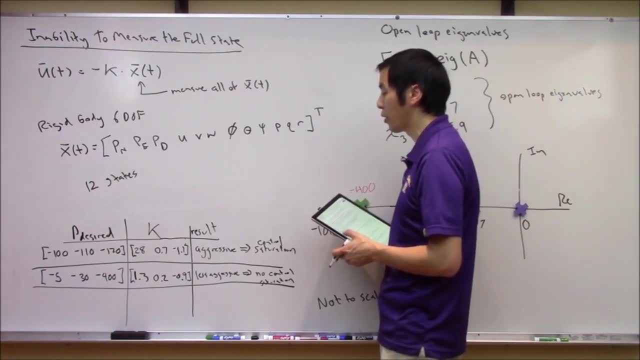 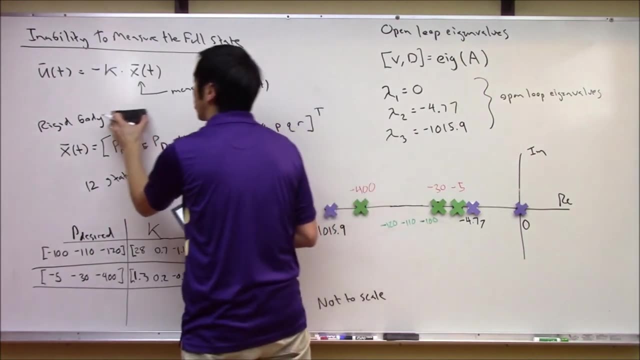 So this is one of the major issues that that we end up with, And we see we actually run into this with our simple DC motor system. So let's, let's consider our DC motor. So maybe let's change this instead of the aircraft example. 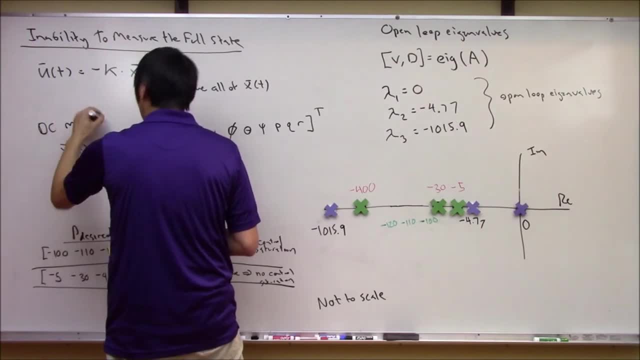 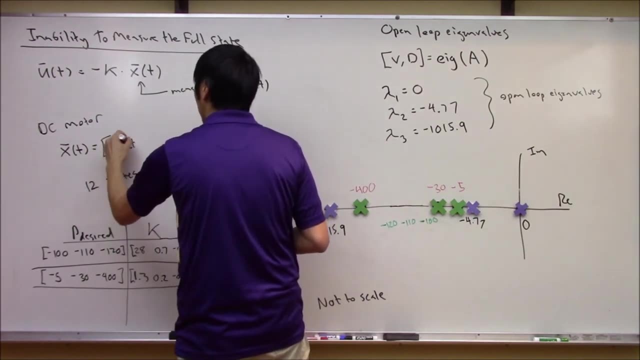 Let's just look at example of our DC motor, Right. So our DC motor was just three states here, Right, It was just the position of the motor. Right, The velocity of the motor and the current running through the motor here Right. 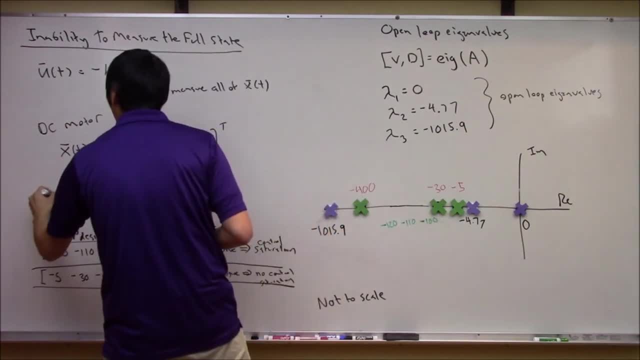 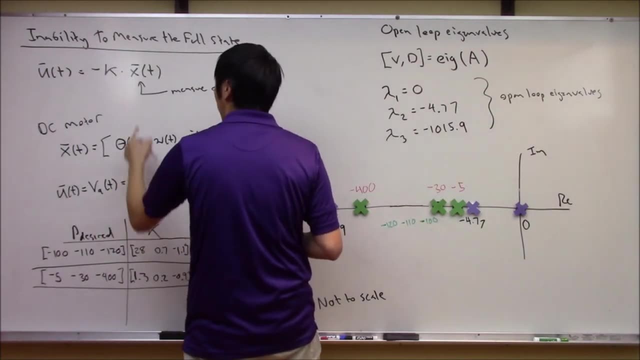 So the control law in this case here is: if you write this thing out Right, U of T, which is effectively the armature voltage, Right, This is going to be minus K, Right, So there's like a K1, K2, K3 times X. 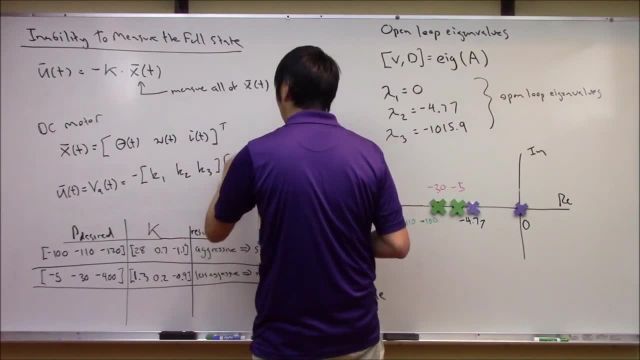 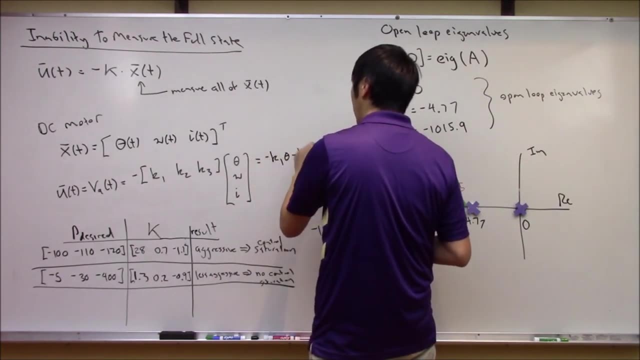 Right, Which is theta, omega and and current here, Right. So again, writing this thing out, you get what You get minus K1 theta, minus K2 omega, minus K3 times I Right. This is how the armature voltage is is computed. 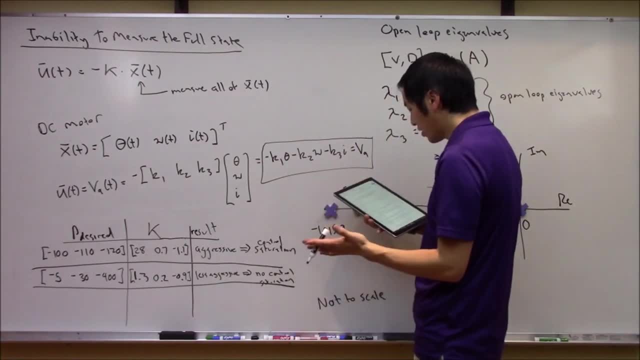 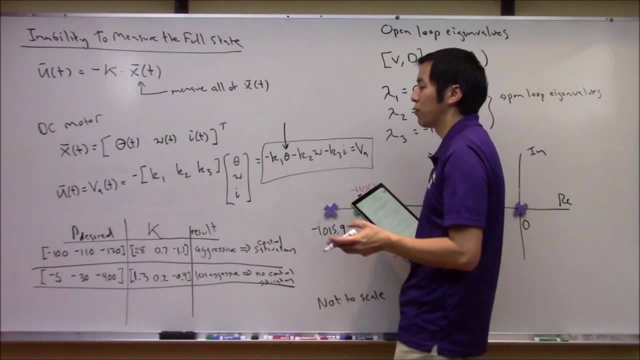 Right, So this is my control law here, Right? Well, in our situation here, what can we directly measure? Right, We have an encoder that will measure the position here. Right, Let's assume that this system, you know, in real life the only thing we have in the lab here is we can measure theta here. 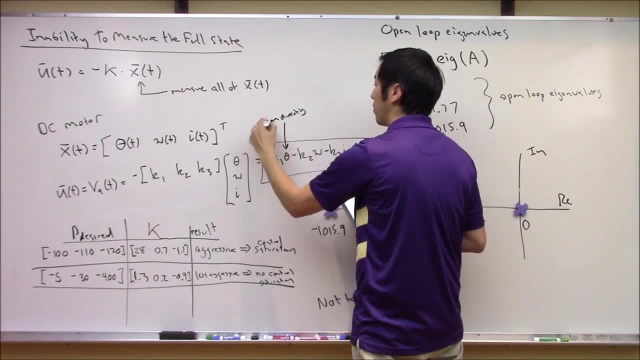 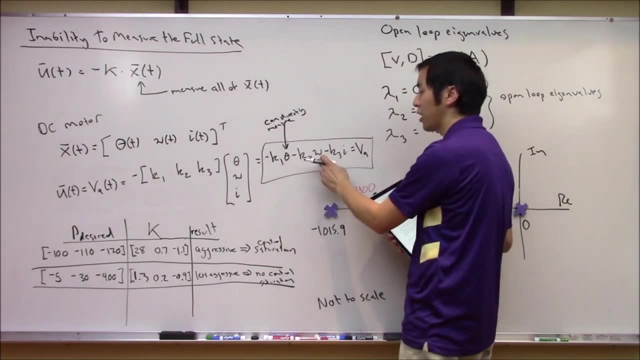 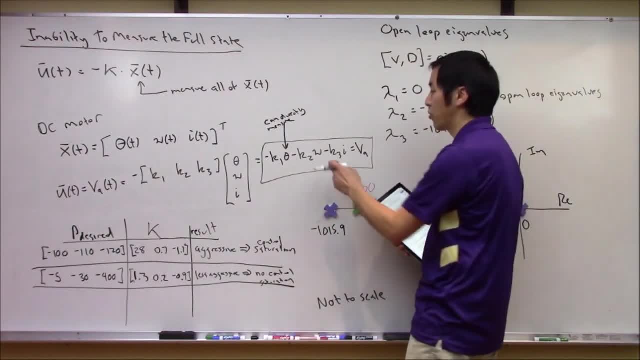 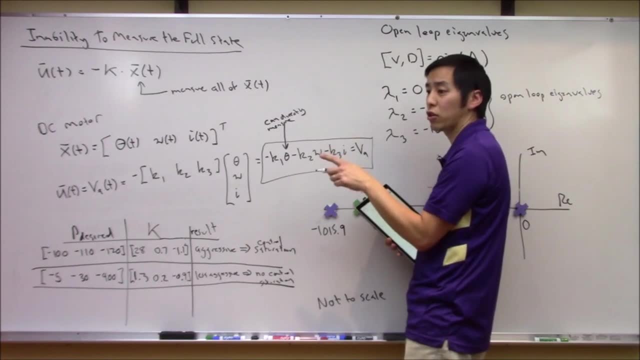 Right, Sure, you can probably make some approximations, like you can probably take try to take a numerical derivative of the position here. But I think, if you're remembering, in one of our previous discussions here on practical PID controllers, we saw that there were some real issues when you try to take a numerical derivative in real life here. 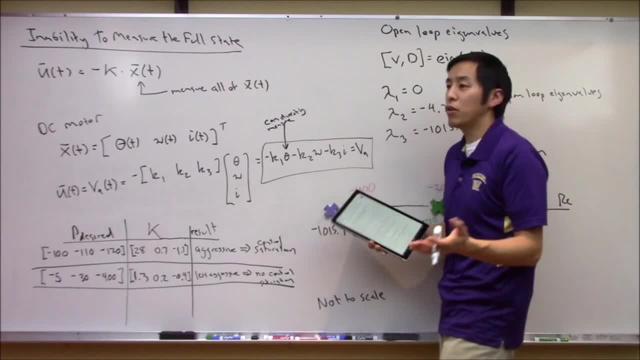 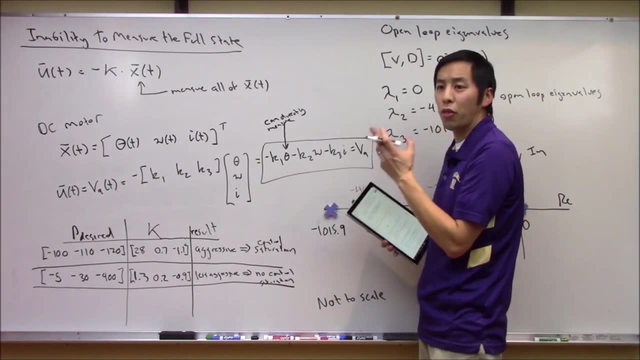 So you can't get omega. Sure, you can maybe do things like like this, like pseudo-derivatives or other techniques here, But, long story short, you can't directly measure this, So theoretically you cannot actually find this, So you can't implement this. 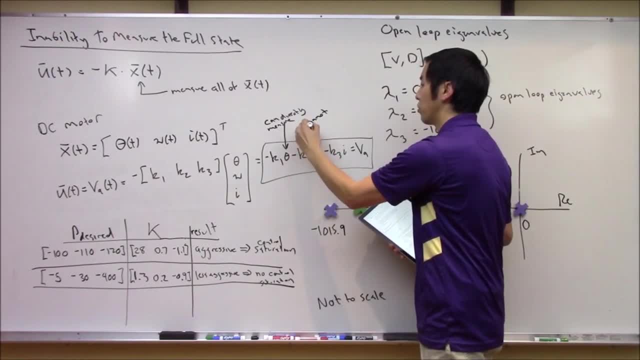 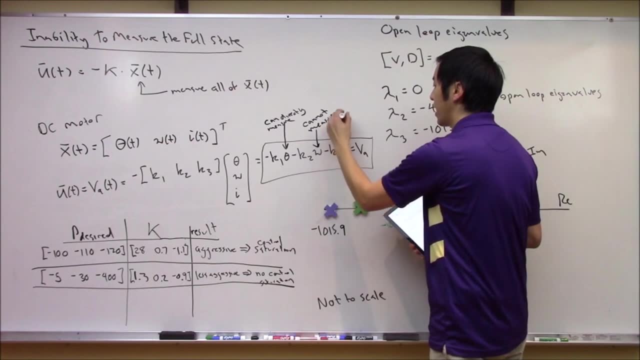 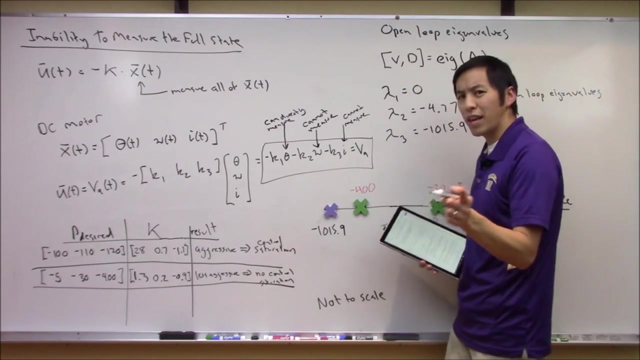 So let's just mark this as a cannot measure, right. And then the current again. there's no way we're going to directly measure the current here, So this is another cannot measure, right. Maybe this is actually a good spot to maybe put another shameless plug-in. 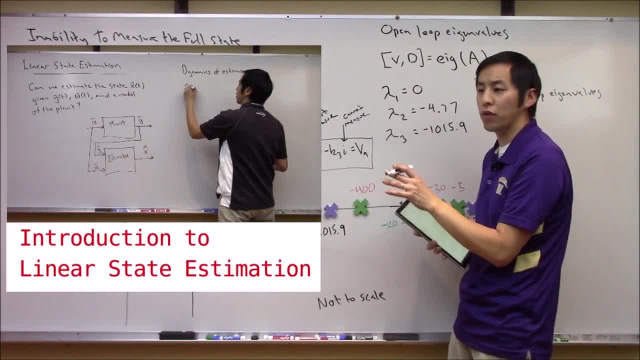 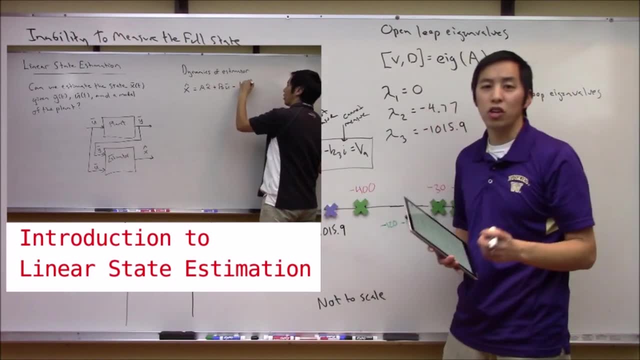 for one of our other videos here. This sets the stage here for this concept of called state estimation here, where you will eventually, you know, based on some of the states that you might be able to measure. can you somehow estimate some of these other states here, right? 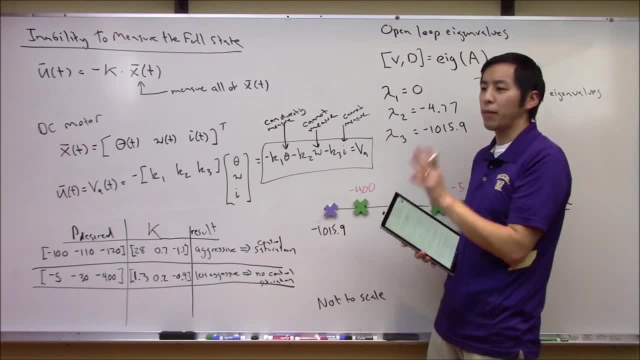 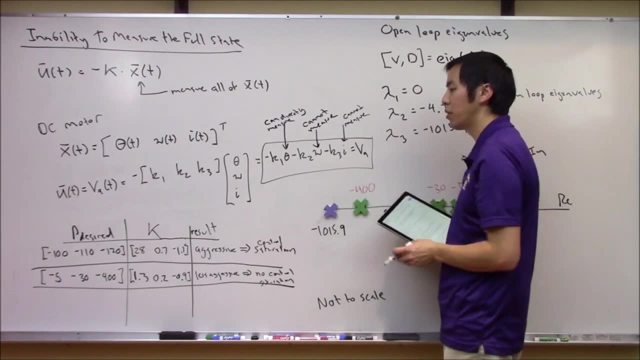 But let's forget about that for this discussion here Right now. I just want to talk about pure full-state feedback controllers here. So in our situation, we can't actually measure these two things here, right, So what we could maybe try. 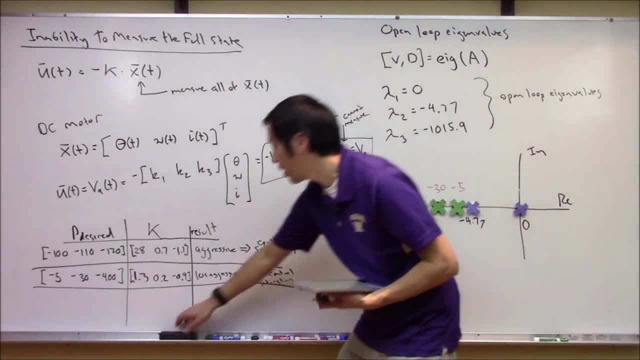 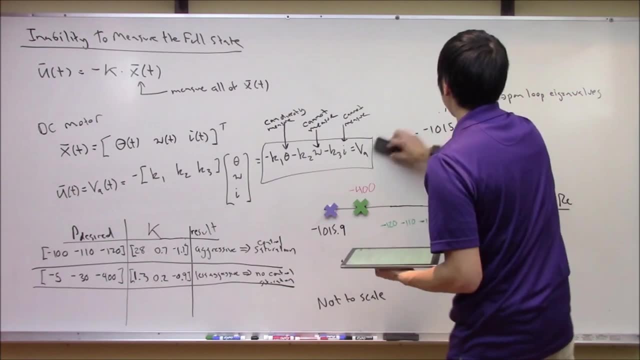 try to do here is, you know, the best that we could implement here, the best that we could hope to do here, is: let me see, maybe let's erase some of this. I don't think we need this any longer- is since we are not able to measure. 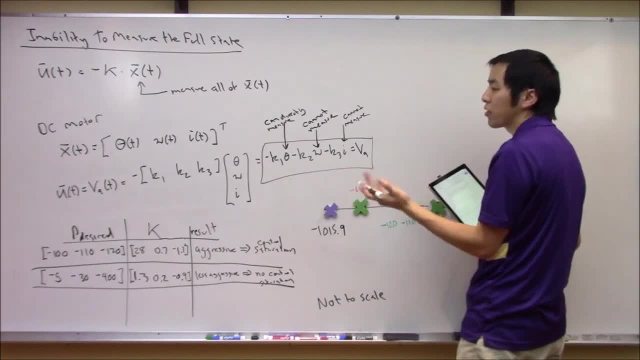 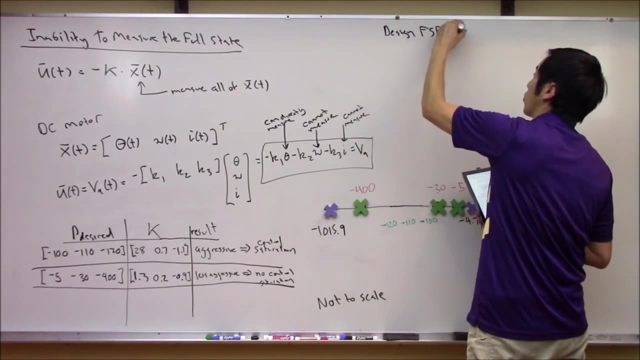 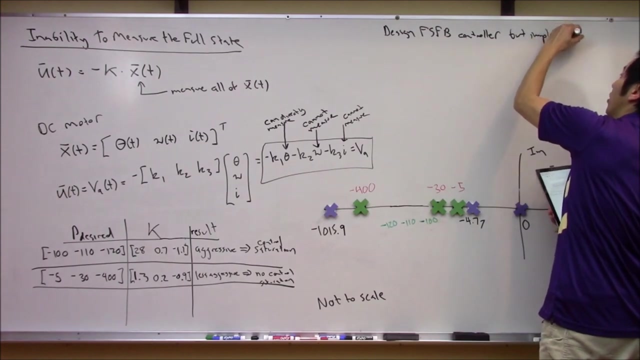 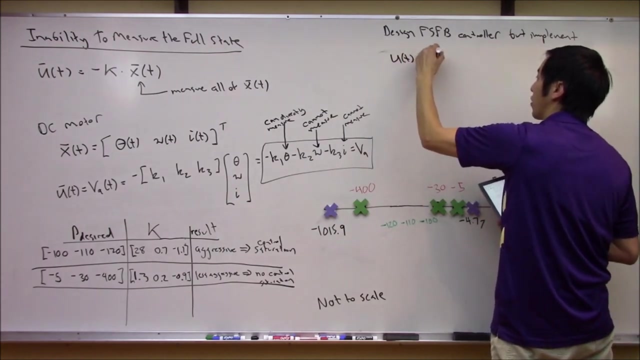 the full state of the system. we could try an approximate control law- right, So we could design a full-state feedback controller- right. But let's implement something simpler. We could implement like U right, Which, sorry U, which is just VA right. 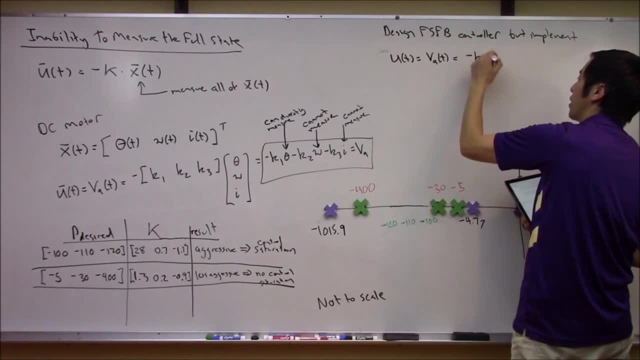 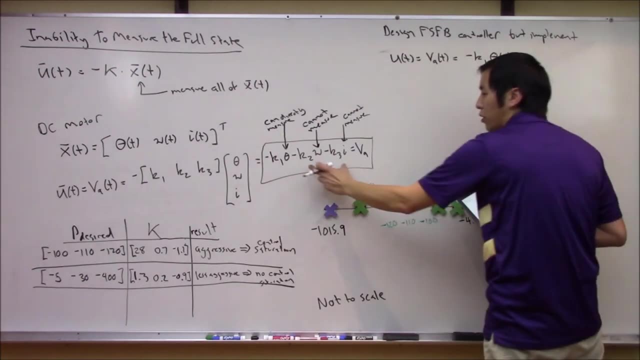 The armature voltage. It's just let's just try minus K1 times theta right, Because I can't measure omega and I so I have no frigging clue what they are. So let's just maybe pretend like K2 and K3. 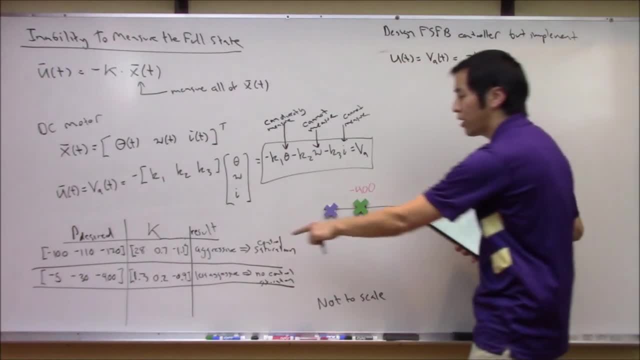 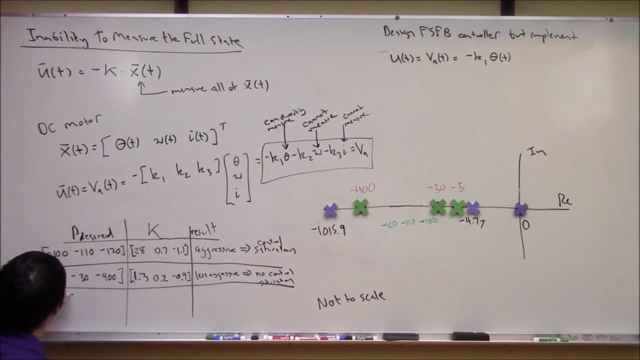 are equal to zero here, right? So let's try that. So maybe, coming down here in our table here, let's try this exact same thing here. Let's go ahead and do a minus five, minus 30,, minus 400 here, right? 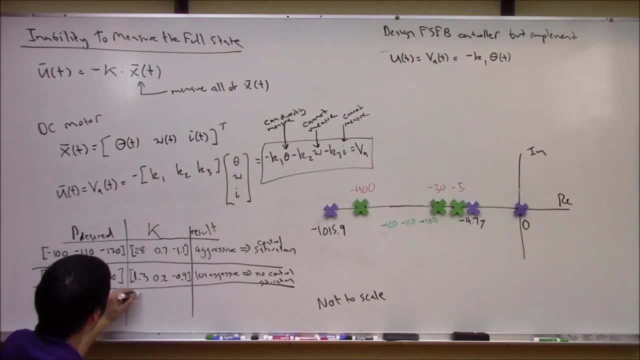 And now what I'm gonna do here is let's just put you know 1.3 here and assume that these other two are zero here, and cross our fingers and hope that that works here right, Because this is the best we can do. 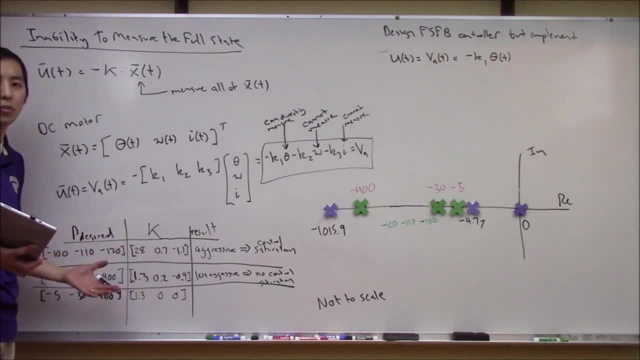 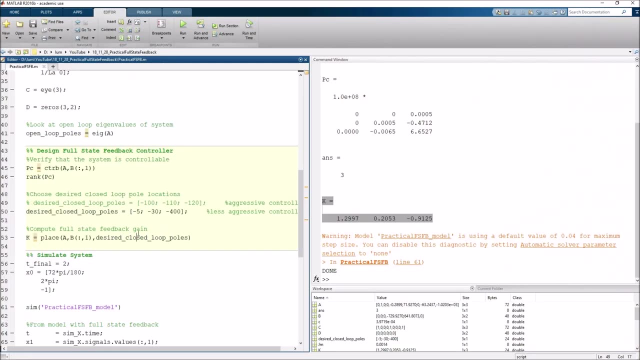 We can't measure these other two states, so let's just assume that their gains are zero. So tell you what? let's run over to MATLAB and just simulate this and see what ends up happening here. All right, So we're back here. 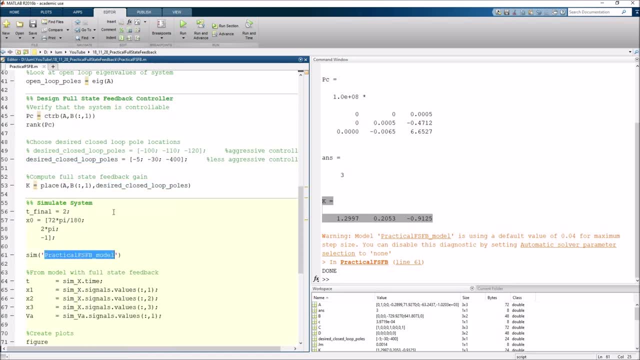 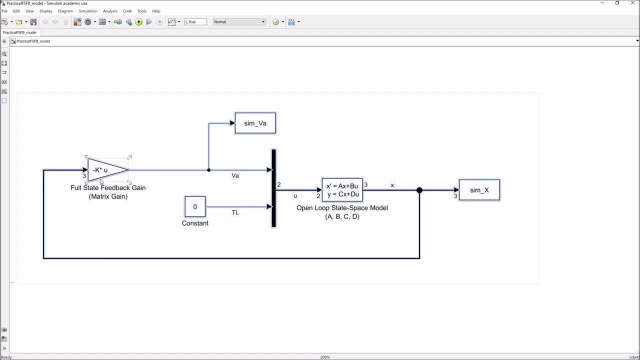 So maybe what we should do here is, in order to simulate the fact where we only use the first gain here. maybe what we should do here is: let's copy this entire block diagram here and let's make a second copy right below it, here. 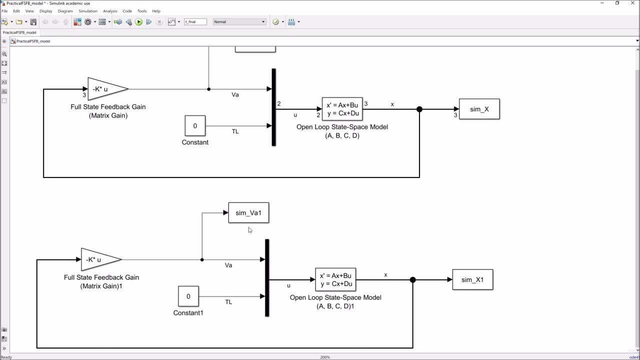 And maybe what we will do here is: let's call this like: instead of VA1, let's call it VA like tilde or something like that for a different version of VA. Same thing for the state here. Let's call this X tilde here. 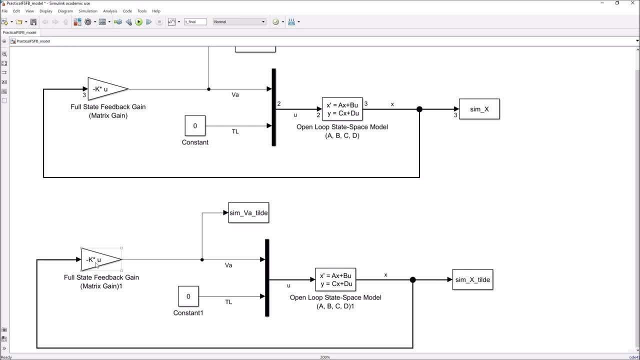 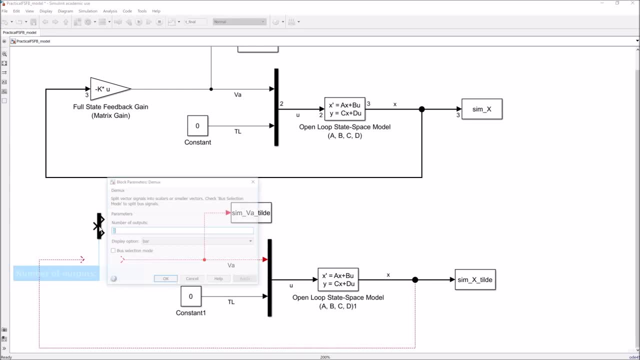 And now, instead of a full gain matrix here, what we should do here is: let's delete this here and maybe pull out a demux, And what I'm going to do is break this up into the three constituent states here of X1, X2, and X3. here. 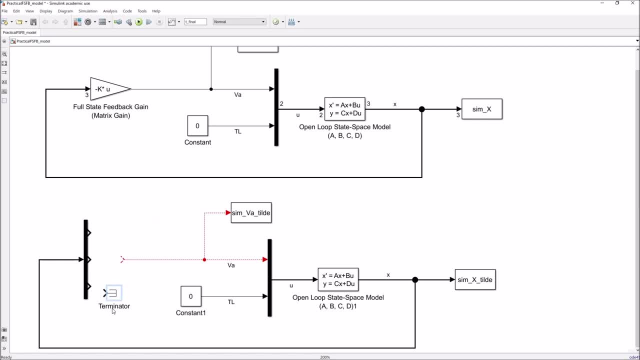 And maybe what we'll do here is: let's just terminate X2 and 3, because we don't know what those are. All right, And instead now what we should do is: let me see if I can pull this up and get a little bit more room. 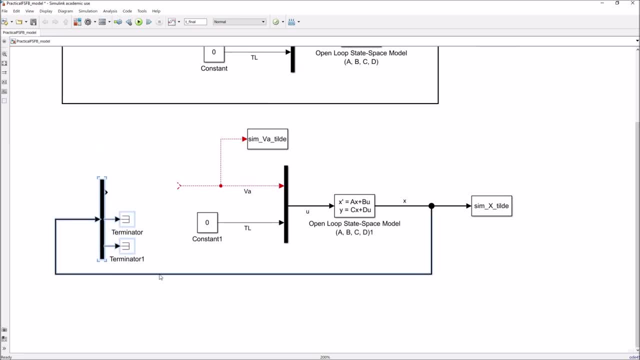 Let me move all this down. Let's see, like something like this: Here we go, Okay, Now let's go ahead and get a gain. Oh, come on, Get a gain. And now this is just going to be minus K sub 1 here. 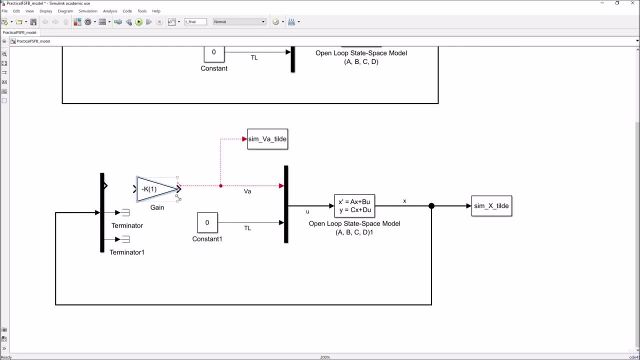 Right. So this is just the first value here And since it's just a single value, element-wise, multiplication-wise it's going to be minus K sub 1.. So the multiplication is perfectly fine here, right? So if I connect this up, does everyone see what I'm doing here? 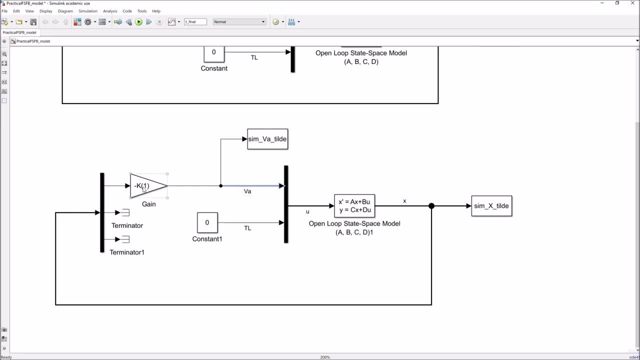 So, in this situation, my control signal now it's just the first element of my full-state feedback controller, multiplied by the only value of the state that I'm actually able to directly measure here, right? So I'm going to now run these two systems in parallel here, right? 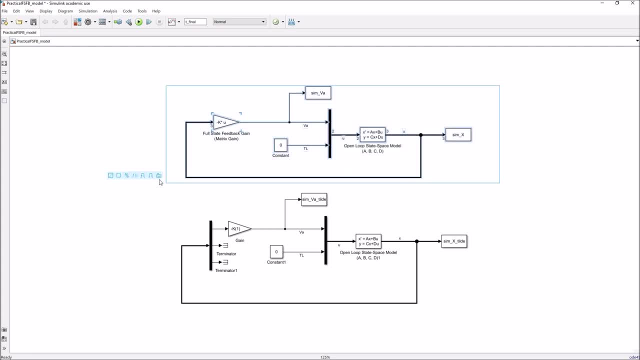 So the one on top is the full, full-state feedback controller as we designed it to be here, right. So this is what would be awesome to have if we had the money to buy sensors for every single state of my system. And this bottom system is basically trying to be. 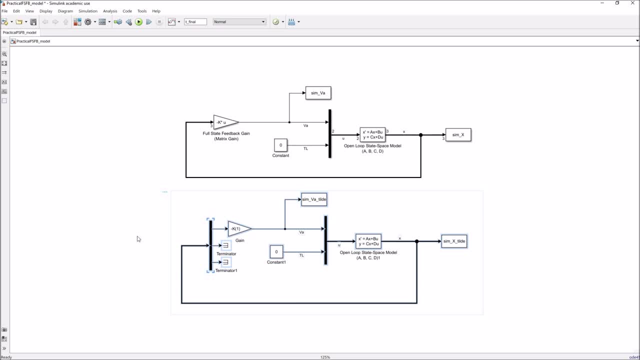 a more realistic simulation of what you might encounter in real life, where you're not able to measure the entire full state. So we're going to have to kind of hobble along and limp by using only the measurements that we actually are able to directly obtain here, right, 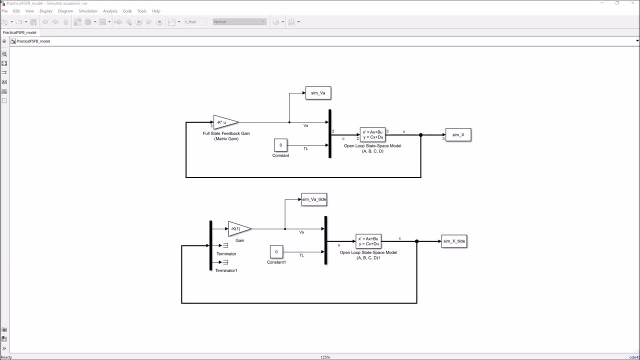 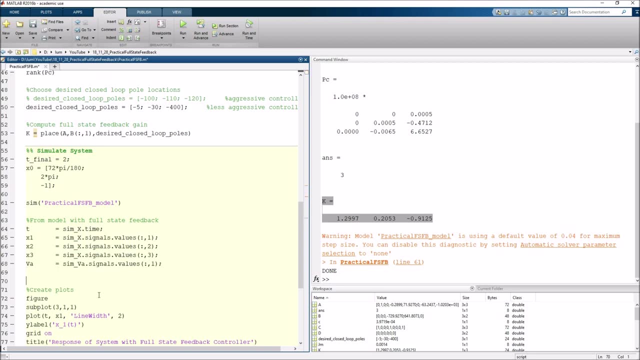 Okay, so let's go ahead and save this And we'll come back to the MATLAB script And basically we will run this again, And maybe what we should do now is: now let's look at maybe, how does the other states do here. 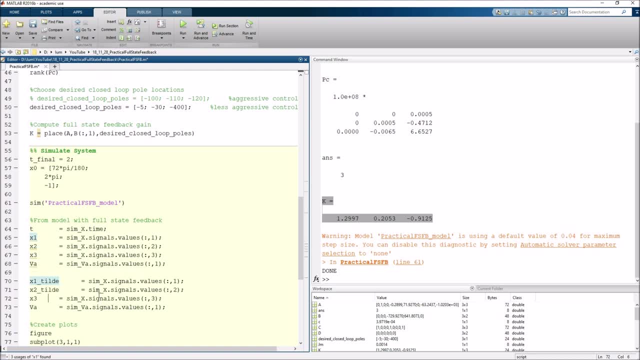 So let's look at x1 tilde, x2 tilde, x3 tilde and va tilde, And obviously, maybe what I should do here is make sure that we are pulling off the appropriate signals here, right? So this is x tilde, va tilde here, right. 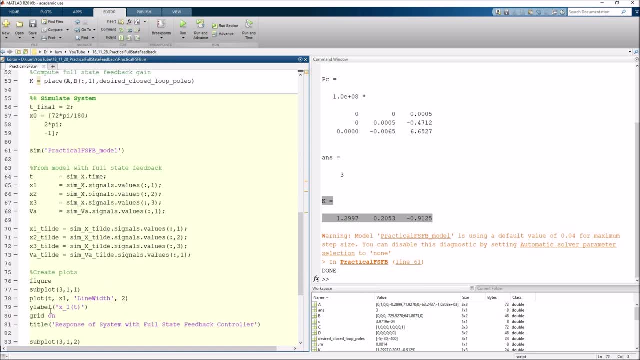 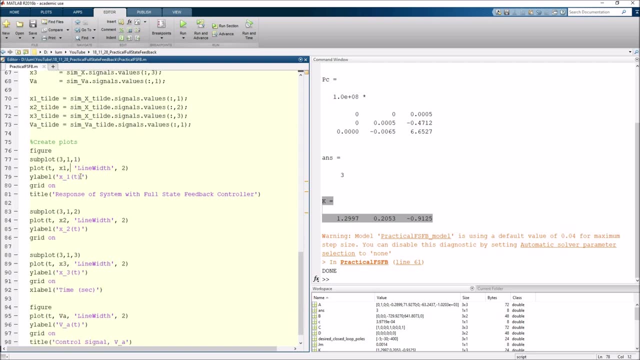 So now x1,, x2, and x3, again are the state trajectories under that crippled controller here. So let's go ahead and plot them all on top of the full states here, right? So t, x1, tilde here. 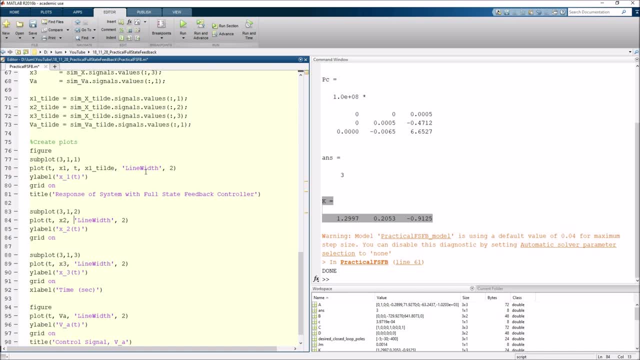 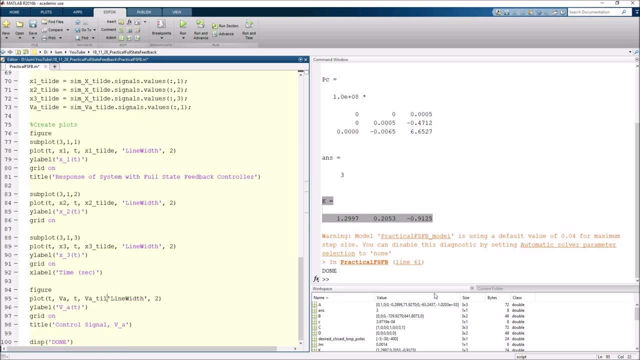 And then let's do the same thing for x2.. And finally for x3.. And then finally, here for the this as well. here, right For the control signal here. So va tilde, Okay, great. So now what we should do is we'll plot both of them on top of each other. 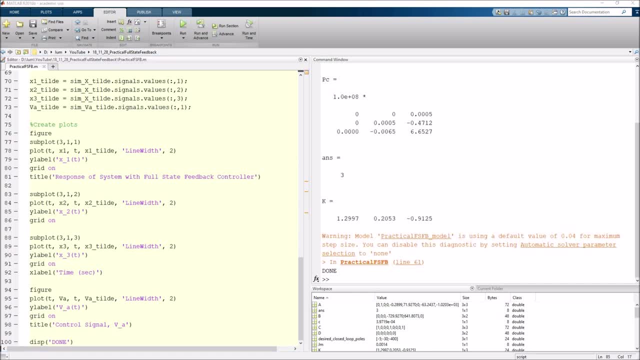 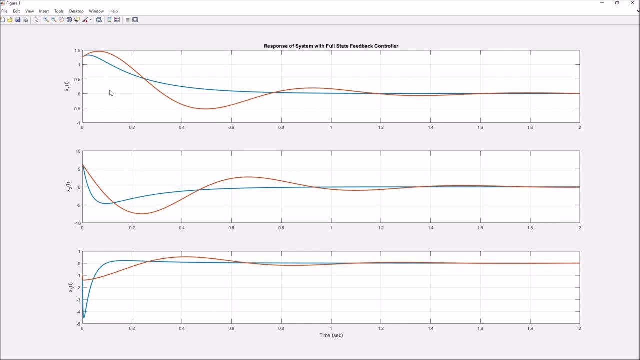 So let's run this simulation here and see what we end up with here. So first let's take a look at the states. And here we are. So you see, here now we're incurring some penalties and the system is not performing the way we expected, right? 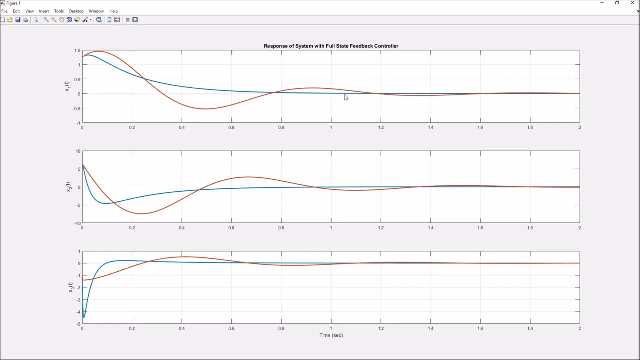 The blue line is what we had earlier and we were totally happy with that right. It settled in one second. It did not seem to work. Let's try to saturate the control signal. Maybe we can Let me pull the control signal over here. 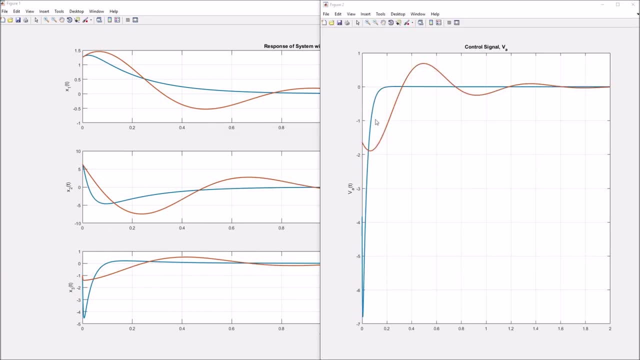 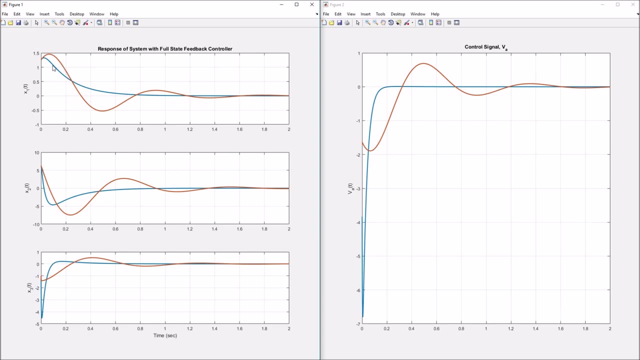 and maybe we can stare at both of them simultaneously. Yeah, maybe let's see if we can put one on this side and then one on the other side, right? So here we go, And now blue is what we wanted here, but since we can't measure the full state of the system, 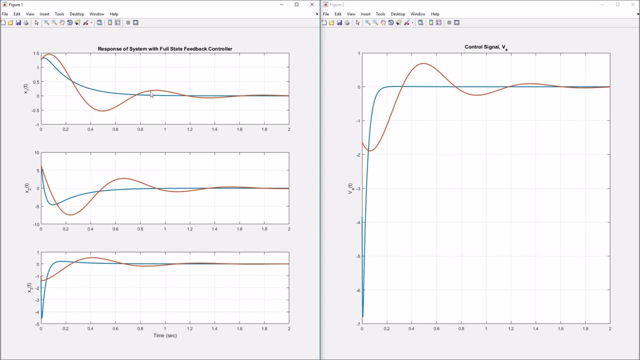 red is what we actually have, And you can see now. this is the problem here, right, When you're not able to measure the full state of the system, you just can't make a full state feedback controller, So we end up with a scenario. 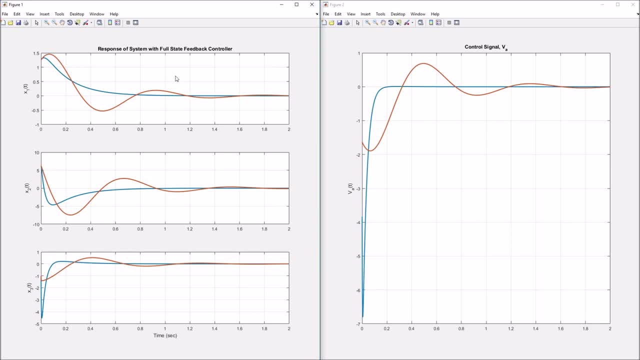 where the performance is severely degraded. right, We now have these oscillations as it's trying to settle here, So this is again not ideal here, but this is one of the practical problems that you have to deal with when you're trying to use a full state feedback controller. 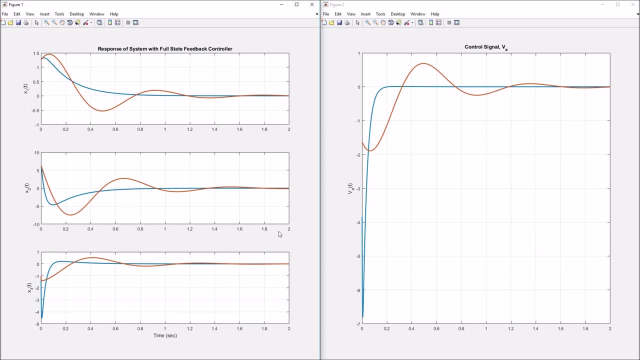 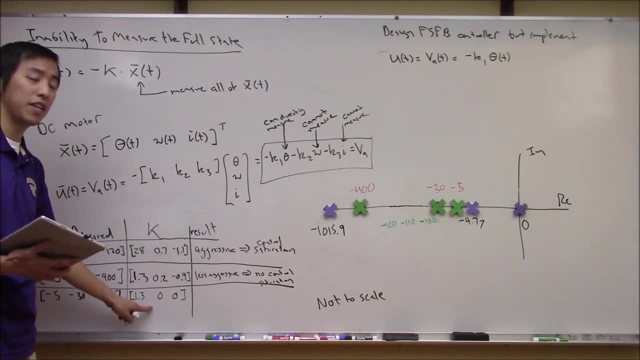 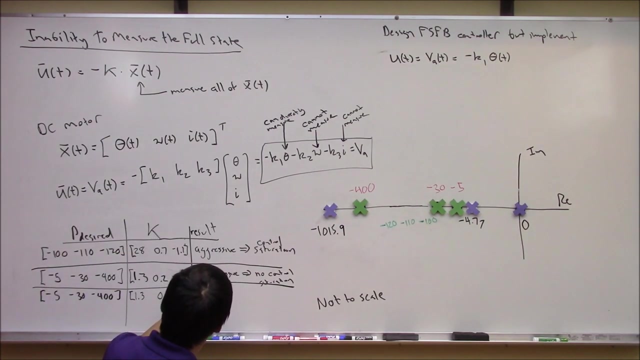 on a real system where you might not be able to measure the full actual state of the plant. Okay, so we saw that this control scheme here didn't really work here, right? So we saw that this had significant degradations, right. 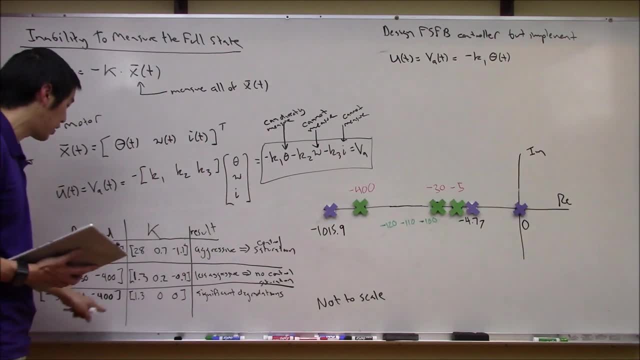 There were these oscillations, It didn't really behave the way we expected We were. basically, we got some surprises when we tried to do this And the surprises stem from the fact that, really, your full state feedback controller- right we saw- had non-trivial elements here for K2 and K3. 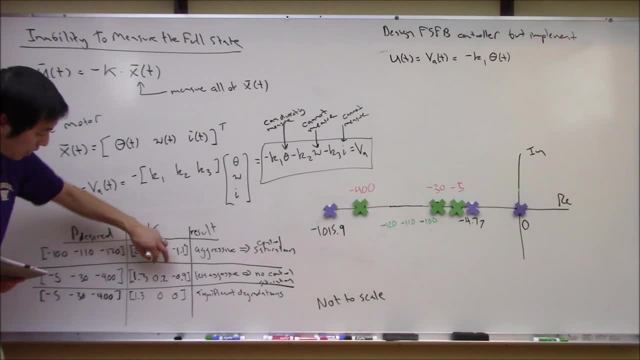 These are not trivial when compared to the K1 here, right? So this concept leads to a little bit of intuition of maybe another way that we could try to tackle this problem here of not being able to measure the full state. So the idea with this now is that you know what? 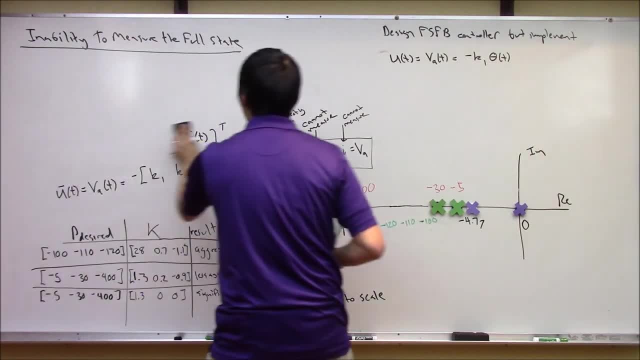 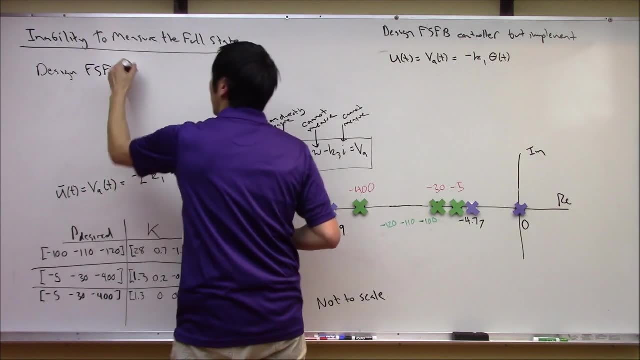 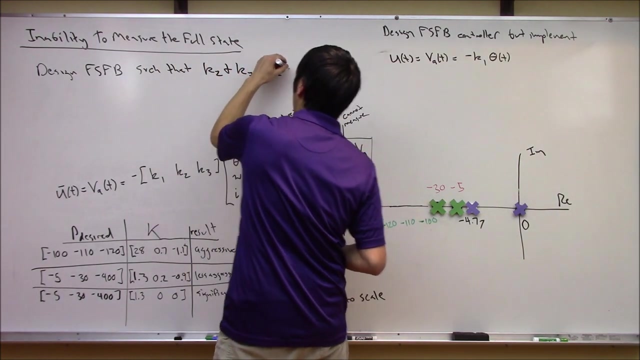 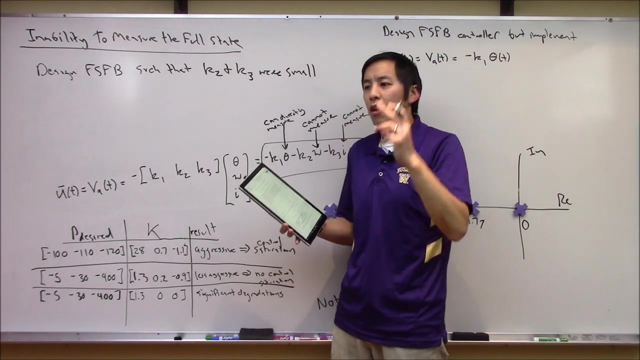 It would be really great if we were to somehow be able to design our system, our full state feedback controller here, such that K2 and K3 were small right, If we were somehow able to basically pick locations of poles, send that to the place command, cross our fingers. 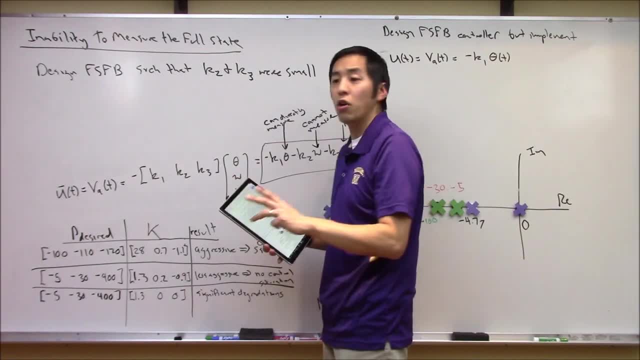 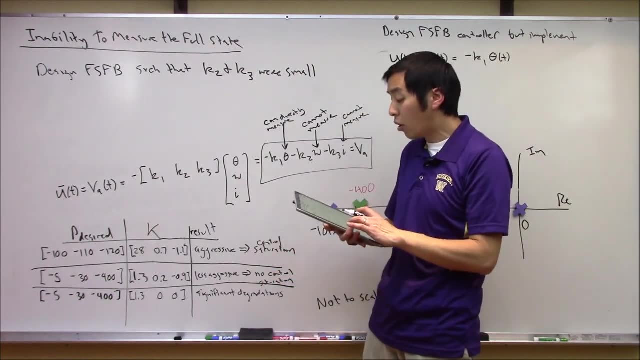 and hope, hope, hope that K2 and K3 were small. then in that case this scheme where we just neglect K2 and K3 would be totally fine. We wouldn't be surprised at all here, right? So the game plan at this point here. 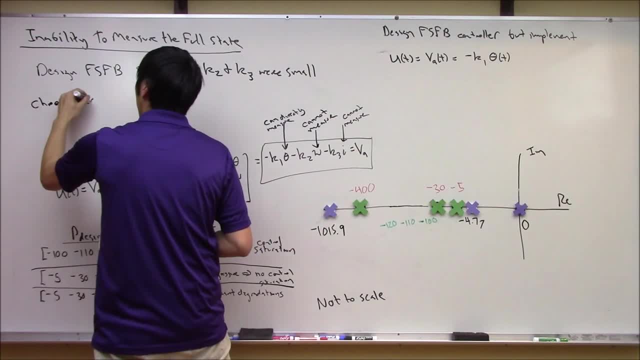 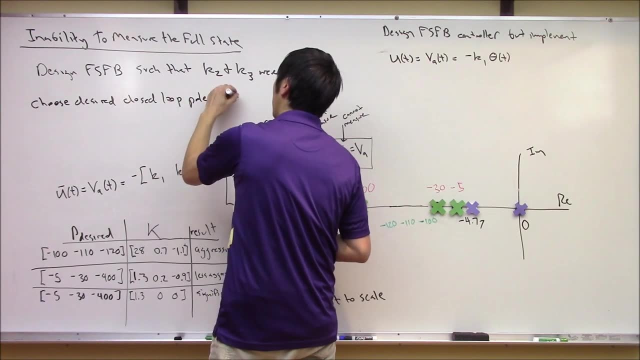 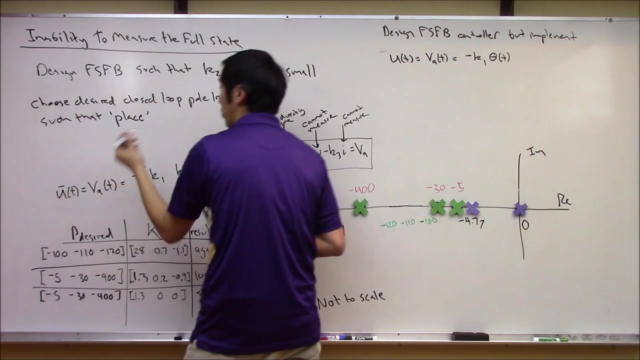 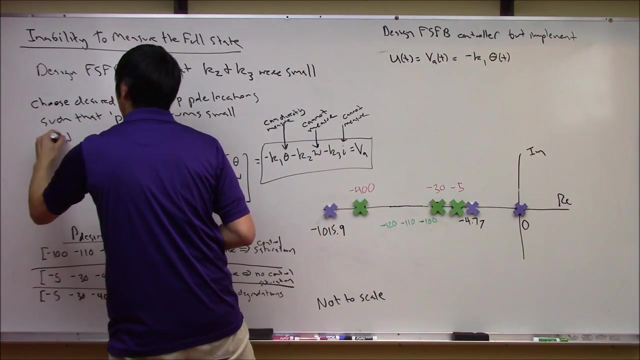 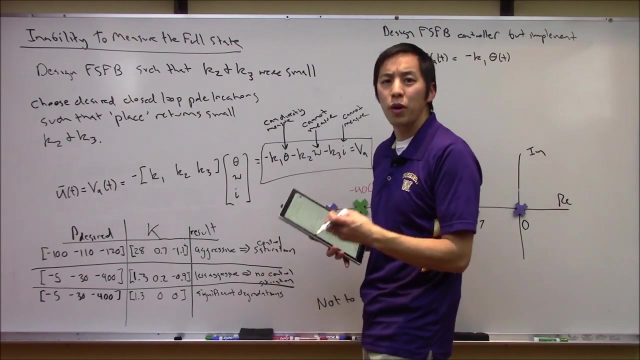 is to choose desired closed loop pole locations such that the place command right or our pole placement procedure returns small K2 and K3.. Okay, All right. So how are we going to do that? Which poles should we move here to hopefully allow K2 and K3 to be small here? 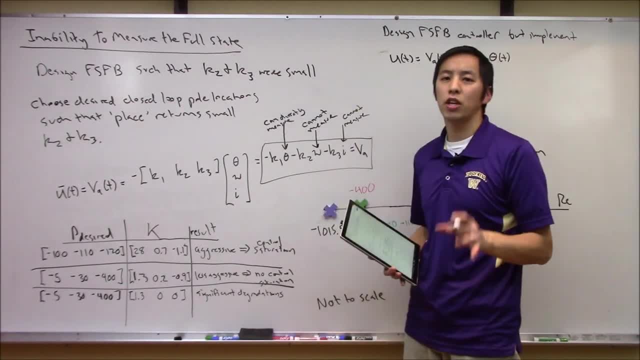 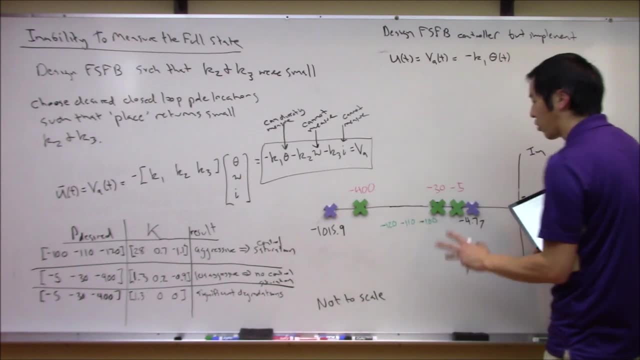 So this is where actually a little bit of physical intuition about the plant is going to help us here. right, Let's come back to this picture that we had. right, There were three blue Xs right. These were the open loop poles here, right? 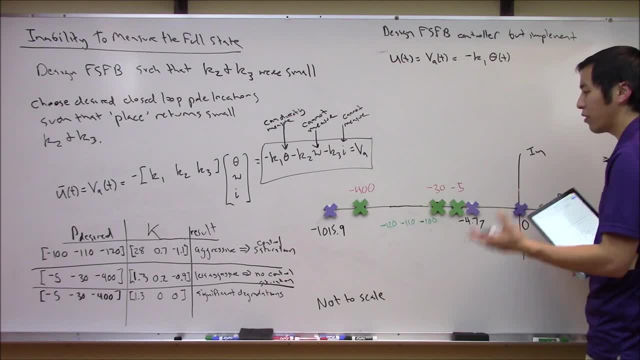 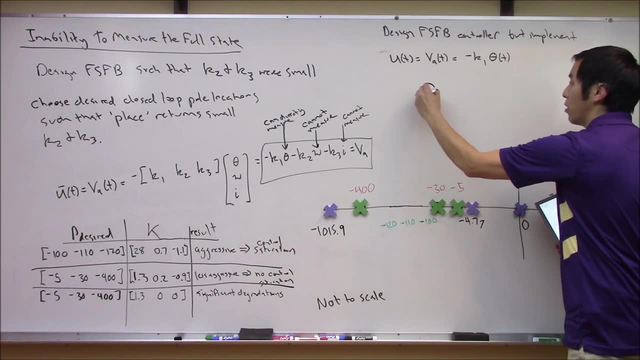 We can think: what are all of these poles and what are they associated here with? So, if you think about this, there's a pole at the origin right here, right? So this lambda one of zero, this is basically a pole at the origin, right? 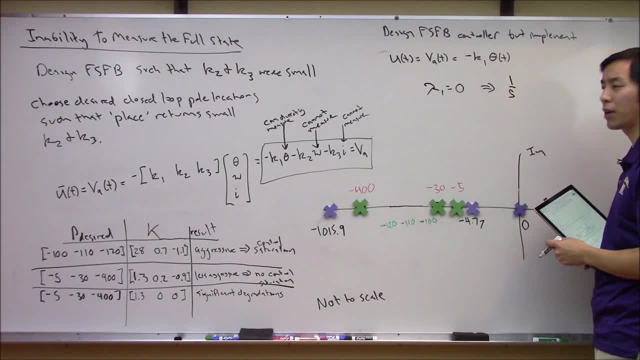 This is something like a one over S in the Laplace domain, right? This is basically an integrator, right, Right? Where in this system here is there something to do with a pure integral here? Well, if you look at our state vector here, right. 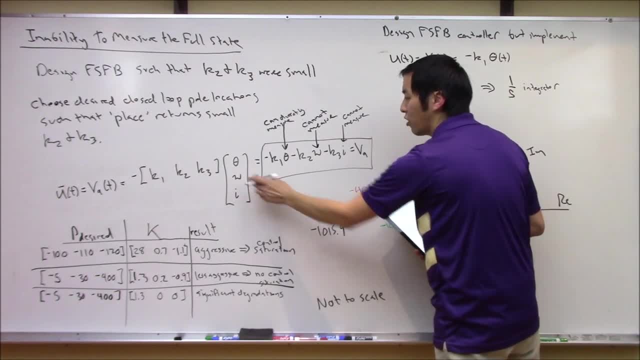 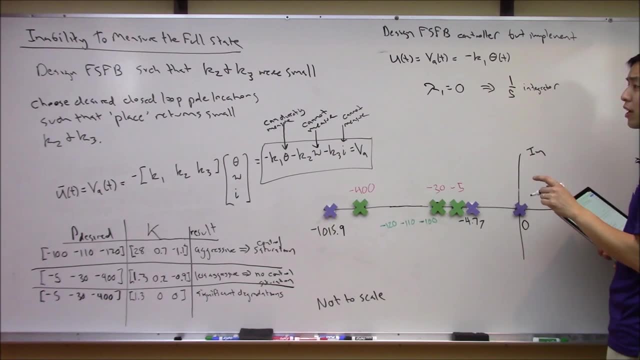 you can see that what Theta is? basically the integral of omega, right? So you can roughly say- and I'm going to have to put a bunch of asterisks here in a second because there's a couple of caveats- but this is approximately related to state theta or X1 here, right? 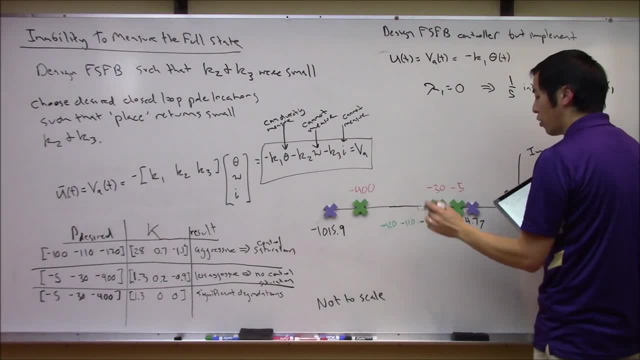 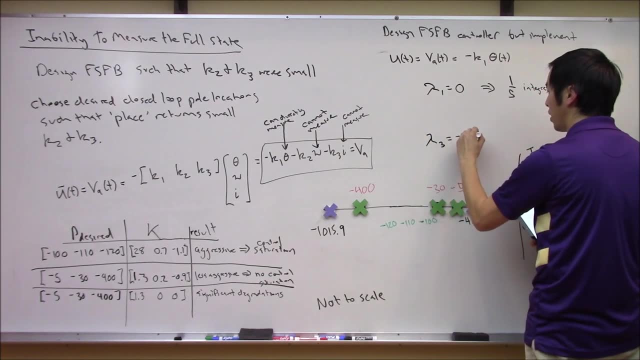 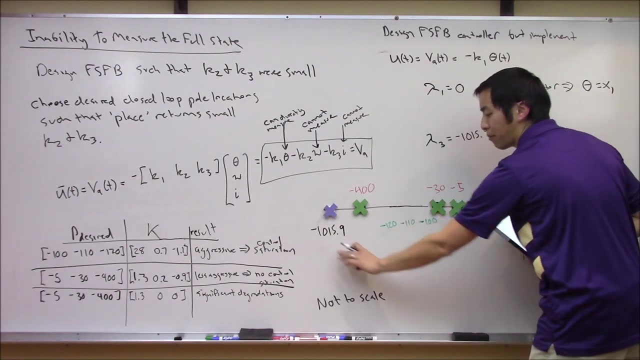 Okay. and then we also know- let's think about this other one here- This lambda three here right, which was at minus 1015.9 here right Physically. what does that mean here right, If you have a pole that's way out here in the left half plane? 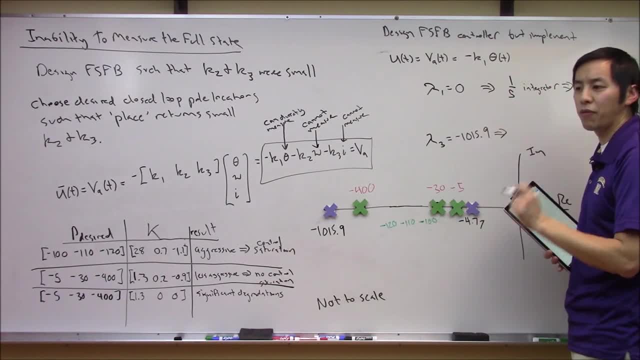 this is something that decays or responds extremely fast, compared to at least these other two blue poles here. right? So this motor here? we got to think to ourselves: what does that mean? Like is there any dynamics here that are very, very fast? 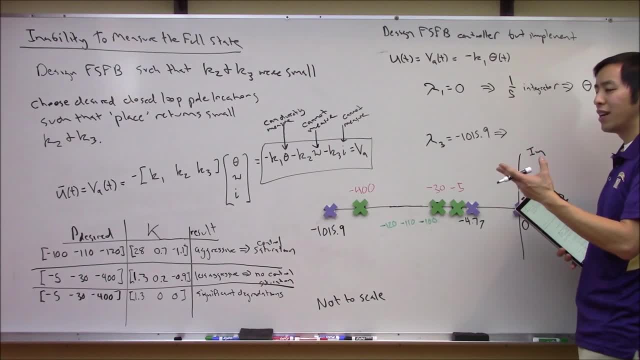 compared to the rest of the system here, right? And we can say, yeah, actually right, the electrical dynamics of this motor are much faster than the mechanical dynamics of the motor of like things, like things rotating. so we can basically say: 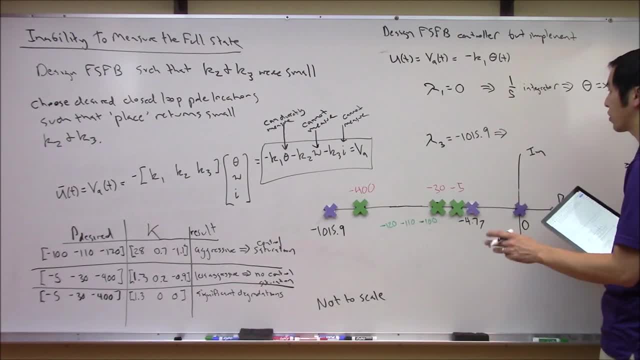 again. this is all very shooting from the hip and with a big asterisk here is that this is approximately. this pole is most likely heavily associated with state of the current here, right or X3, right Because this current, this is the electrical component. 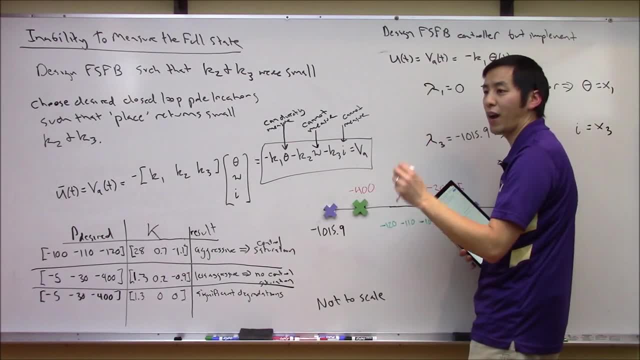 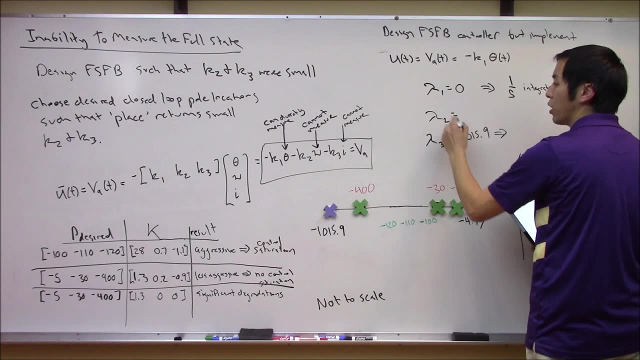 Things with the current die quickly, They change very fast and they reach steady state very, very quickly compared to these other two here right. And then lastly here lambda two here right, which was here at minus 1015.9.. 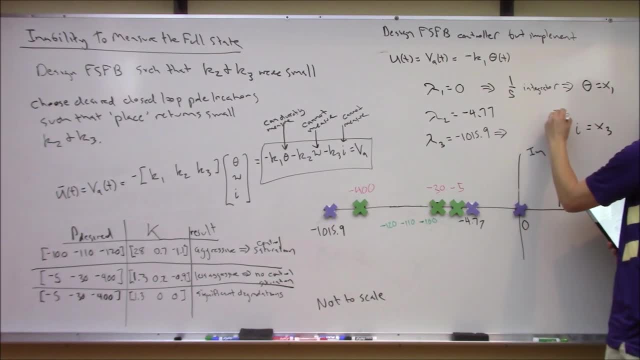 This is 4.77 here, right? We can kind of again roughly say that this has something to do with omega here, or X2, right? So maybe let's label these quickly and maybe again I want to put giant asterisks. 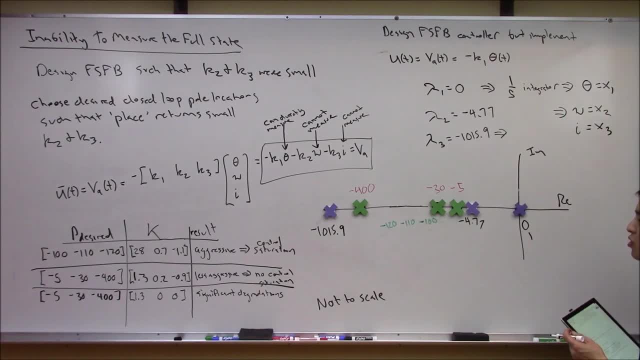 around a lot of this discussion here because you can't really do this in general, but I think for this particular case it works well here. This state we said is mostly associated with theta here. right And again, let's put a big asterisks in here. 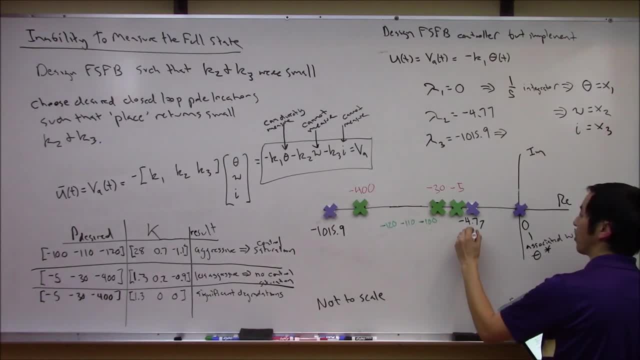 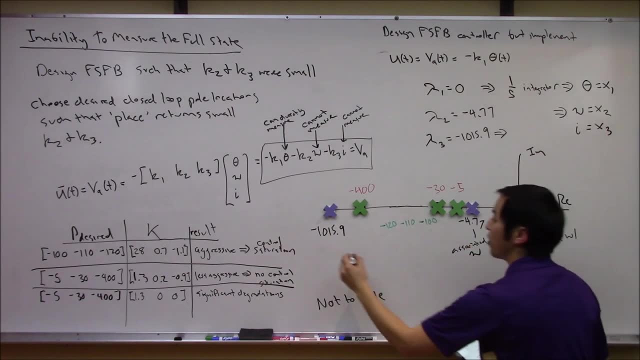 I'll say what that asterisks is in just a second here. This 4.7 here, right, this is associated with omega And this one way out here is associated with, I right, or I guess, X3.. Maybe we should label these as X2 and X1,, right. 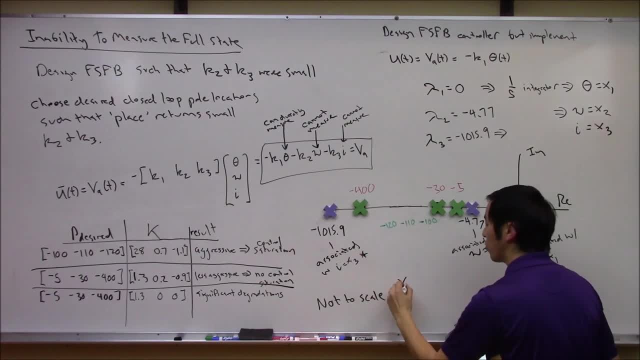 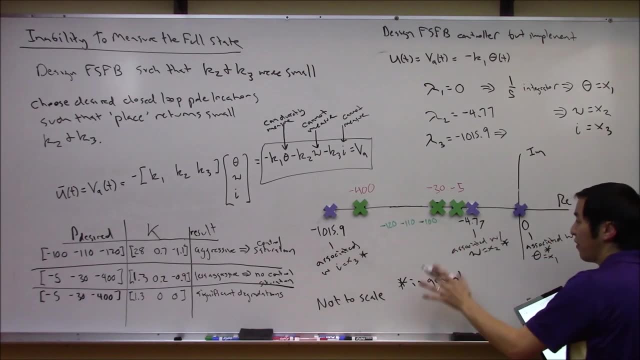 And again, let's put the big asterisks around all of these And the asterisks here. the disclaimer here is that in general- right it's difficult- You can't actually say that a pole or an eigenvalue is directly associated with a state. 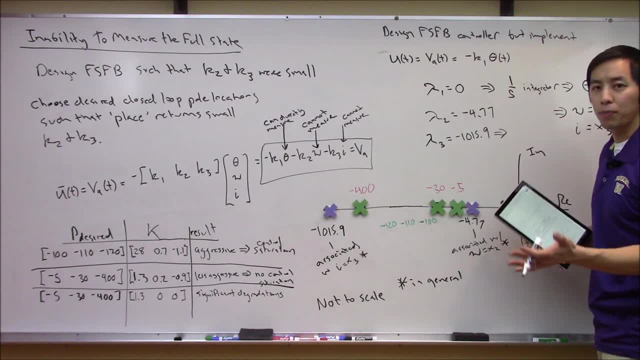 Usually it's associated with multiple states here. right, We have to do a little bit of eigenvalue-eigenvector analysis if we really want to tease out. how much does this eigenvalue influence each state here? Maybe we'll take a look at that. 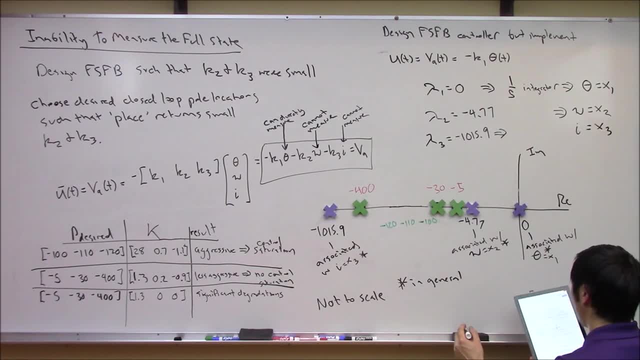 in just a second here. But let's just put this here as a disclaimer here That in general it is difficult- it's not impossible here, but it's difficult- to associate an eigenvalue slash pole with a particular state or states here. right. 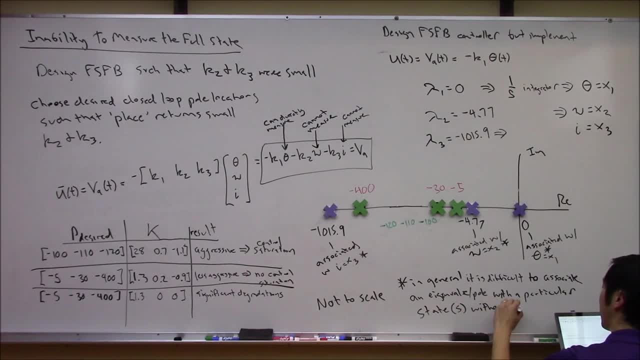 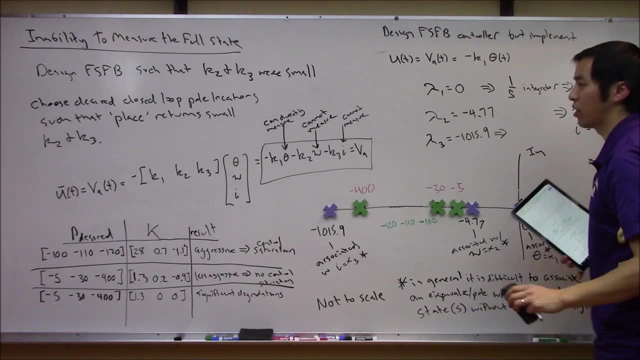 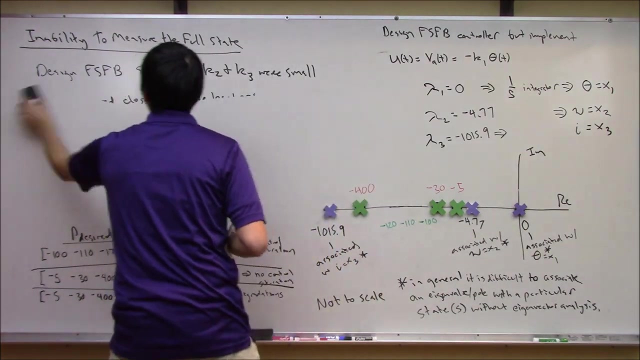 Without without using eigenvalue-eigenvector analysis. Okay, Maybe let's quickly talk about this eigenvector analysis here. Let me erase some of this here. Okay, So the eigenvector analysis that you would have to do again, the derivation of this. 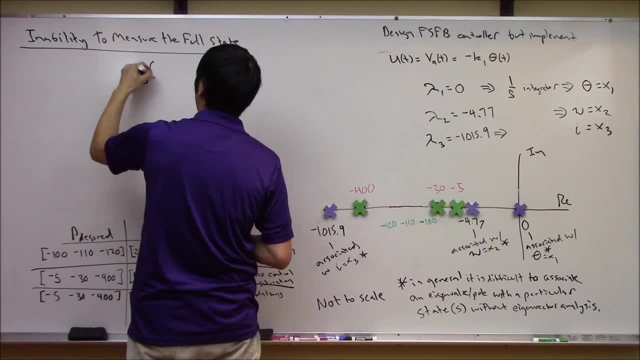 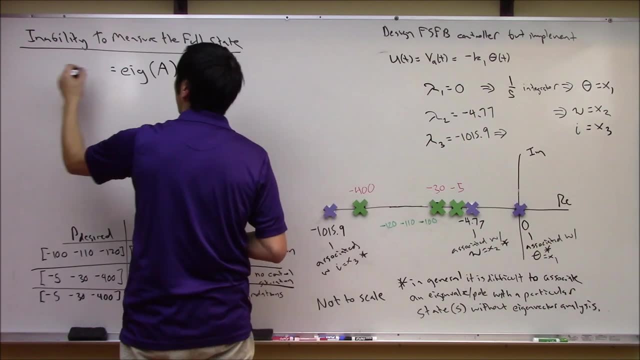 is probably outside the scope of this lecture here. Maybe, if we have some time later, I'll take a dive into that here. But again, if you look at the eigenvalues and the eigenvectors of A and ask it for eig here, 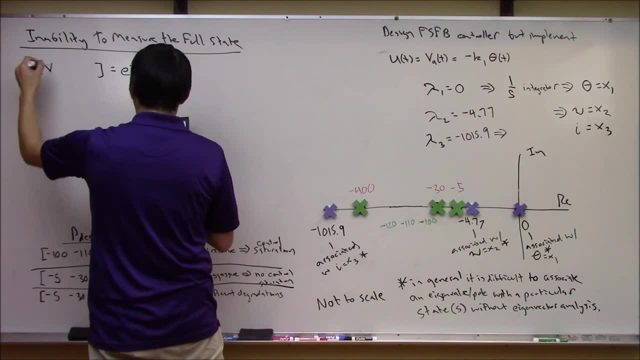 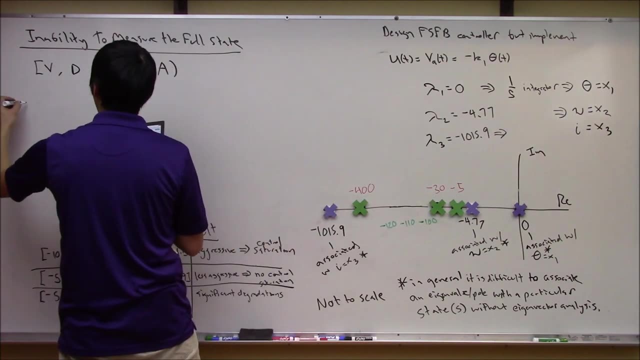 and again. what this is going to return to you here is a bunch of eigenvectors and a diagonal matrix of all the eigenvalues here. So what you're going to see here is that the D matrix here is going to be just a square matrix. 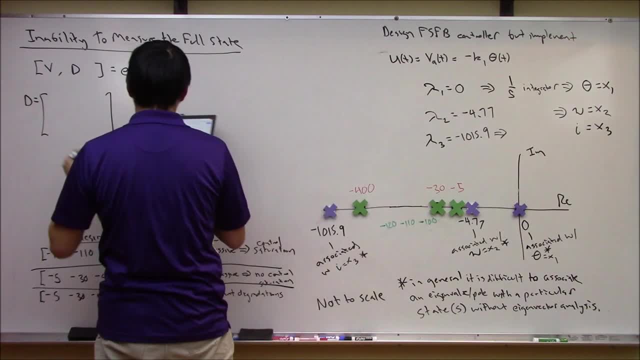 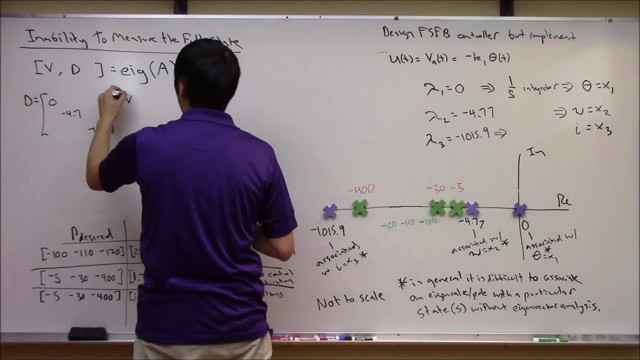 with all the eigenvalues here, These three eigenvalues along the diagonals here right. So it's just going to be 0 minus 4.7, minus 1,015.9 here right And V here is going to be. 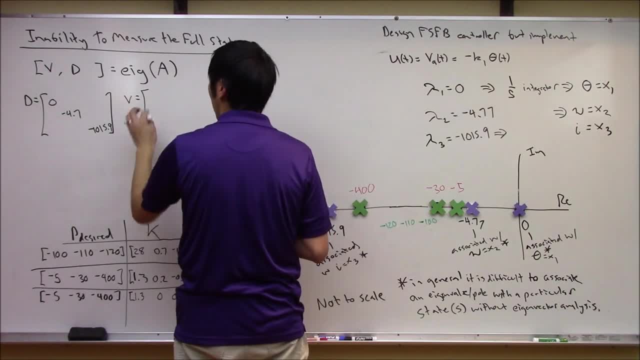 a matrix of all of the eigenvectors for each of these. So the first eigenvector here you're going to get is a 1, 0, 0. Then you're going to get a minus 0.2, 0.97, minus 0.06.. 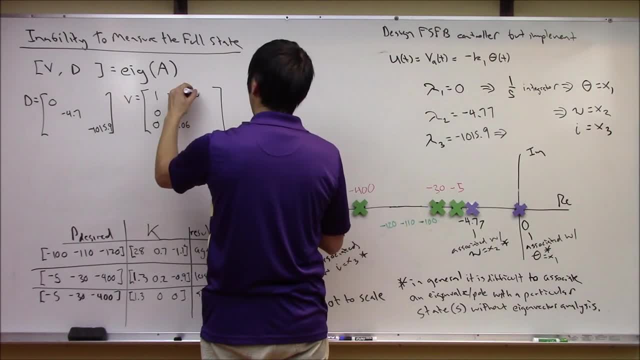 And then finally this one over here. this is going to be 0.0001, 0.0706, 0.9975 here, right, Okay, And I guess maybe we should think about this. I'm going to fill this out. 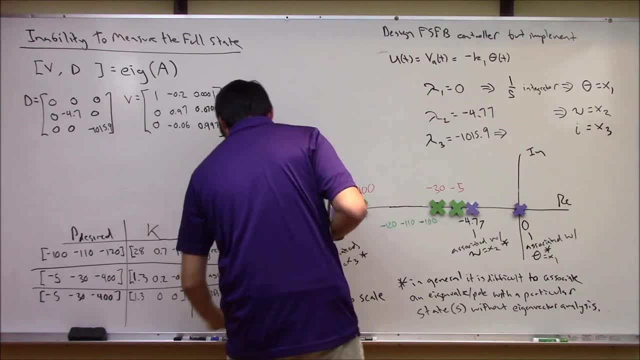 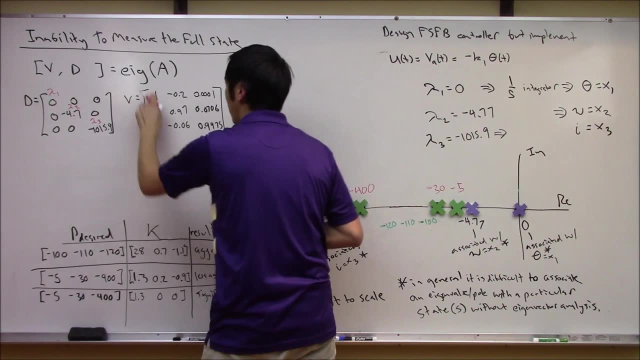 These are all going to be zeros over here, right? So what we see here is here's lambda 1, here's lambda 2, here's lambda 3, here, And then this row here is actually the eigenvector associated with eigenvalue number 1.. 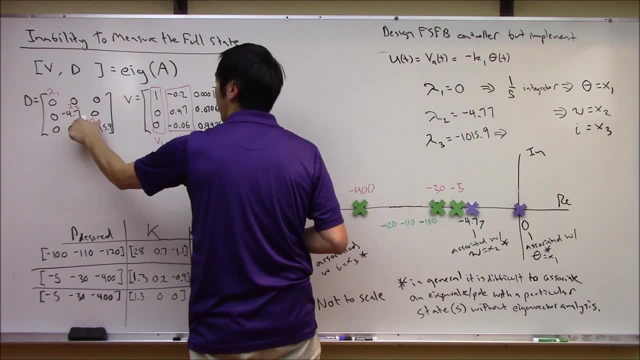 This row here is going to be the eigenvector associated with eigenvalue number 2.. And this, oh sorry column, I keep saying row. These are all columns I'm drawing here. right, This column here is the eigenvector. 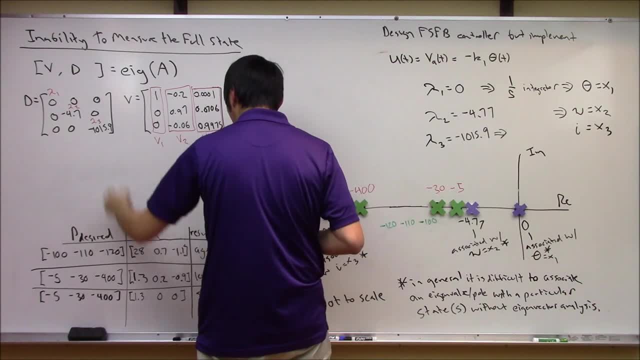 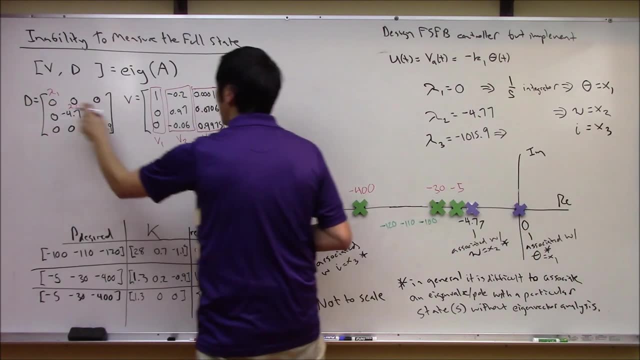 associated with eigenvalue lambda 3 here right. So if you look at this here right, this eigenvalue here of 0, right. you can actually see here that if I line this up with the states here right, x1,, x2, and x3,. 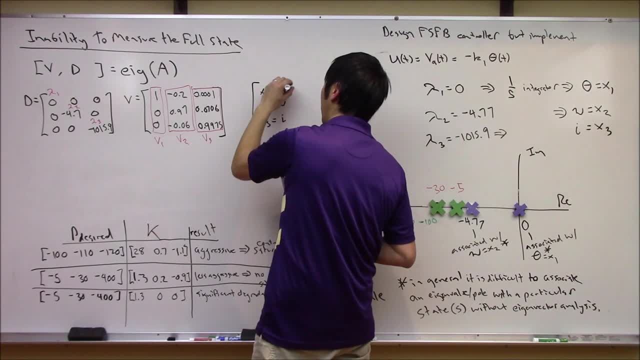 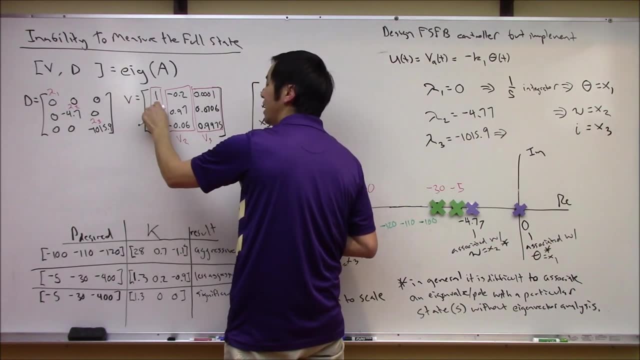 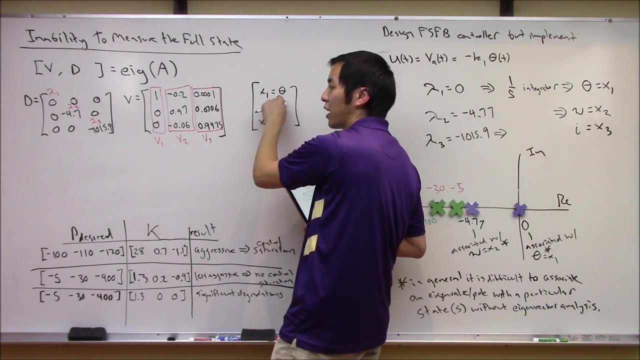 which are theta, omega and i here right. you can basically see that lambda 1 is actually completely and 100% and not in any coupled way here. it's completely associated with the first state here of theta, here right. Lambda 2: here right. 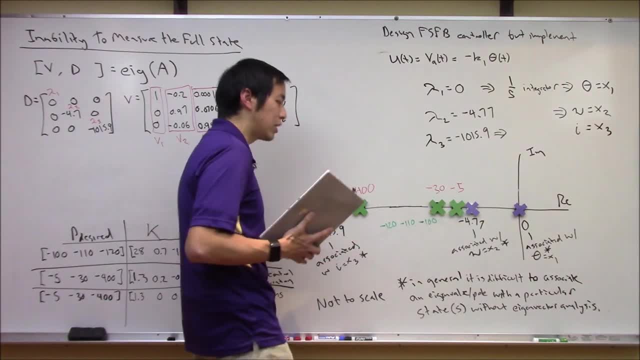 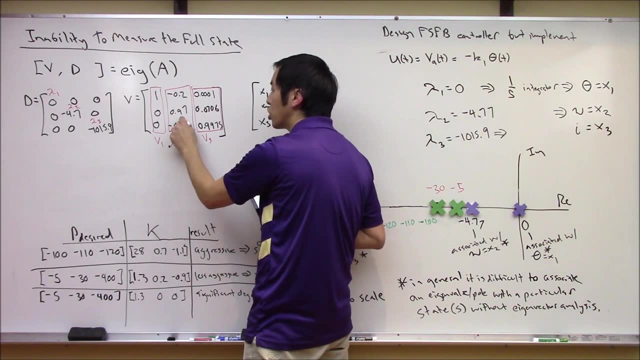 this pole right here, which we claim is mostly associated with omega. you can see that this eigenvector actually backs up that analysis here, right, Because there's this large component 0.97.. This is much bigger than these other two. 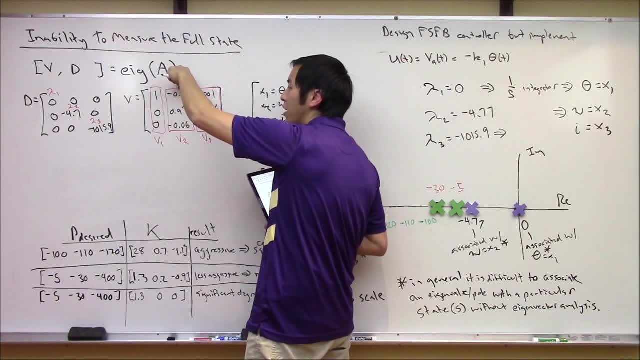 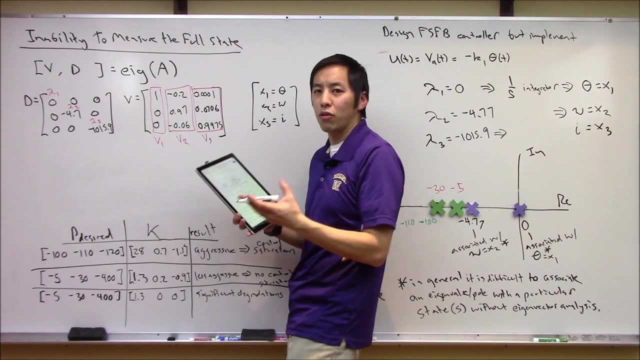 I mean, I guess this is non-trivial here, So it's a little bit coupled with the dynamics or the state here. x1 here. So this is where you see there's some of this cross-coupling, there's some of this connection. 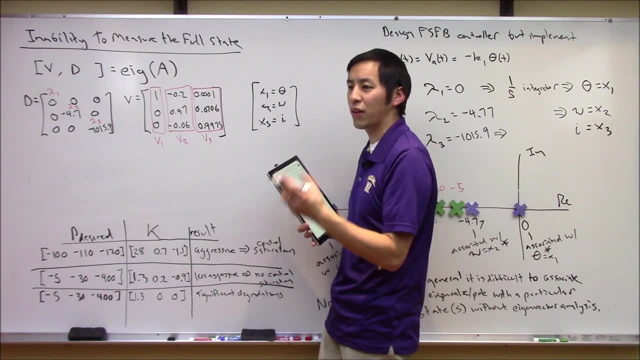 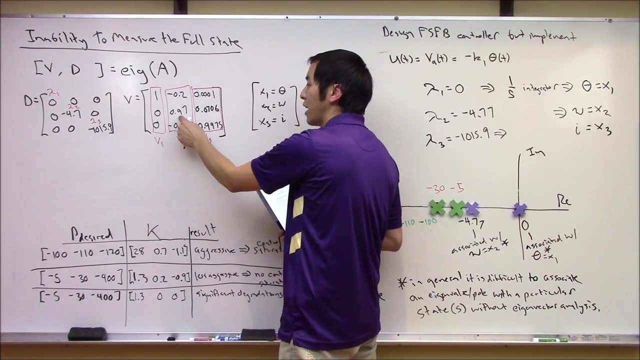 So we can't actually isolate an eigenvalue to a specific state, because there are usually these scenarios here where you've got some of this crosstalk here. But still, I think it's fair to say that eigenvalue lambda 2 here is mostly associated with state x2,. 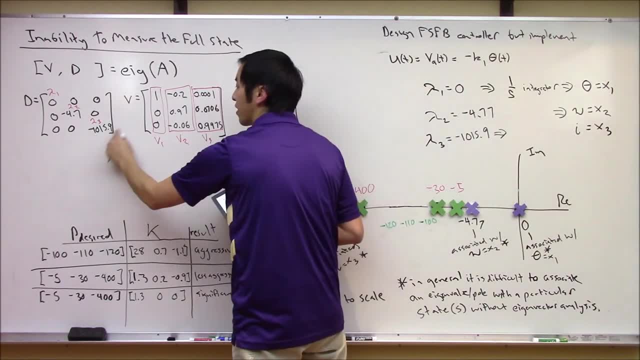 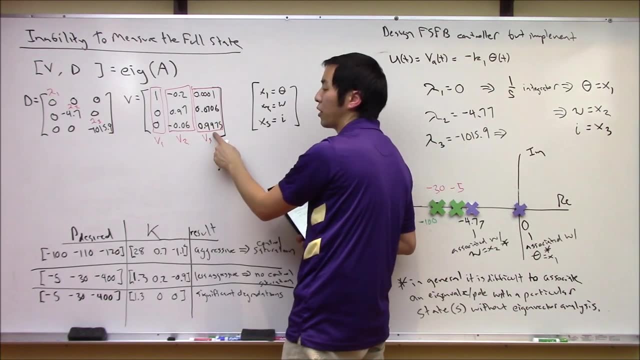 which is the velocity here. And finally this last eigenvalue here of minus 1,015.9,. we can see from its eigenvector that actually actually, yeah, this is a pretty good, solid claim here that that eigenvalue is associated. 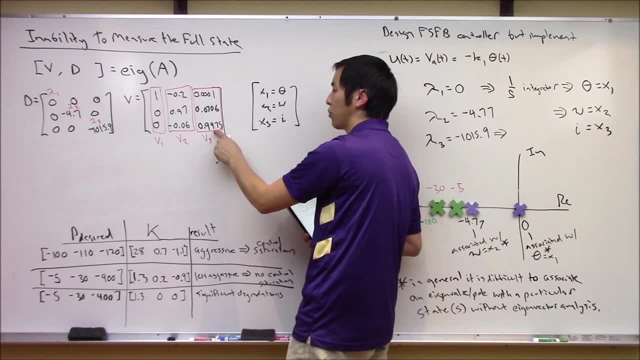 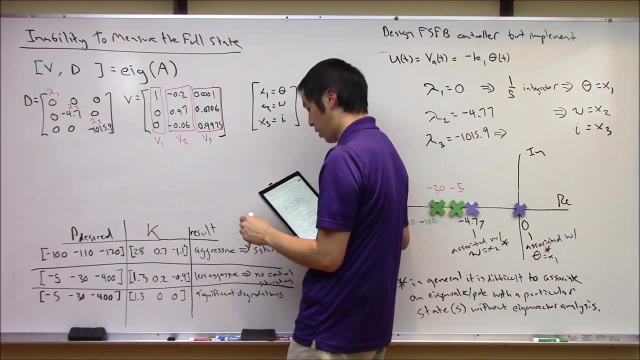 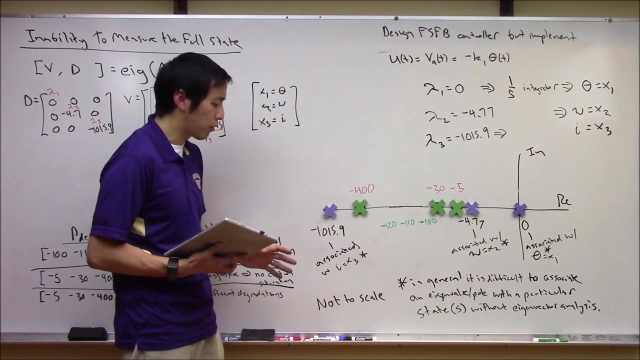 almost purely with this last state x3 here, because the third component of its eigenvector is 0.9975 here, right, And these other two are basically negligible here, right? So what we can say is: you know, these claims are roughly true here, right. 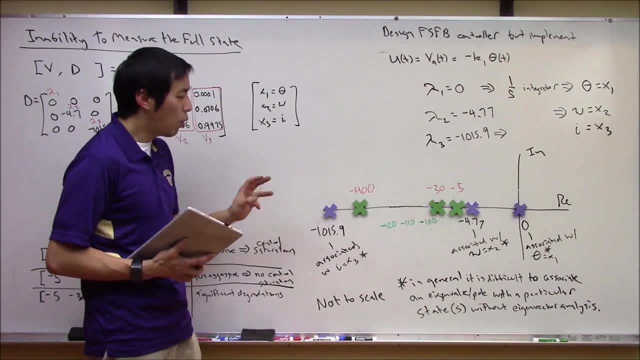 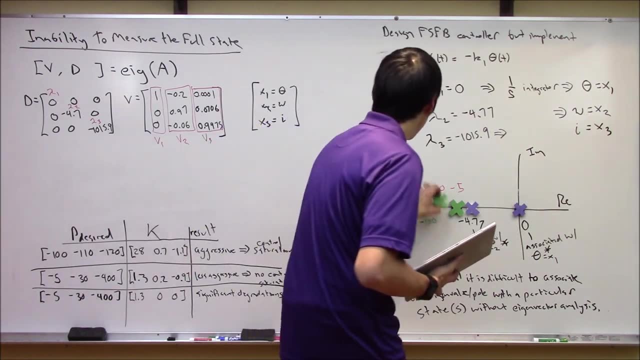 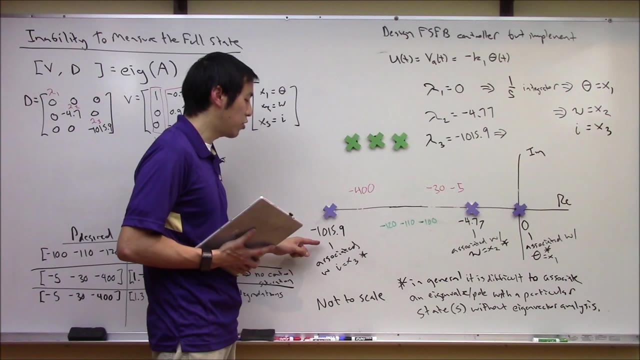 So the game plan now here is maybe what we should do when picking these desired closed-loop locations. Let's pull these off here, okay, for just a second. What we should do here is: don't screw around with the ones that you're not able to actually directly measure here. 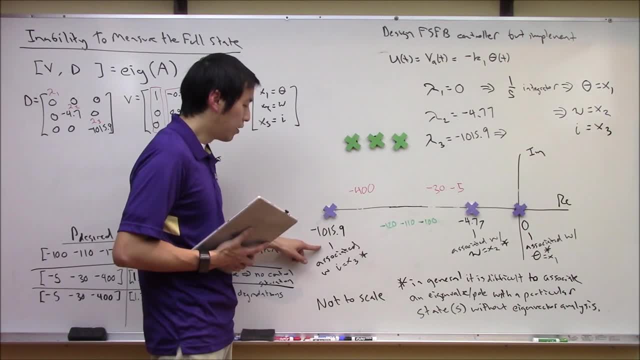 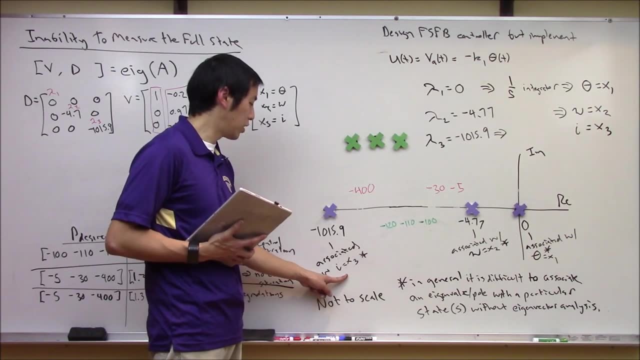 So, in other words, here this eigenvalue: since we're not able to measure the current here, don't try to change the dynamics associated with the current or this state. So in other words, leave this exactly where it's sitting here right now. 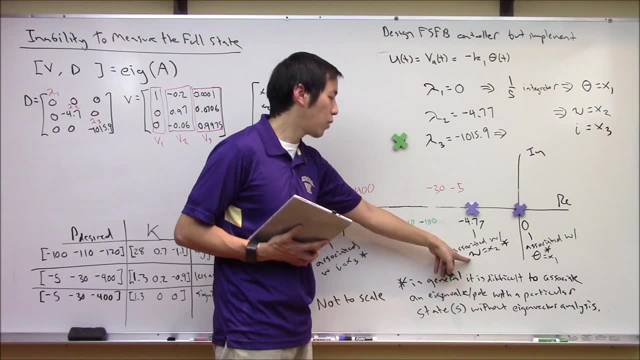 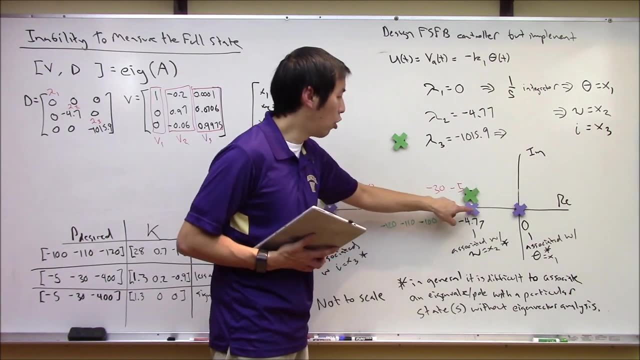 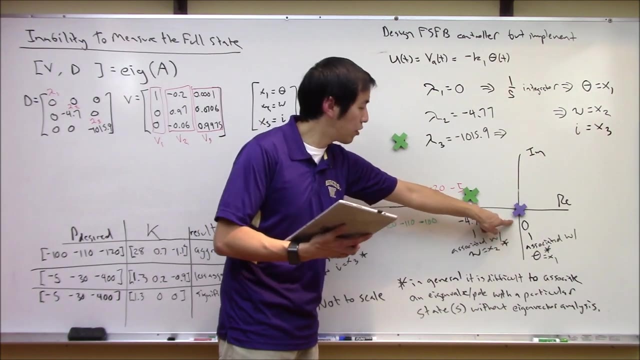 Same thing for omega. here We are not able to directly measure the velocity here, so don't mess with it here. So just leave its desired closed-loop eigenvalue should be the same as the open-loop eigenvalue here. However, we are able to measure theta directly here. 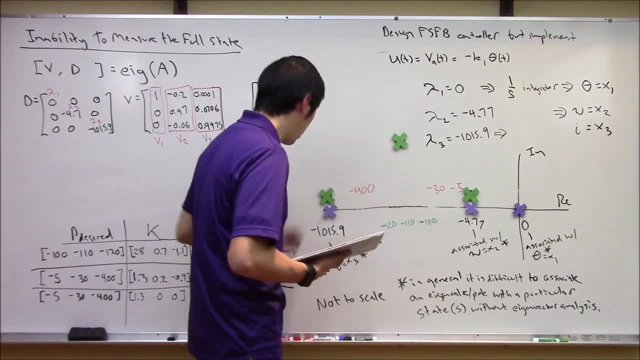 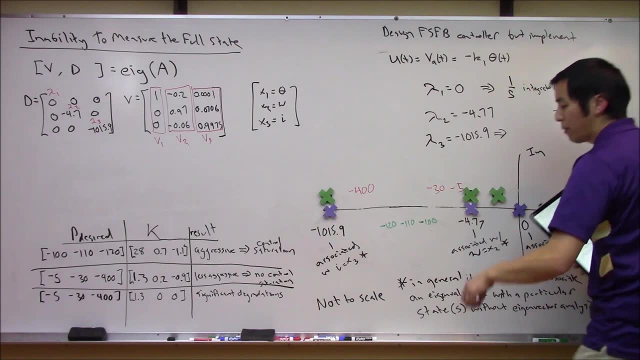 so it shouldn't be a problem to move this. So what we should do is: let's just again move it very slightly. So let's move it over here to maybe like minus 2.. So maybe in blue, let's do our last pair here. 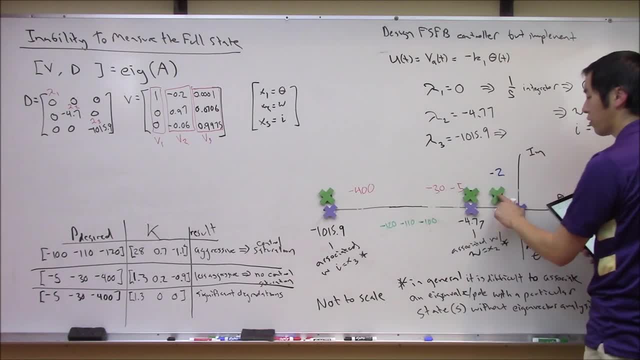 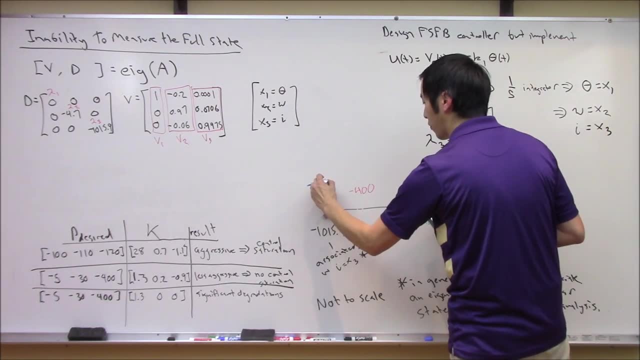 So let's go here at minus 2 here for this closed-loop one, This one here, just leave it at minus 4.77.. And this one over here: leave this at minus 1015.9.. Right, And then let's go ahead and run place on that here. 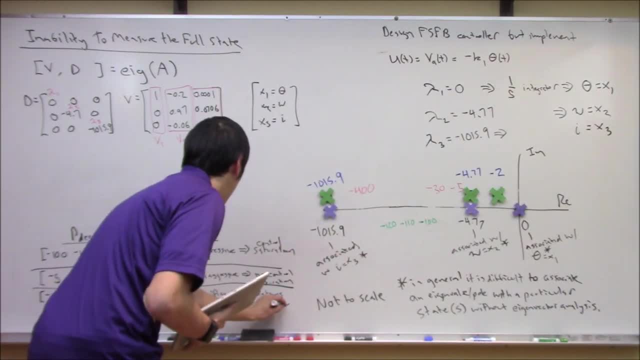 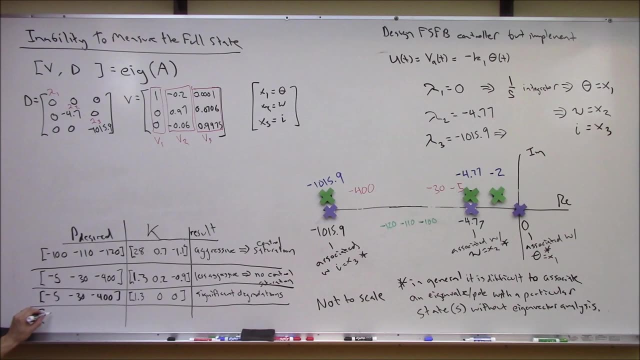 So, in other words, let's fill out this table here with one last row here, Right? So my p desired here is: we're going to move this one minus 2 here And then these other two. don't mess with them, Leave them the same here. 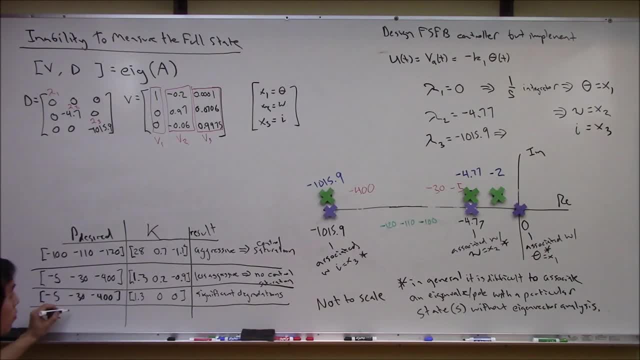 So maybe let's just say: well, what should I do? here, Don't change, Right From the open-loop position right. And also here, don't change, Okay. So let's go do that and run over to MATLAB. 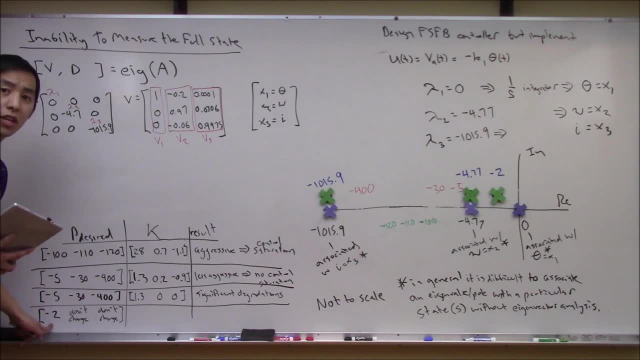 If we don't change these other two and only change the state that we're able to directly- or sorry, only change the eigenvalue that is mostly associated with the state that we can directly measure. let's do that and see what the pull placement command. 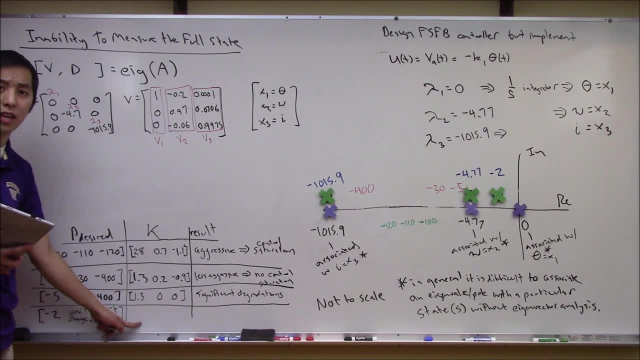 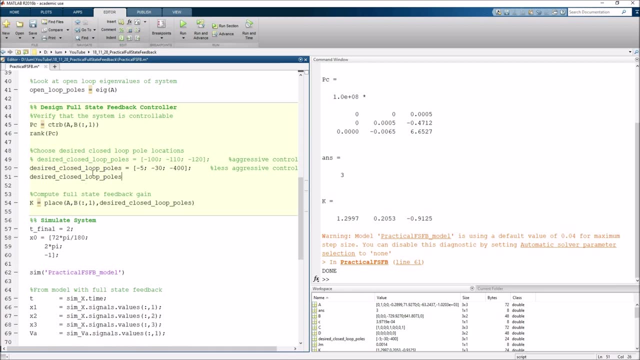 is going to give us in terms of k, And we'll look at the resulting performance here in Simulink. All right, So here we are. So all we got to do here is basically come up with a new set of desire. closed-loop pulls. 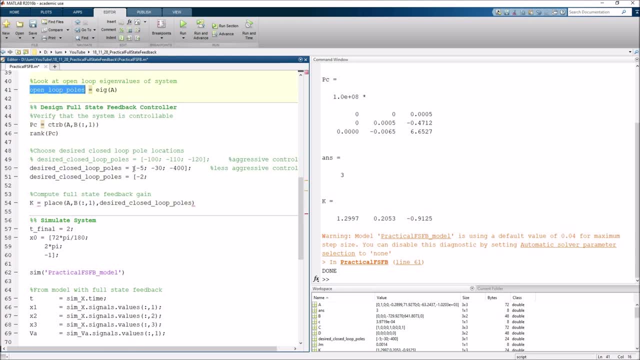 like we talked about Minus two here And then don't change the other two eigenvalues, Something like that. And maybe let's just double-check and make sure that this is in the correct order. I think it does list them in. 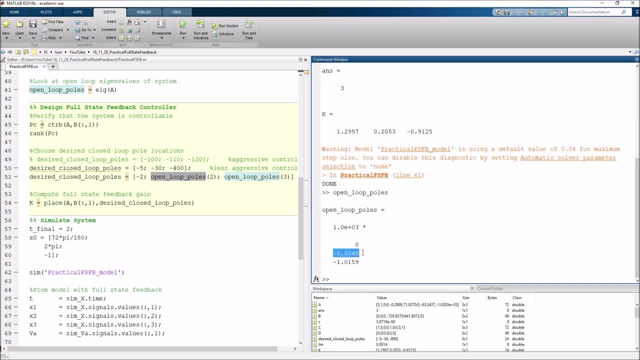 Yep, here we go. So leave this other one here at minus 4.8.. Leave the other one at minus 1,015 here And we should be good to go. Let's maybe comment out this one here And maybe let's make a small comment here. 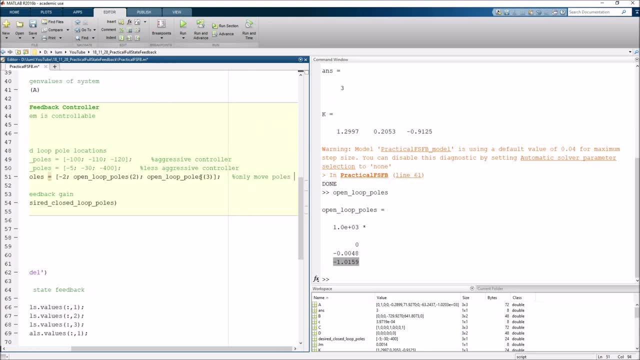 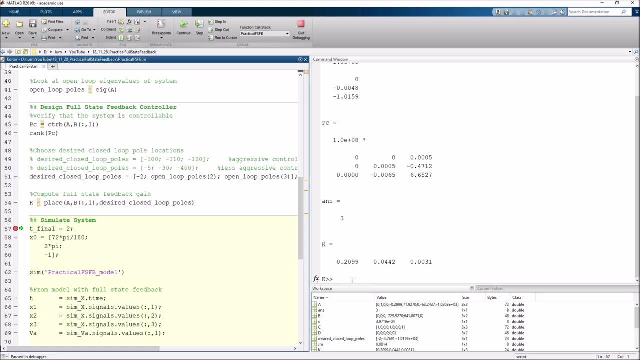 that this is only move pulls, Move pulls associated with states. we directly measure here, right, So great, Let's go ahead and maybe put a breakpoint here and run to that location, And if we do and look at the k matrix, this actually is here we go. 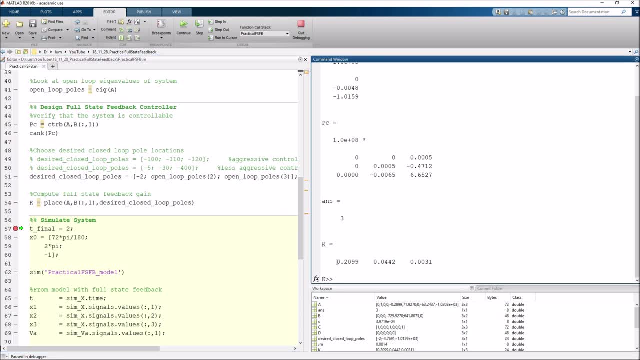 This isn't bad here, right, Look at the controller we end up with here. We end up with a 0.21 here for the first value, But the second- k2 and k3, their magnitudes are, you know. 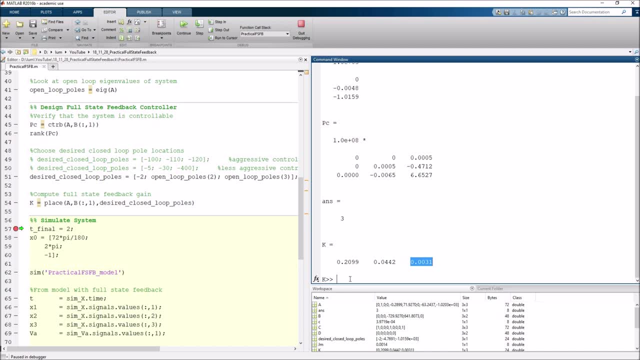 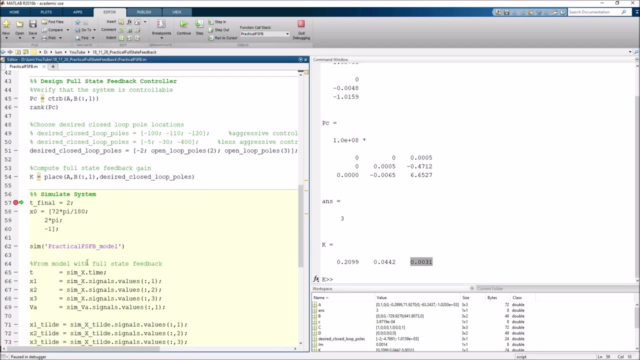 relatively small when compared to the other one. So hopefully it's not a big problem to neglect them when we run our simulation. So again, what we'll do here is run this model here. So just to refresh your memory, I'll open the model here. 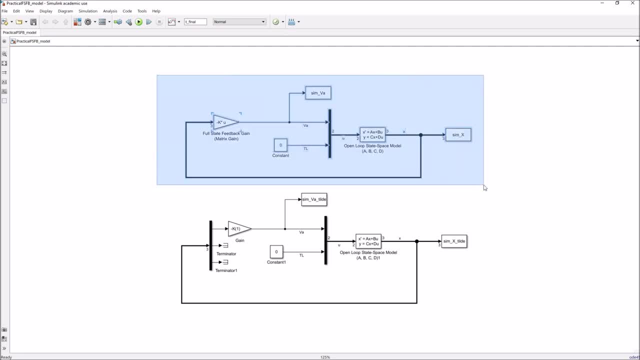 This is actually the exact same situation we had earlier. The top is the full on system. if you actually were able to have all full state feedback control. And then this bottom one is the realistic scenario where we're only using the position of the motor for feedback here. right? 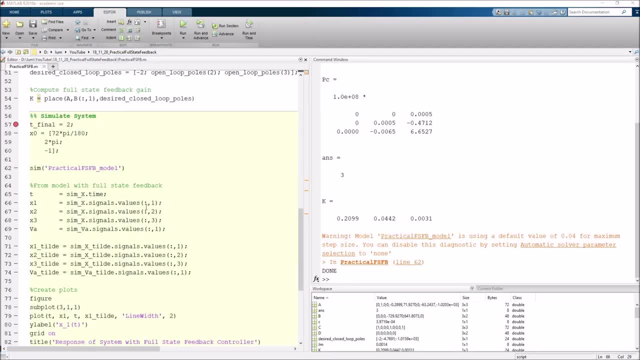 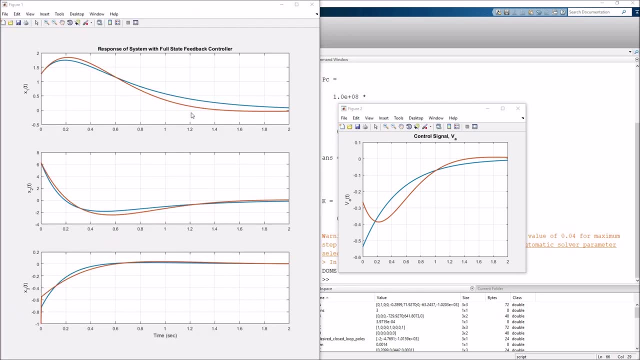 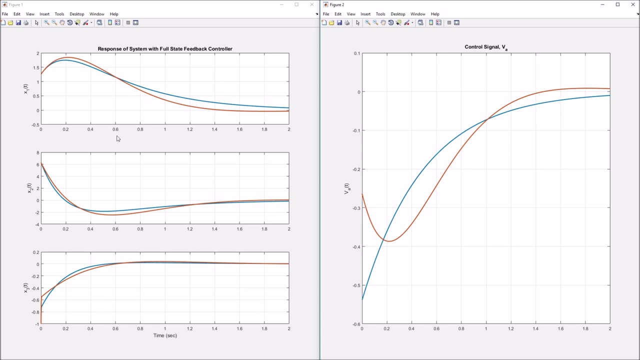 So let's go ahead and run this whole thing, And I'll pull up the result and the control signal here. So again, let's put them side by side here, And here we go. This isn't bad here, right? So again, there obviously is still a difference. 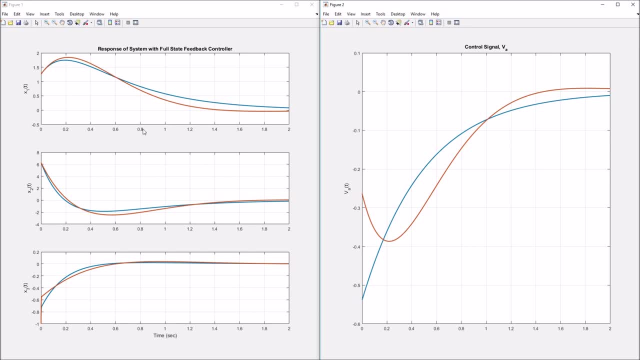 between the blue and the red line, but they're not as drastically different as we saw earlier right. So we're not as surprised when we design and hope for the blue line, but we actually get the red line here, right, So great. 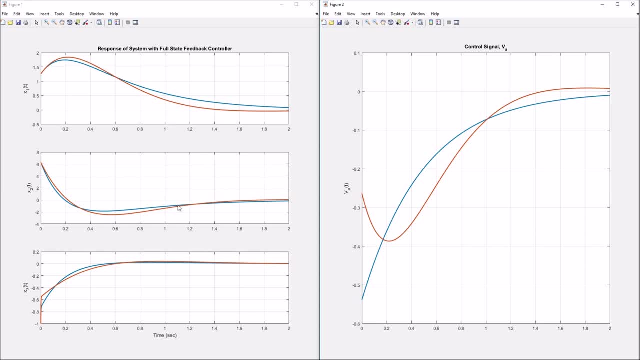 This looks pretty good here and it looks like a reasonable way to go about trying to solve this implementation issue, where, in reality, it's difficult to measure the full state of the entire system. All right, great, So that was pretty reasonable. So why don't we finish our table here? 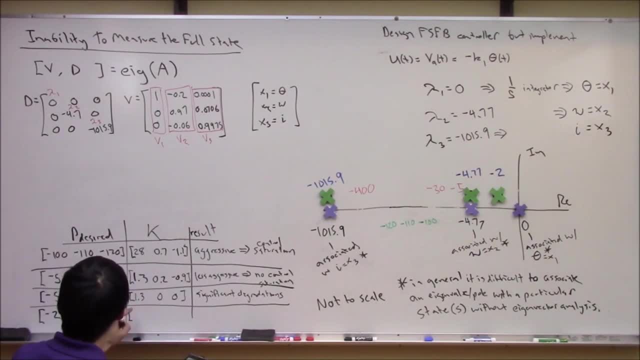 just to make this summary slide complete here. So in this situation we ended up with a controller here, okay- of 0.21-ish here, And then 0.04, and then about a 0.003 here, right? 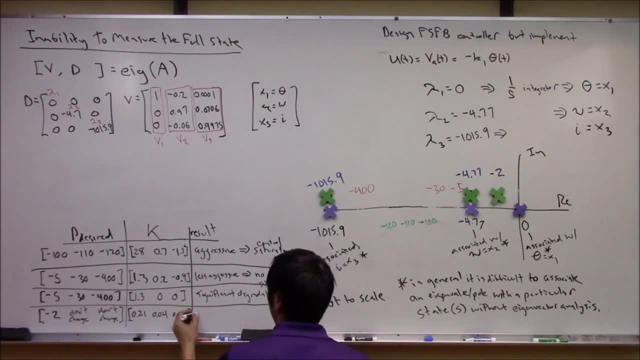 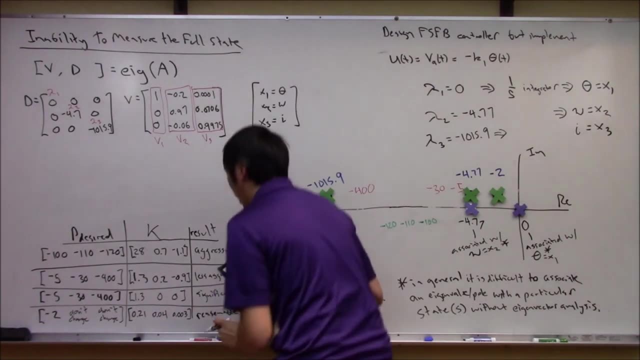 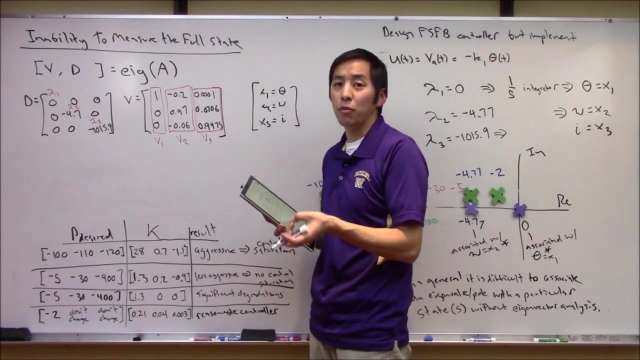 And again, what actually resulted here was: this was a reasonable controller right. It wasn't super aggressive here and it didn't require us to use states which we're not able to directly measure here. So I think this is probably the best we can get. 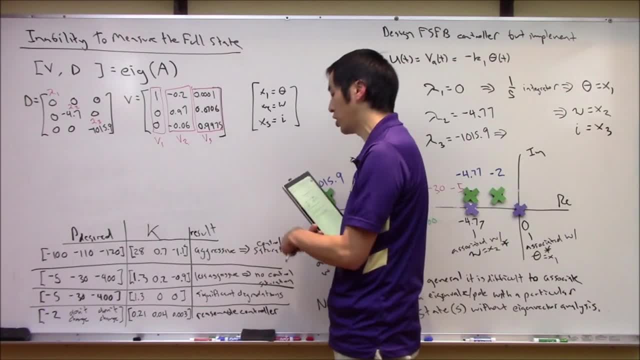 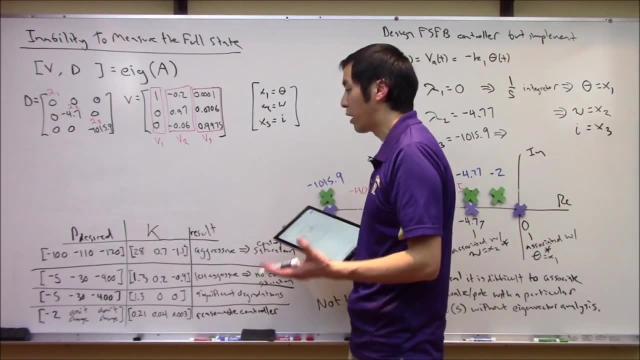 It's the most realistic. It deals with control saturation issues. It deals with this inability to measure the full state of the system And I think it's a reasonable way to go about trying to implement a full state feedback controller with an actual, real system here. 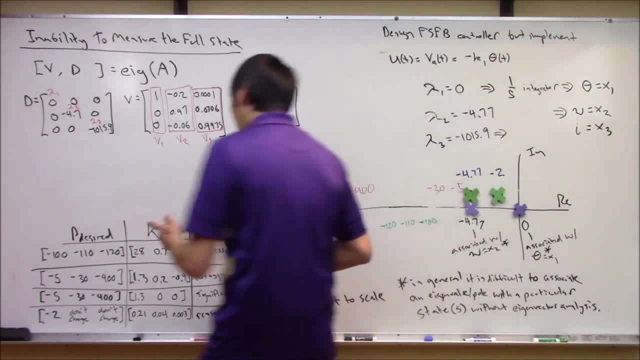 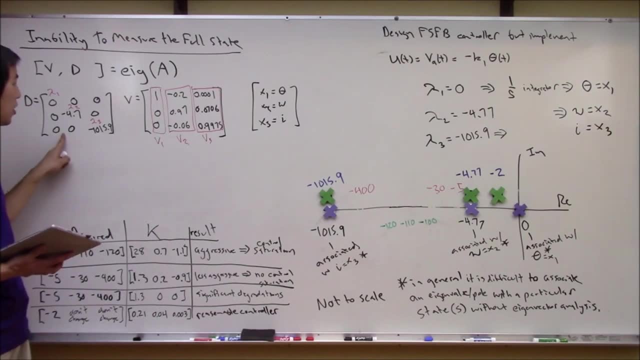 So, with that being said here, let's talk real quickly about this concept here of choosing the eigenvalues and then, kind of in a circuitous fashion, hoping that it resulted in a full state feedback controller that was actually implementable. Hopefully, when you're watching this, 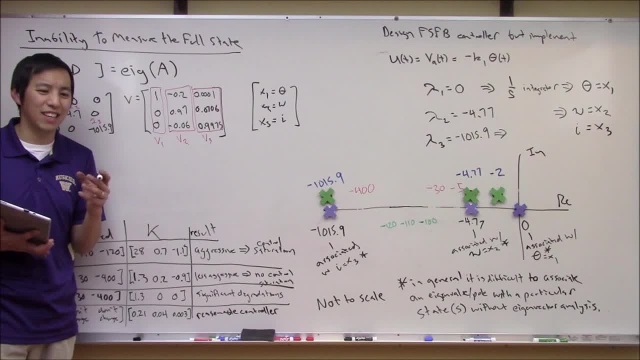 something probably went twang and clang in your head and you said it was a little bit unsatisfactory here, right, It seemed like a very roundabout way, indirect way, of trying to design a controller here by moving these poles where we don't actually have.